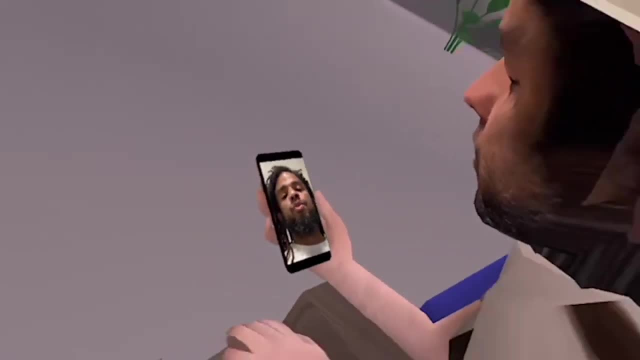 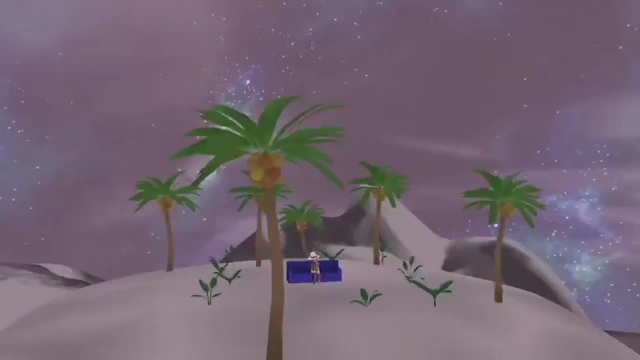 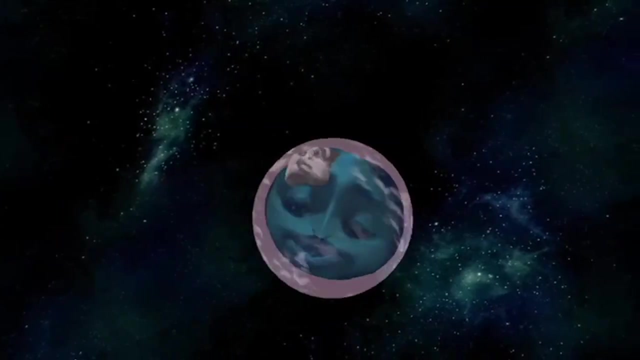 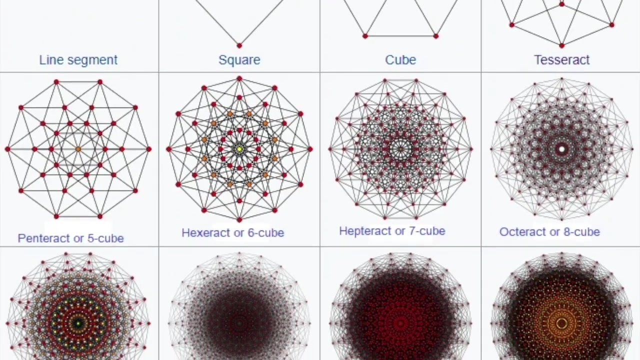 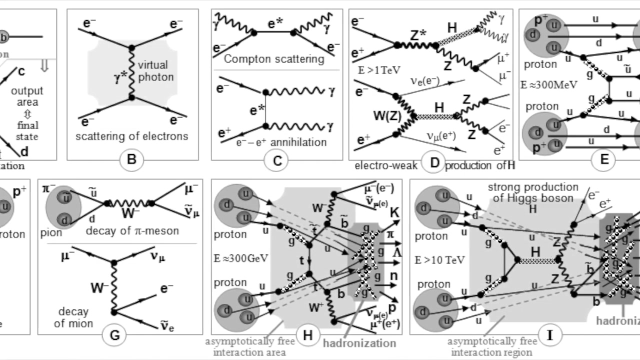 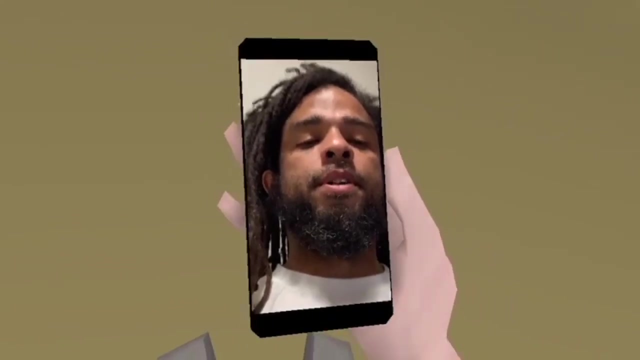 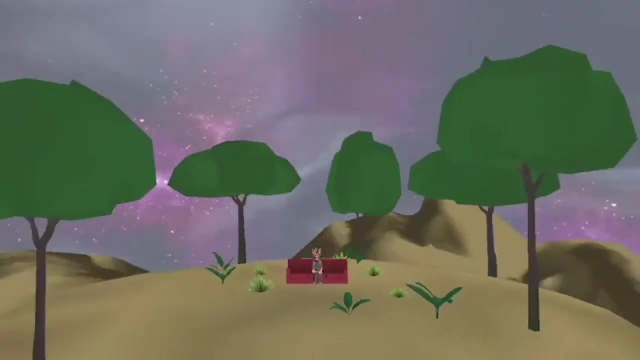 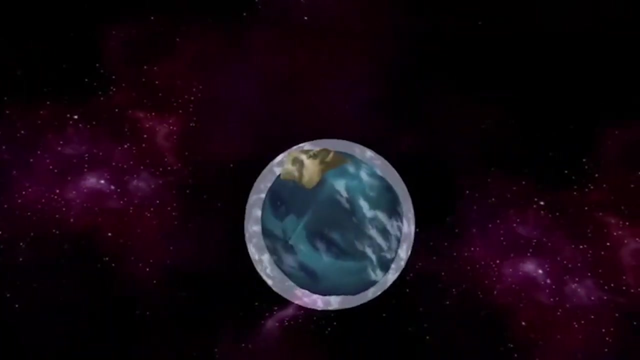 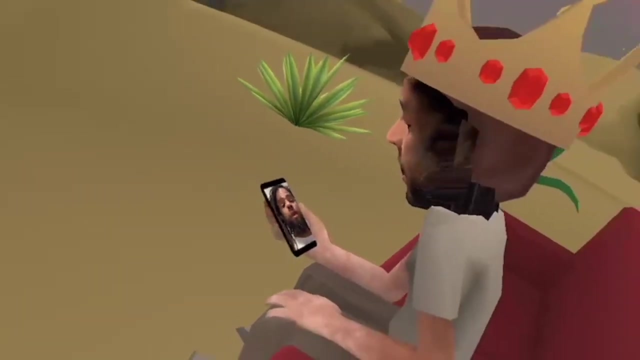 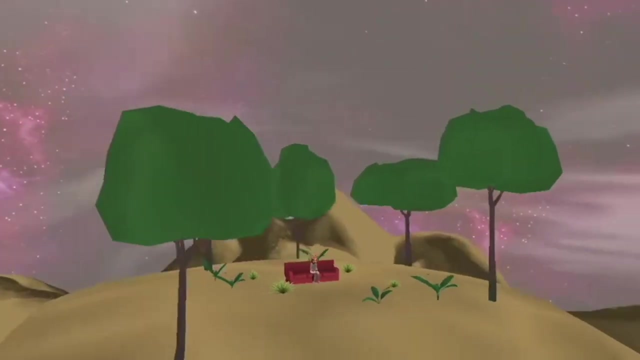 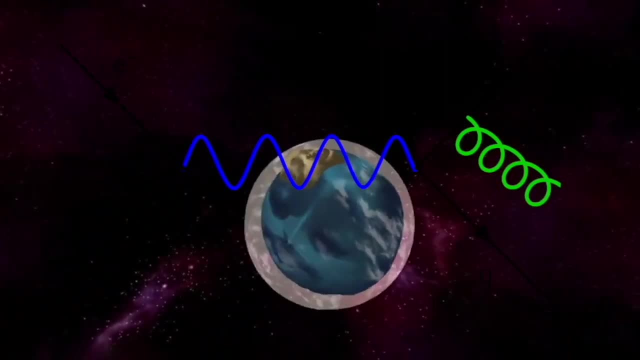 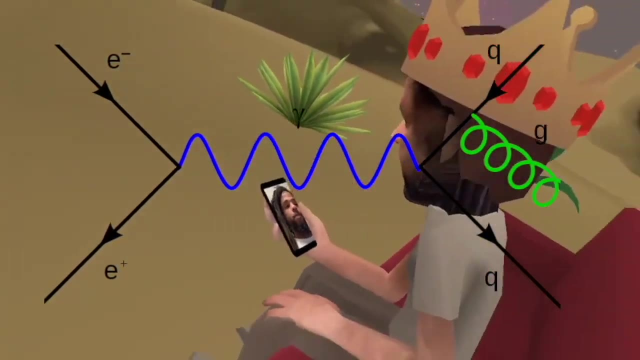 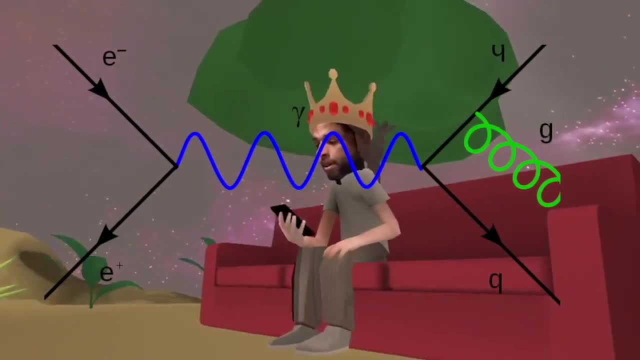 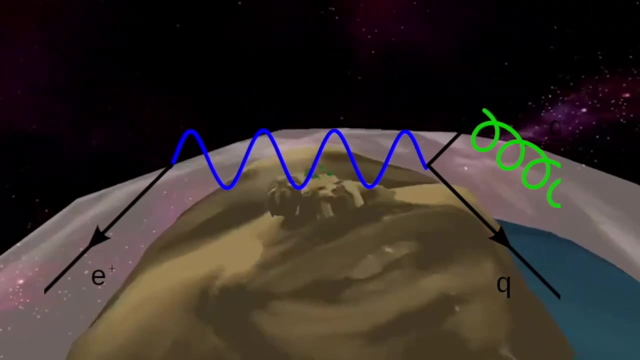 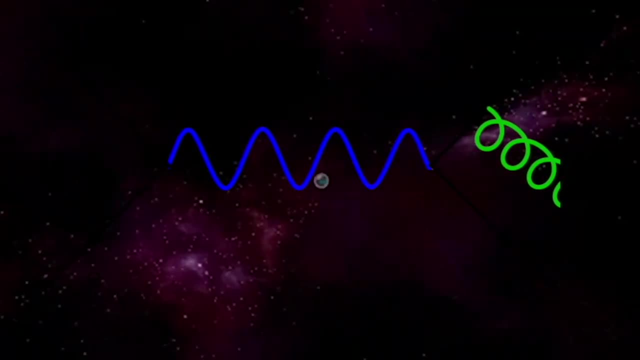 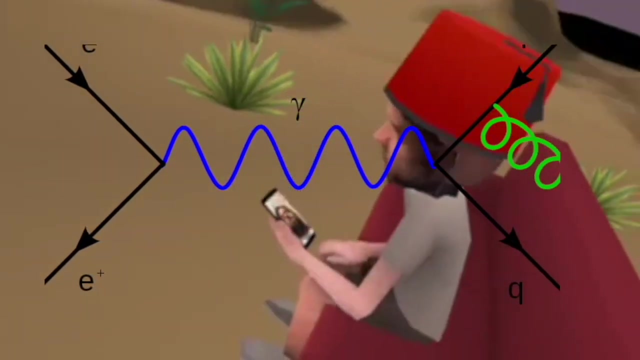 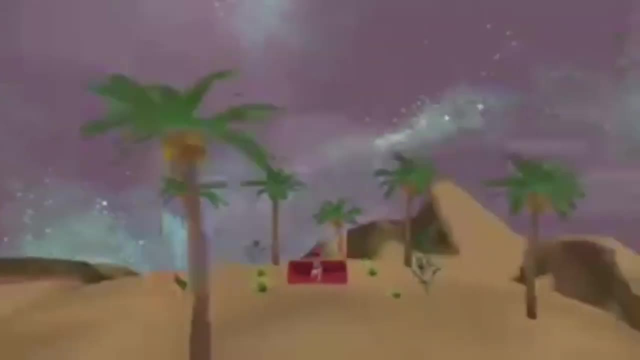 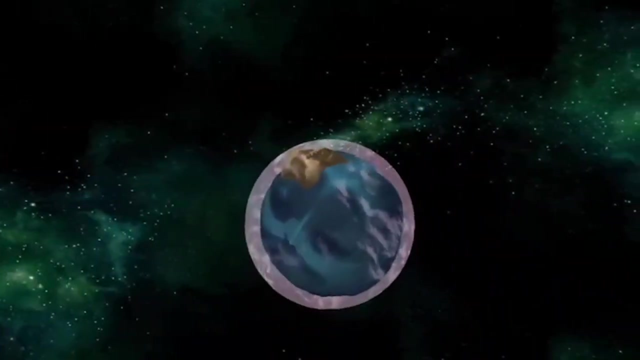 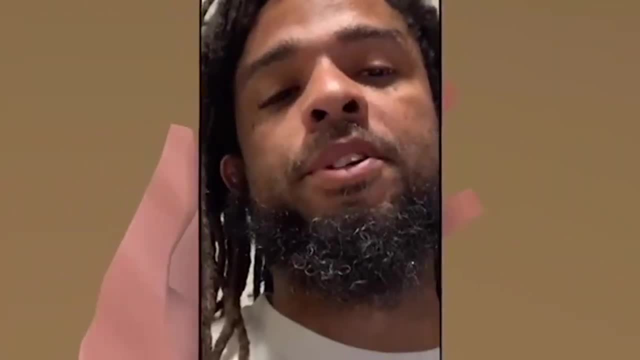 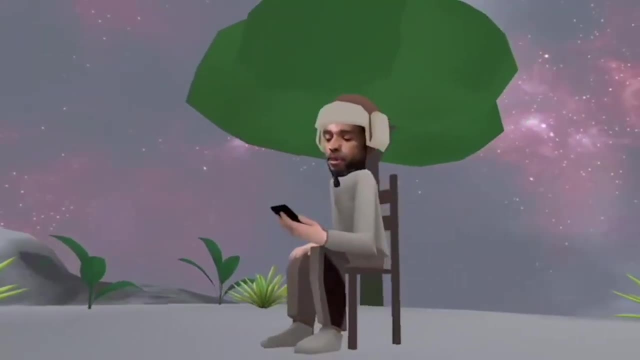 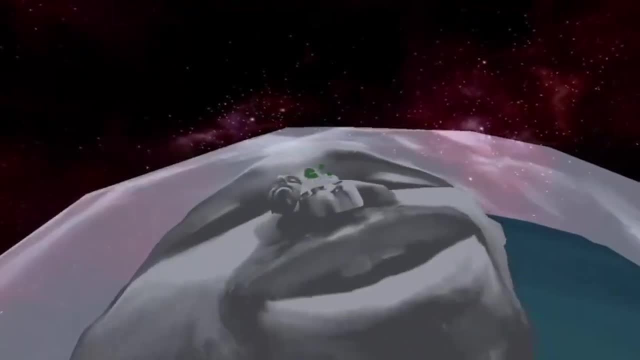 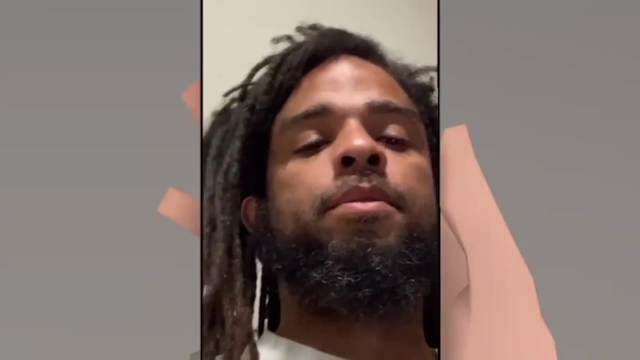 but then, if you do like, take a time-lapse photo, like when you see cars driving through the city. you see the lights as strings. your life looks more like a worm, like you're going to work, you're going to the grocery store, you're going to these places. it's more of like a trail of your body, you know. 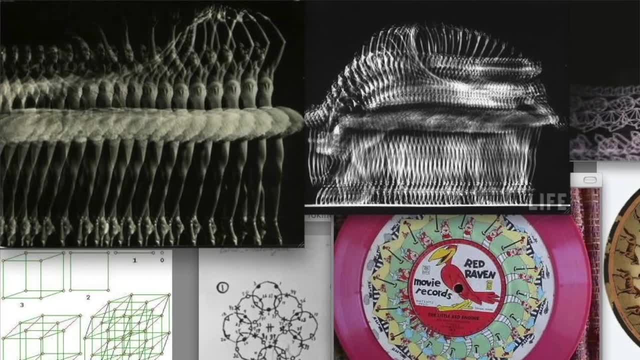 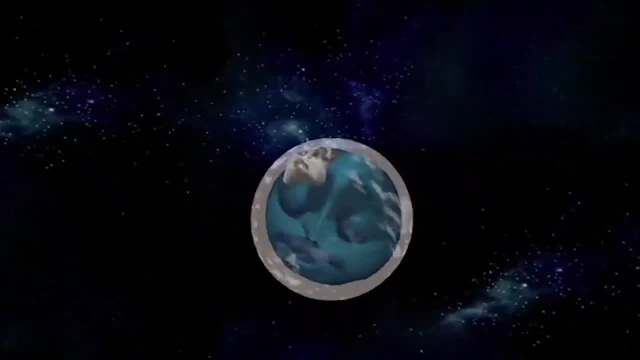 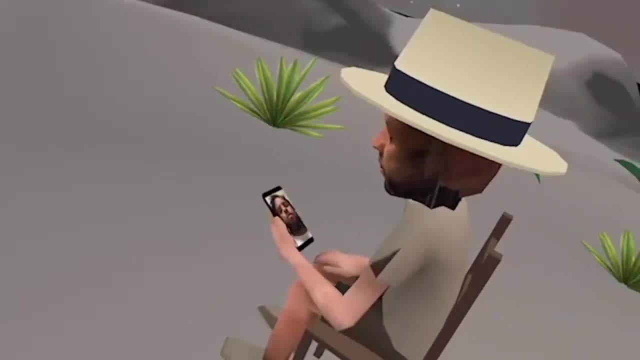 and i first learned about the fourth dimension, uh, under, uh, steve sagur at the paideia school when i was in high school in atlanta, and uh, you know, rest in peace, steve sagur. and you know he was working with people at brown university and, um, i guess he went to brown university, but yeah, 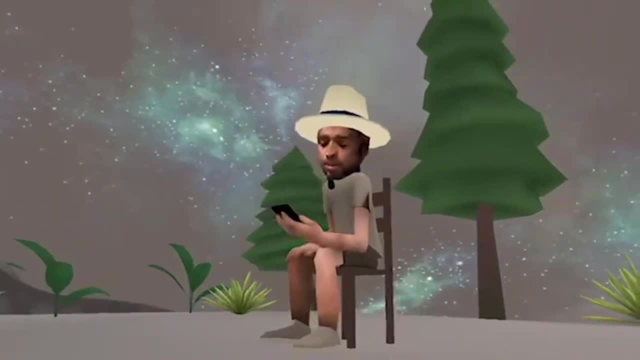 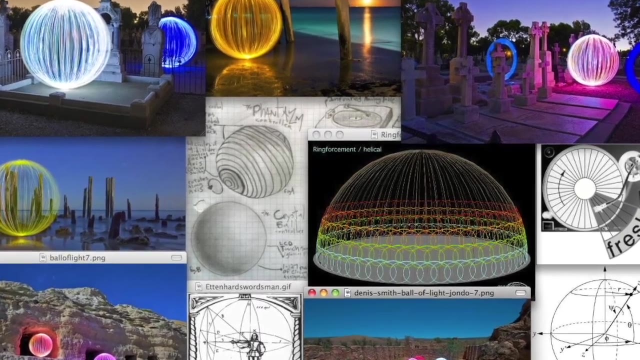 he was working a lot of students in the 90s and so in high school he was telling us about the fourth dimension. you know we were just kind of bugged out like oh, wow, like it's, you know. but really the fourth dimension is not very, uh, difficult to understand, you know. um uh, because 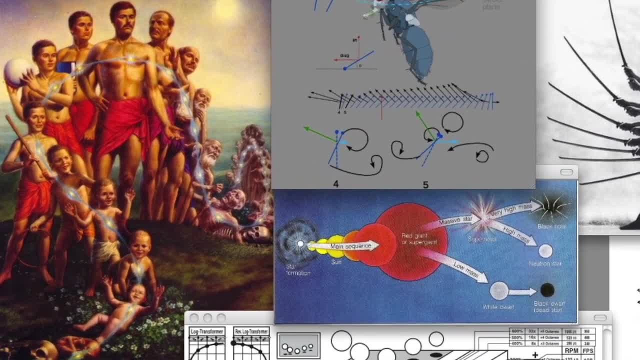 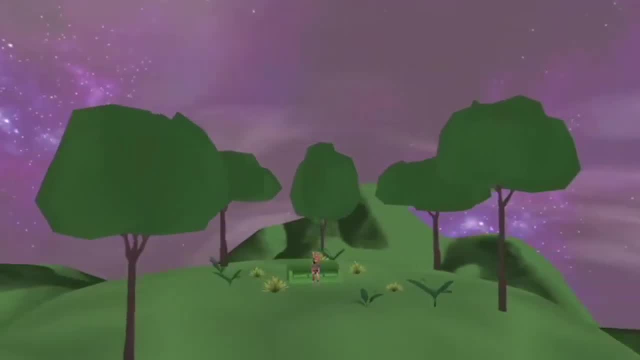 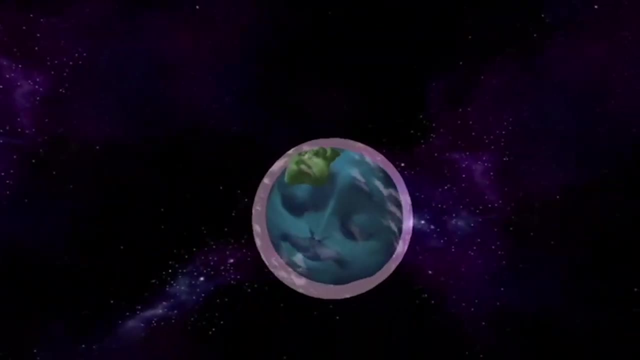 really it's just time relative to our 3d world. so every higher dimension up, you know it, uh, the fifth dimension is just is time relative to people in the fourth dimension. but people that are living in a fourth dimensional plane and not just a 3d plane, they, uh, you know, they're looking at the world in a time-lapse view and 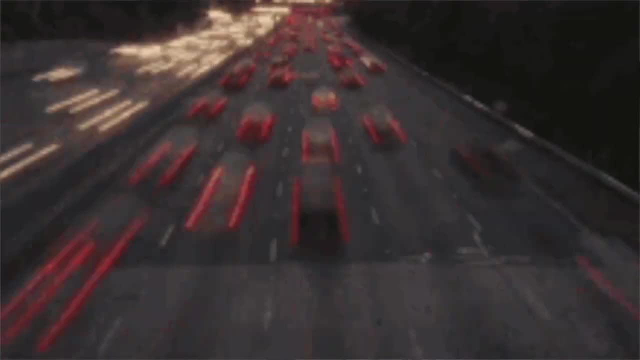 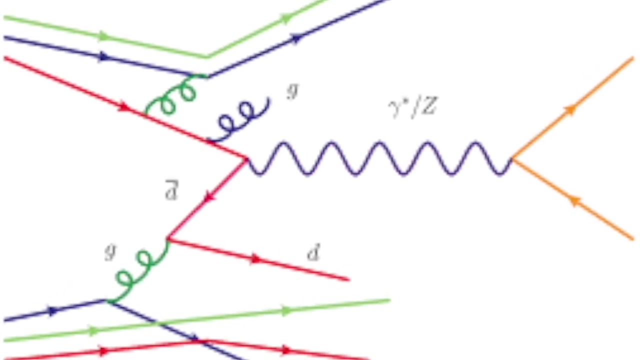 that's similar to what feyman diagrams are. feyman diagrams are stepping outside of normal time and showing a bigger picture of kind of like a almost like a predestination type of a thing where a bunch of particle events happening. it looks like a star chart. you know, i'll show the graphs. 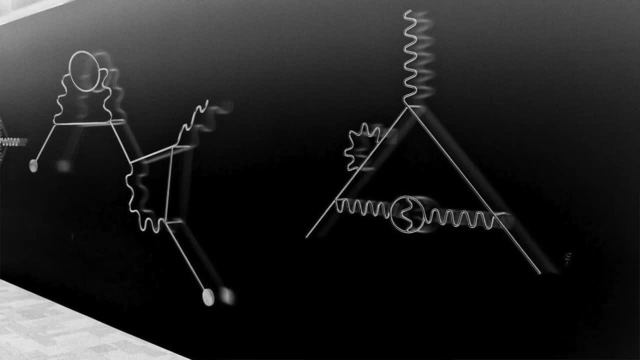 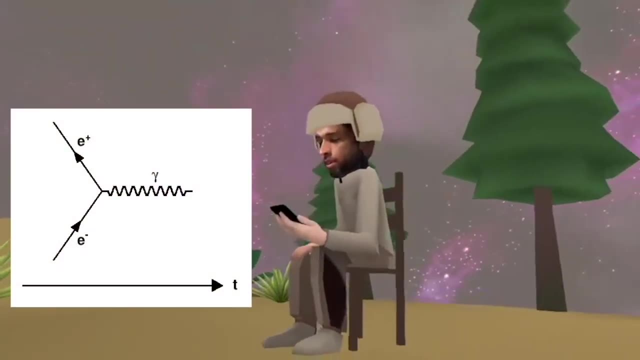 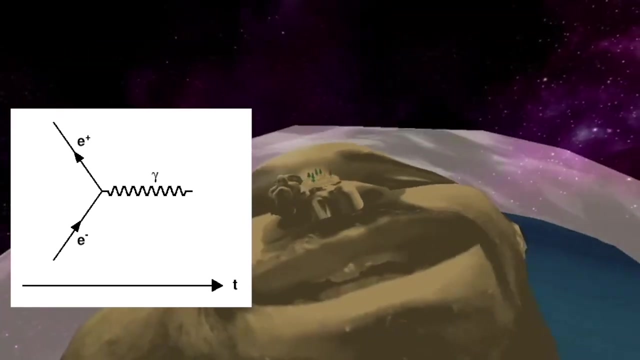 uh, or these diagrams, um, they look like star charts, you know, because you see these particles hitting each other and forming new particles. so the two rays come together, right, the positron and the electron. um, they both hit each other and they annihilate each other and they create a photon. 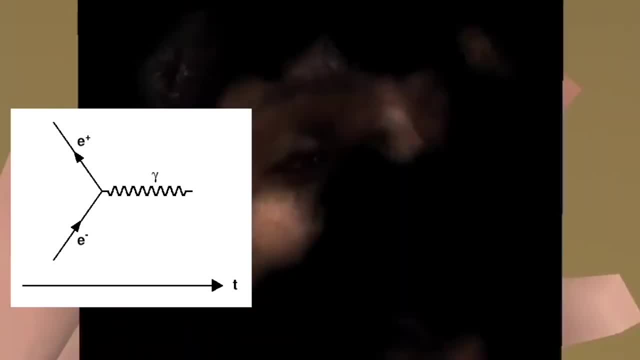 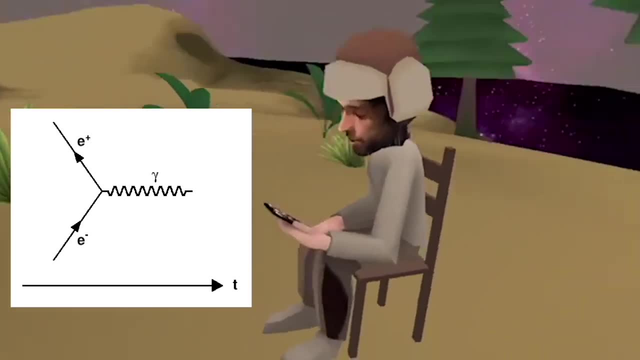 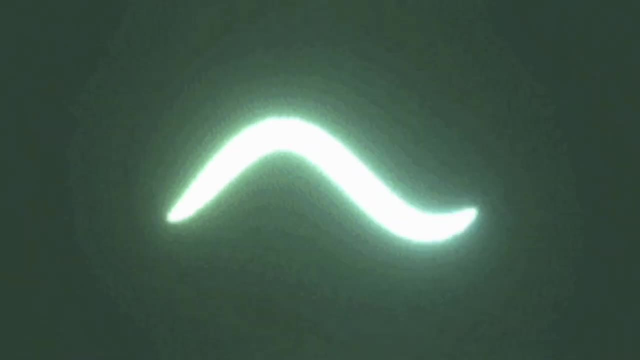 and the photon is represented by the gamma symbol in greek, but the actual visual image that feyman used in his diagrams is pretty much the ancient egyptian uh dj symbol, the j right like tahuti jahudi, uh the snake, you know the the winding snake, the wavy snake. 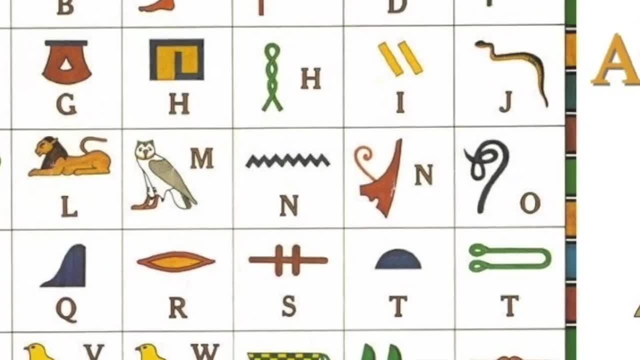 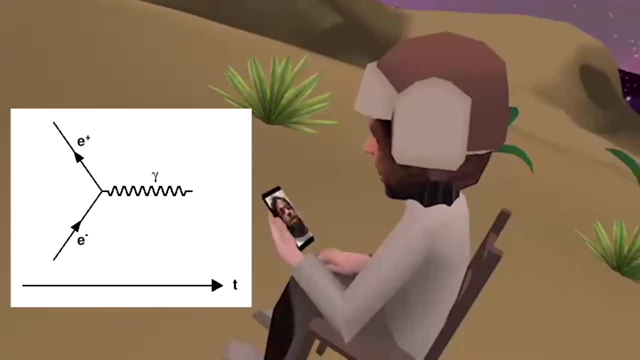 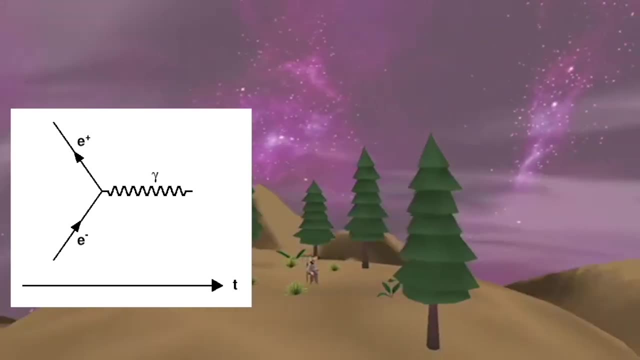 and the symbol in egyptian right, um, and that's the photon symbol. so the two rays, the forward ray and the backward ray of the electrons, are hitting the actual uh, you know the wavy pattern, the, and they become a photon. you know so the um, it looks like all three of them are hitting. 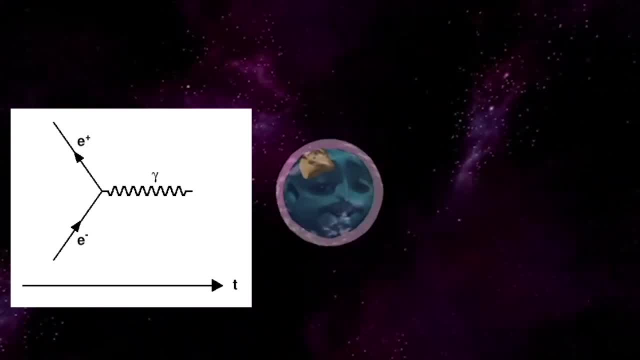 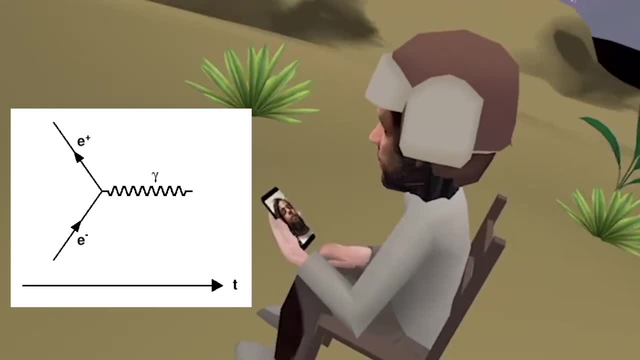 at the same time. but they're not. what's happening is the uh negative electron and the positive electron, the positron. um, you know, electrons are by nature negative. negative they're, they're hitting each other and they're annihilating each other and they're becoming a photon, right? so that's. 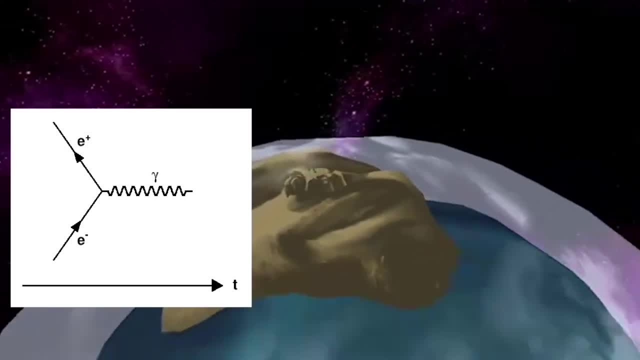 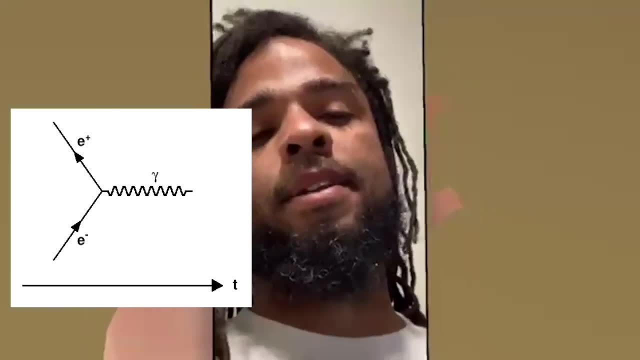 what's happening in this picture, so that so the photon is then traveling right at the speed of light. and remember, um, electrons aren't traveling in a linear path. you know, electrons can, you know, pop in and out of existence. like i was saying, 10 of the electrons in our bodies can be anywhere in. 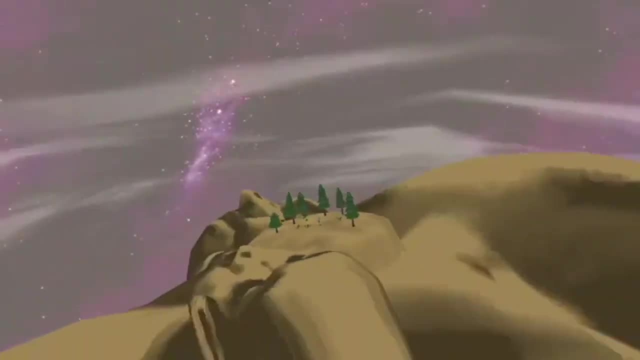 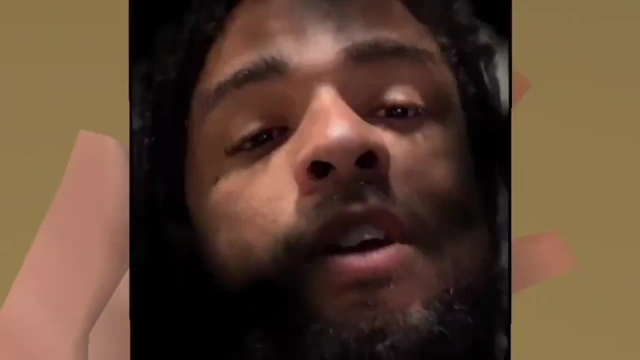 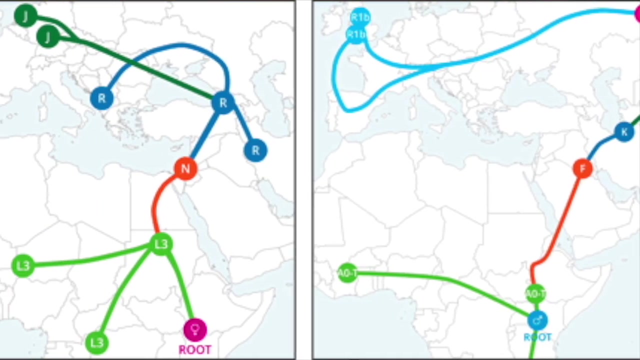 the universe. the other 90 are within our body, right? so you know as far as, uh, you know that type of stuff, that means that you know um quantum entanglement wise we can be. you know um a lot of different places and that goes back to the ancestors. if you take everything on a fourth, 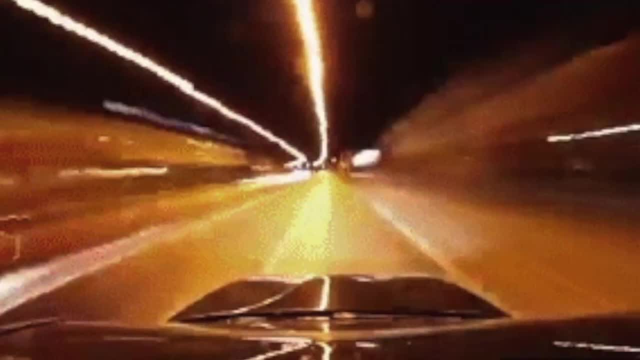 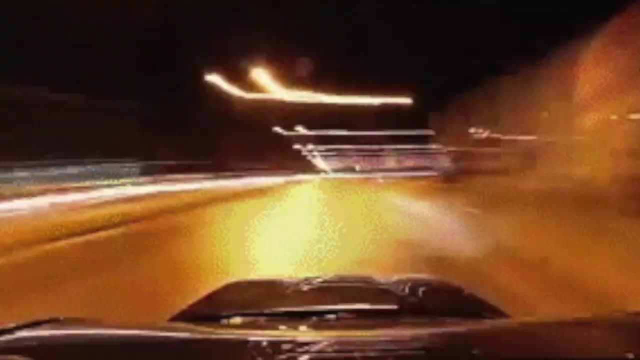 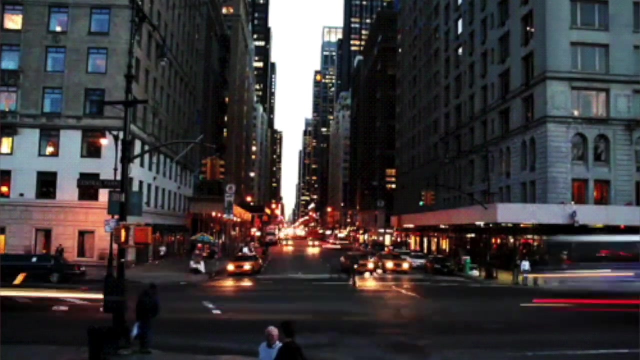 dimensional level. if you um go to the car that's driving through new york city really fast and you see the trail of this light, that 4d light, if you take that car and and you revert and you take um go all the way back to where it was made at the factory right, the whole worm-like trail of that car's existence. you know. 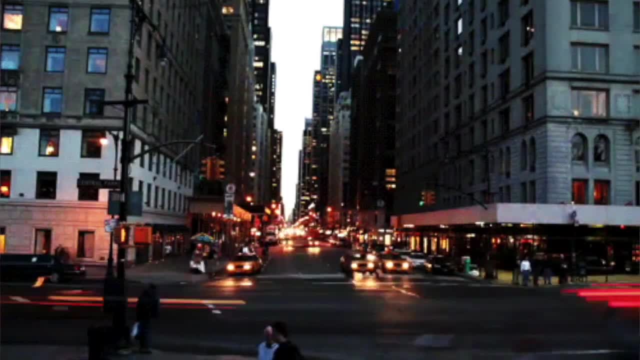 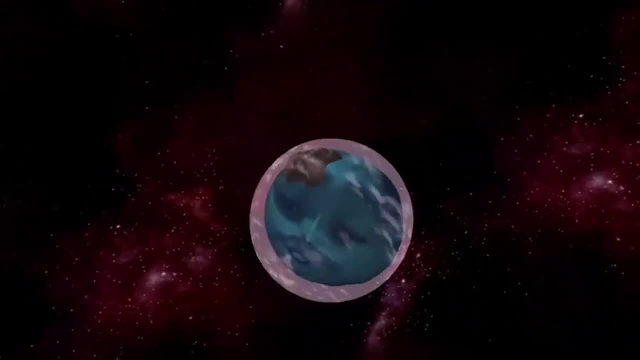 you're going to see, uh, where that car originated from, and you'd be able to see that, you know. so, from a fifth dimensional world. they'd be able to look at the fourth dimensional world, like how we see the fire, uh, you know, push the car down the whole way right, and not even be able to see. 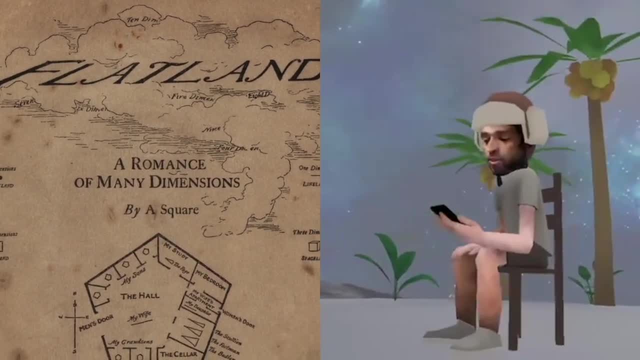 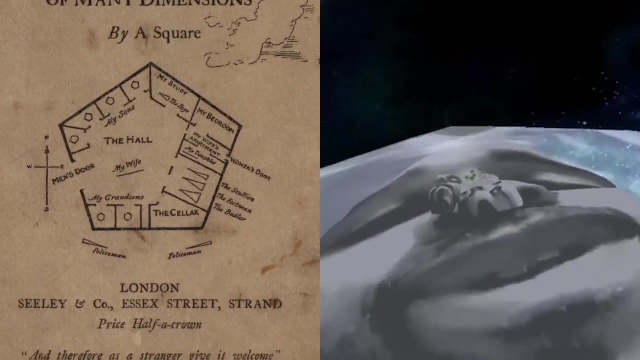 where we are at the edge of the earth, right so that with with the five dimensions and encourage an in person experience. that's truly the most powerful way people in higher dimensions look at a no taking links where you know. you know you're just sitting around on a bike riding a. 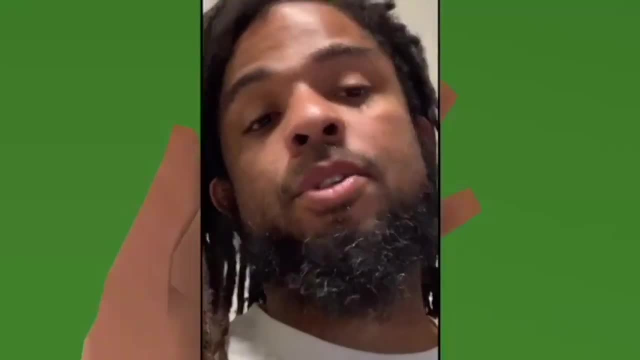 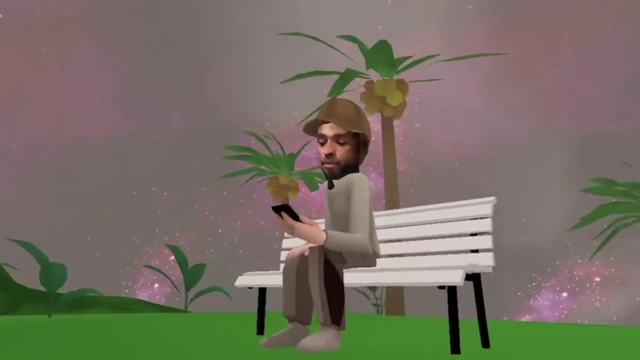 bike, riding a bike, spinning a- well, you know, just be like: oh yeah, i can see, i can see trees, just like that. right, let's look at a space inRISE, because that's where you know life is. you know, like it's not an object, you see, it's just a thing, that's not something. 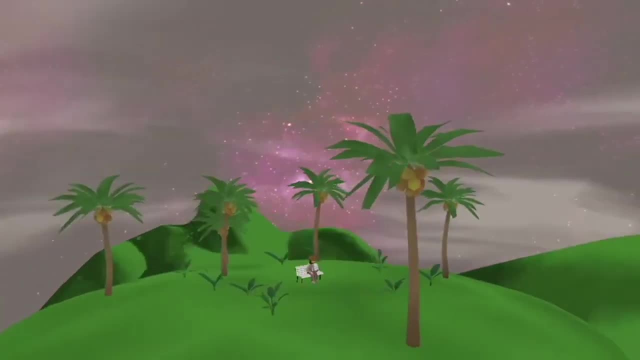 and dimensions. might they see that the lower dimensions is objects, just like we see? uh, you mouse's world? he's living in a flat world, you know? that's that's his whole world- is on a plane, right? so you know there's a book called flatlanders you might want to check out. 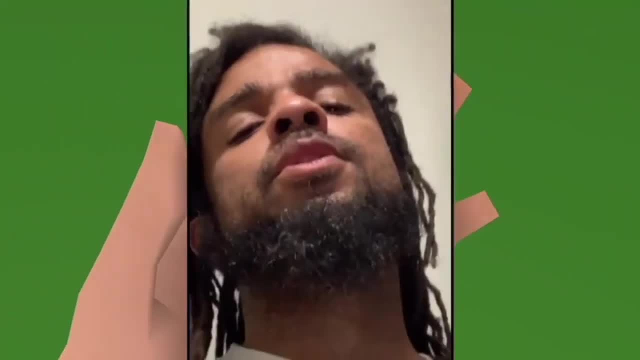 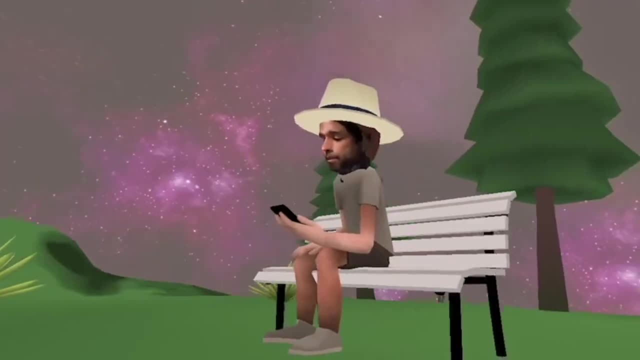 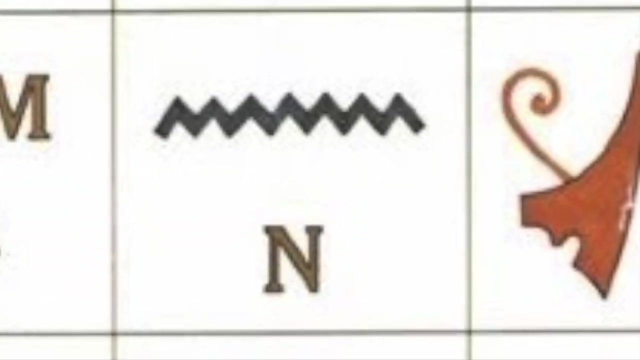 um, and i believe maybe steve sagur actually showed us that in high school flatlanders, you know, and uh, yeah, so you know. um, with the feyman diagrams you'll see that the photon is traveling right. it looks just like, exactly like the, the symbol in egyptian right um. 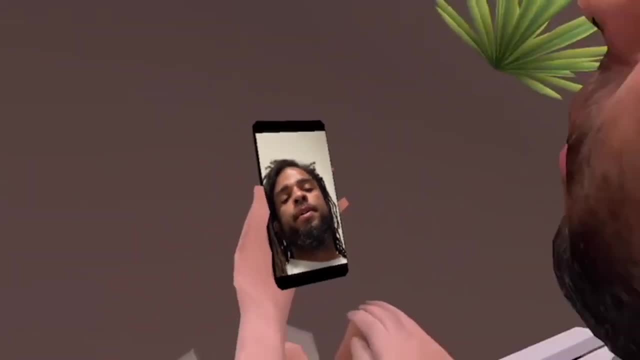 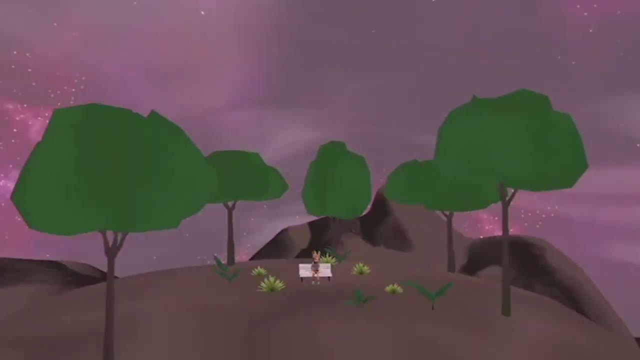 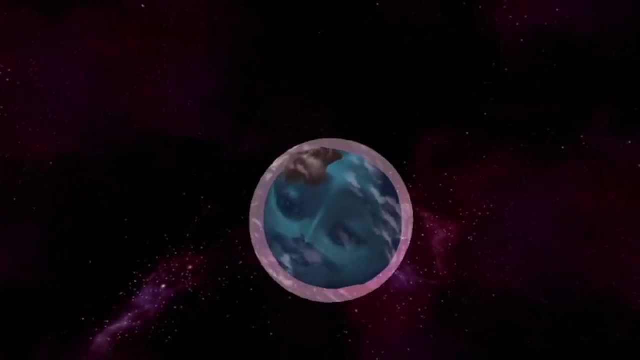 and also it's important to note too, uh, that although the, uh, the egyptian glyphs have been said to be- uh, you know, rosetta, stone, stuff is said to be deciphered and all that type of stuff, given that it was germans that did all that stuff, we don't know if all those phonetics are. 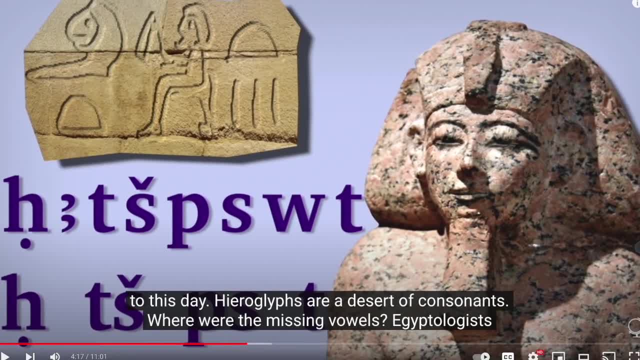 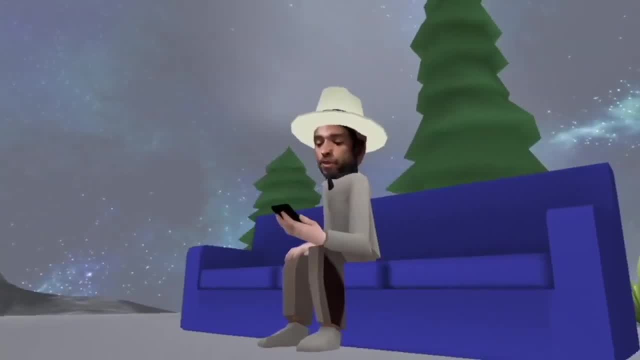 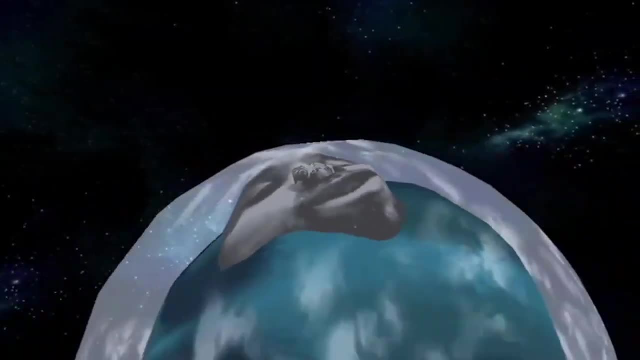 actually correct, you know, because there's no vowels in in all these things and a lot of these things were created from a germanic uh perspective and, uh, you know. so the people say the meta netter news, the meta netter's been uh deciphered, but you know as far as how it's. 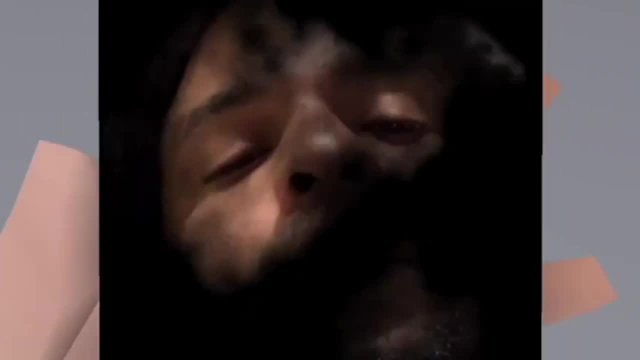 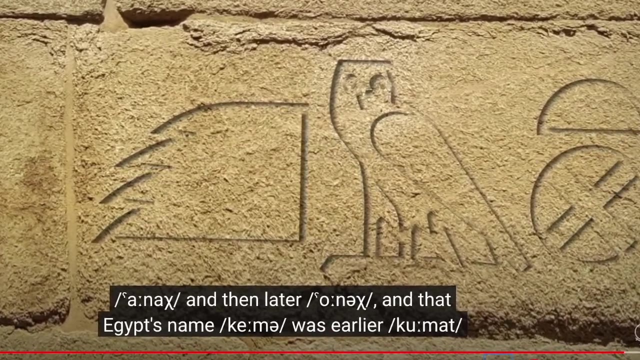 even said and things like that. you know we don't really necessarily know. a lot of people say: you know the the first name of egypt was kuma. right, you know um the way it was pronounced, but you know there's so many different pronunciations, especially as far as the vowels, we don't know. 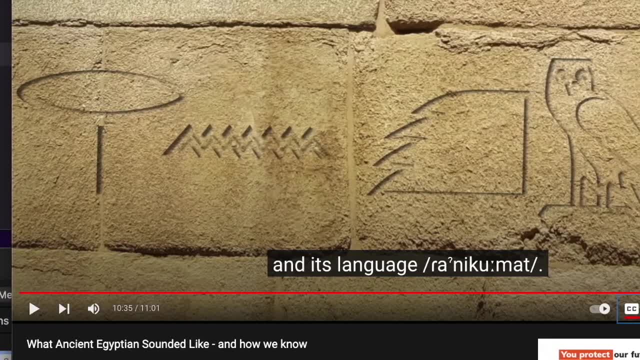 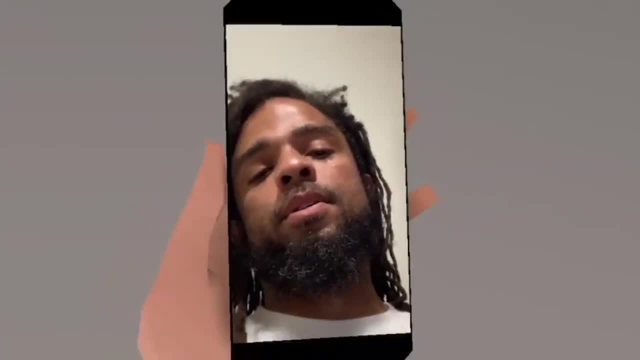 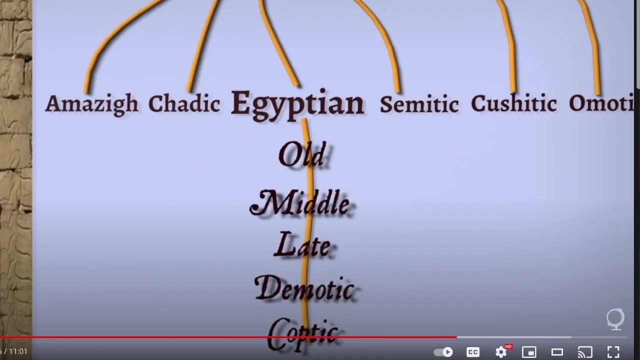 how long the vowels were or how you know um what they sounded like, if there were any right. but you know it's different and over time usually vowels- you know sounds- can change. you know people create new accents all the time, just like uh. within our society, you know, we've got languages evolving very. 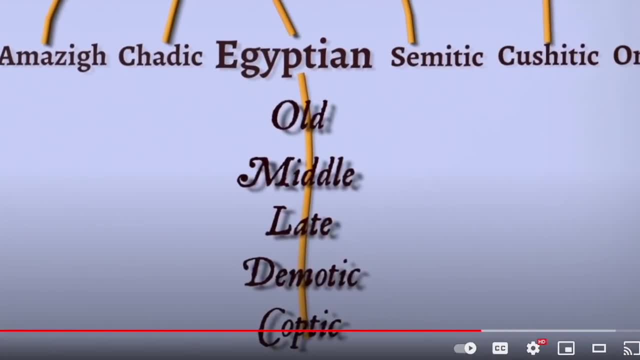 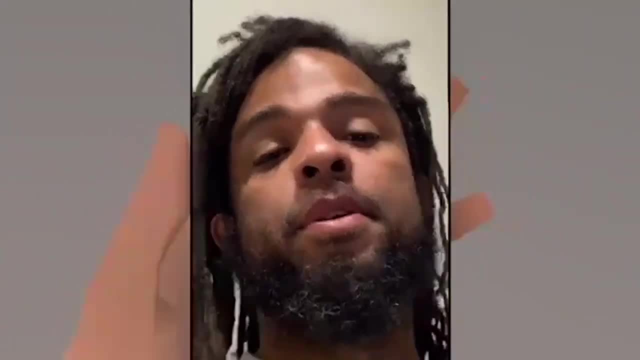 very quickly. um languages can evolve very, very quickly, um back in the day too. so just when you see the same glyphs, hieroglyphs, you don't know that you know they were always spoken the same way in every dynasty right, you can't assume that you know, you can never assume that, just like we. 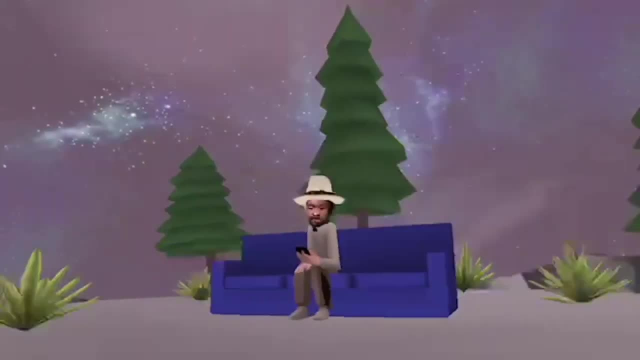 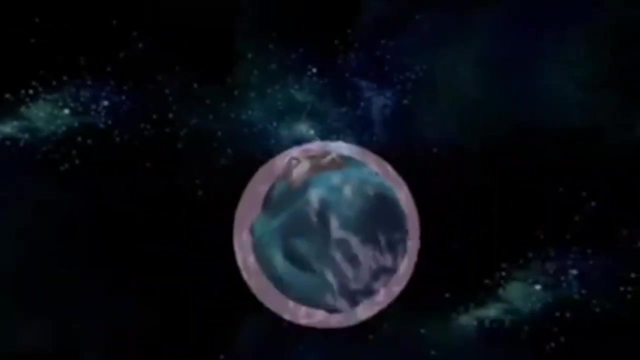 can't assume all these principles and physics apply to every universe in different multiverses, right? um, you know, another way of looking at is like in men in black. you know, when they go into the uh, you know they go into the actual uh. what do you call it? locker in the um? 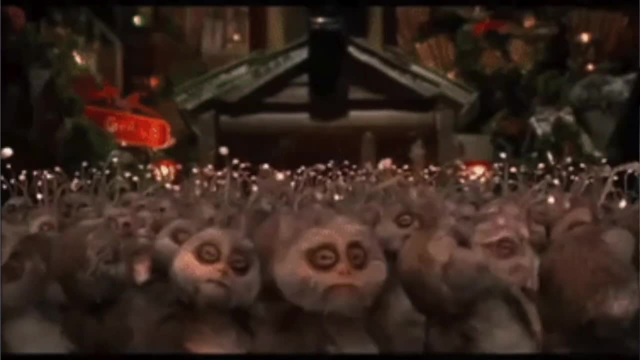 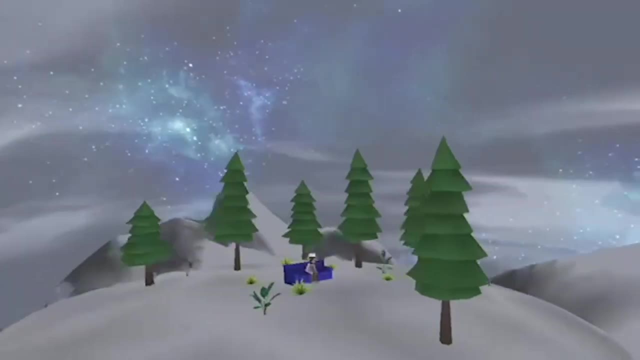 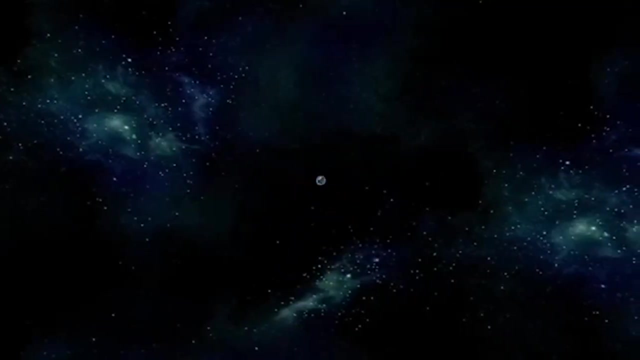 bus station or the train station, maybe it's like grand central station. um, i'm actually in men in black three back in time in warhol's uh party. i'm actually doing a cooking dance. shout out to to bass guy and shout out to seb- you know what i'm saying- his dj, but uh, yeah, so you know as. 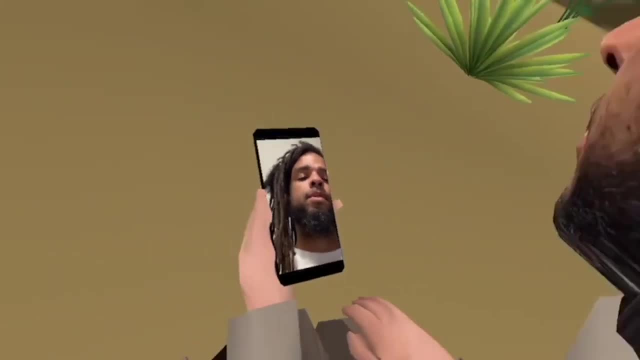 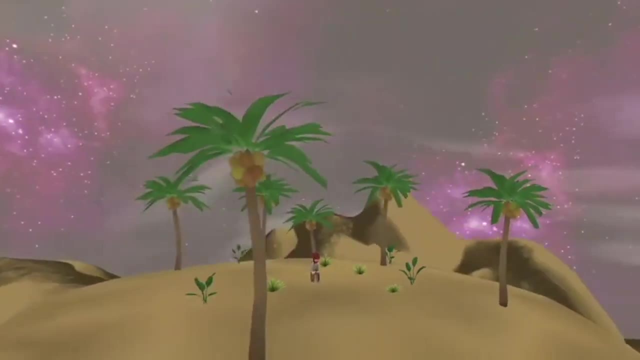 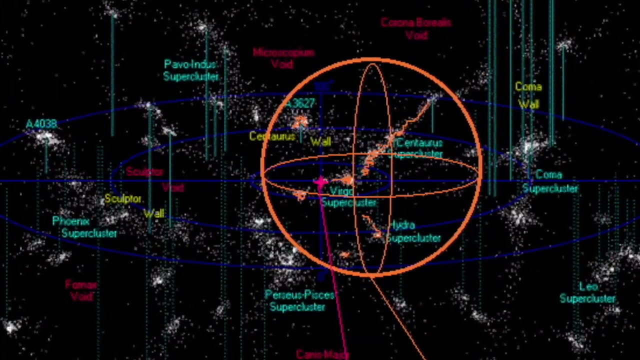 far as, like, time travel, different universes, you know all these things are all possible there's. you know there's infinite uh, planes and things like that. you know, and uh, even uh, you know, if you take the, the, the strings of uh, laniakia, you know the um, the name given to the, all the. 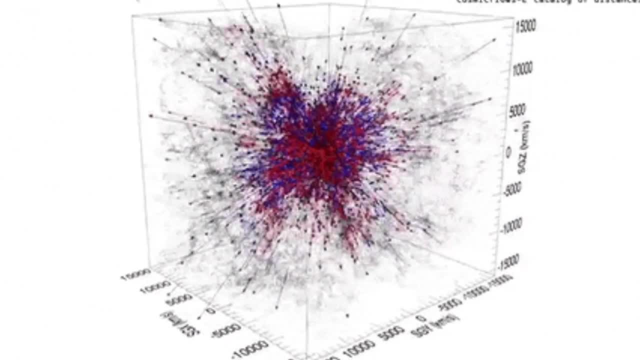 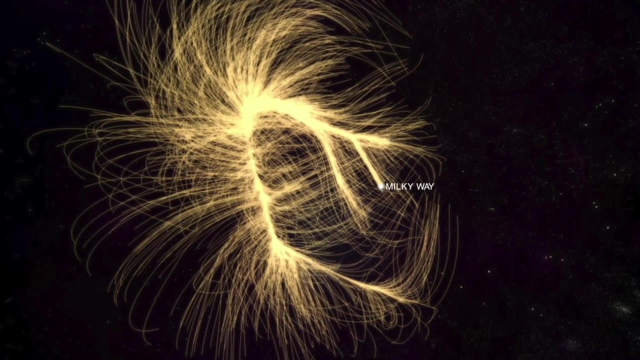 clusters of all the universes. um, that we know so far. you know, it looks like a, you know, like a, like a giant lung, like a tree, you know, and, and that's how we, uh, connect back to our ancestors in the fourth dimension. you know, i'm saying the fourth dimension, you know, would just show the. 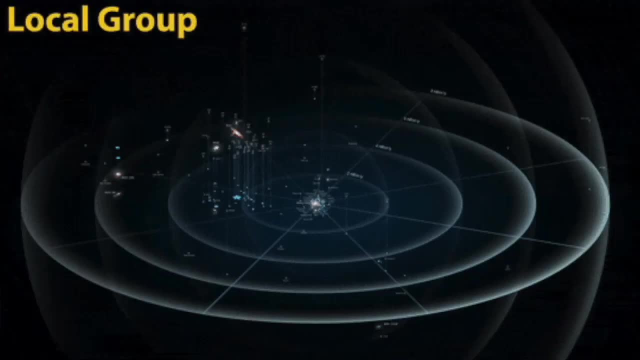 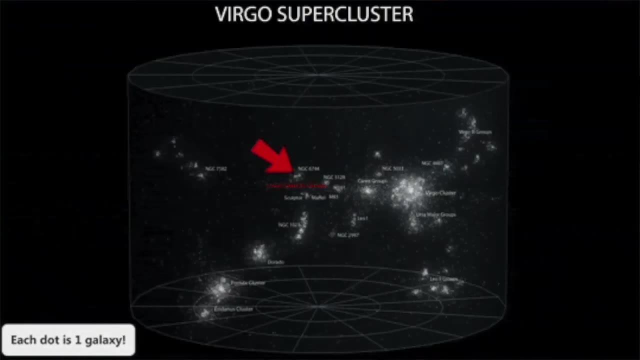 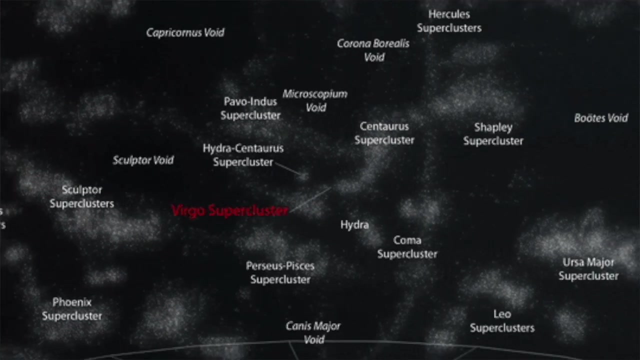 trail of your entire existence, which would look like a interweaving kind of a worm, or like more of an interweaving uh uh pattern of of knots. right, you're tying knots or loops. you know if you're going in a loop in life or if you're going to new places, if somebody's traveling around the. 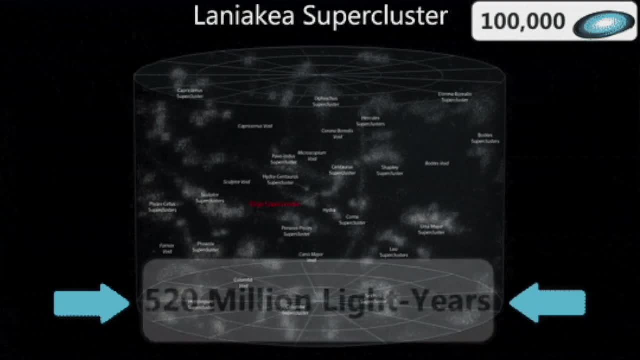 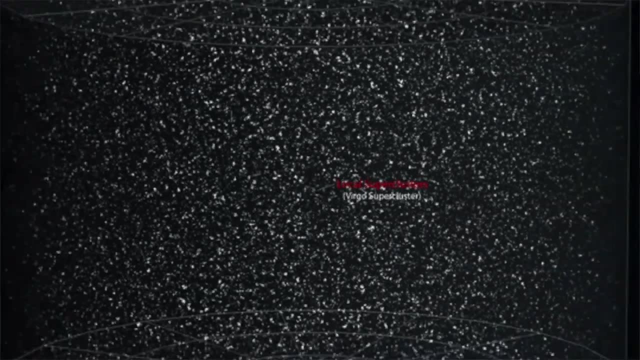 world and they're and always going to new places. it's not going to be loops where somebody's, you know, just going to the corner, going back home, um, is just going to be a loop of going to the corner back home and another, you know, you can. 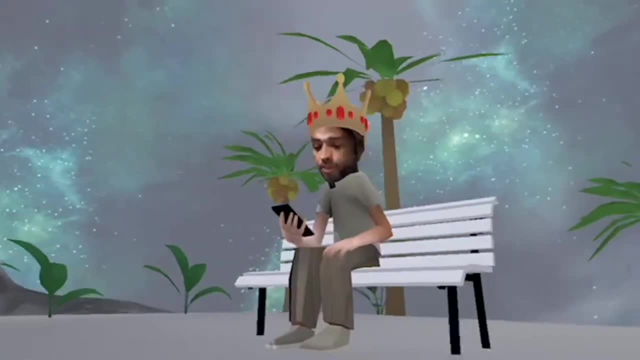 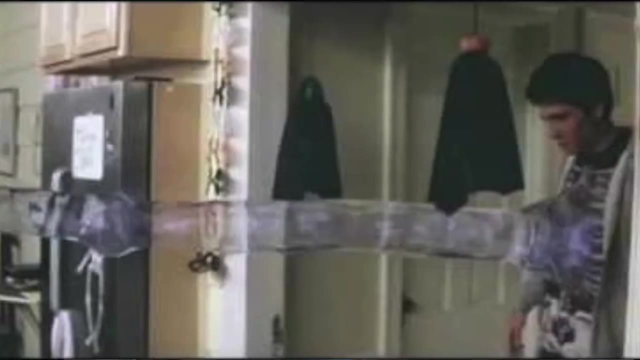 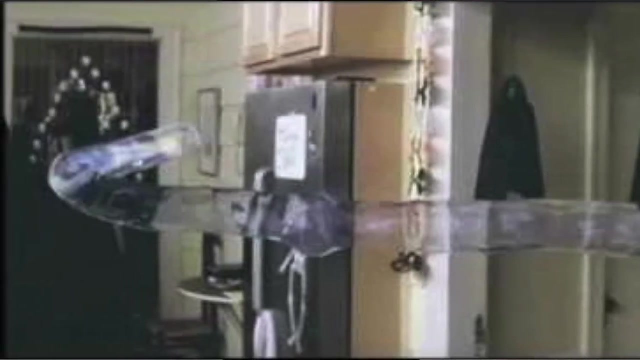 see this in donnie darko: uh, when, out of his solar plexus, um, the you know, his uh future is kind of showing. it's kind of showing him where he's going in the future. he's seeing his uh, he's stepping outside of time and seeing his fourth dimensional trail, you know, because to see your force, you know. 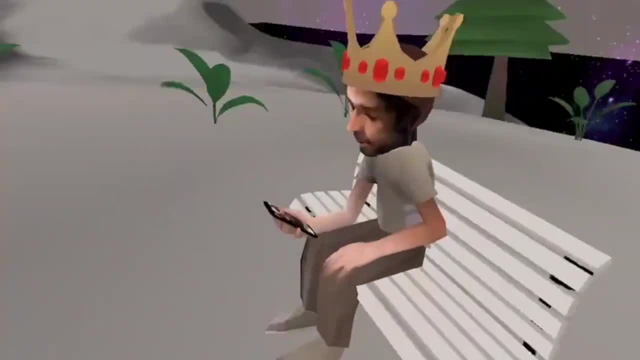 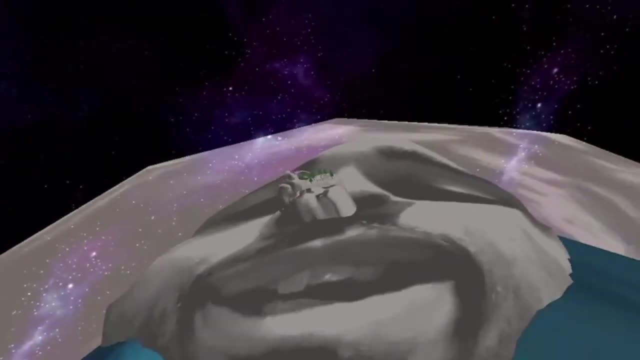 we can see our fourth dimensional trail when we wave our hands um, but to see the entire existence of the universe and the existence of the universe and the existence of the universe of you know, this universe as just an image is more like when you're traveling, the higher 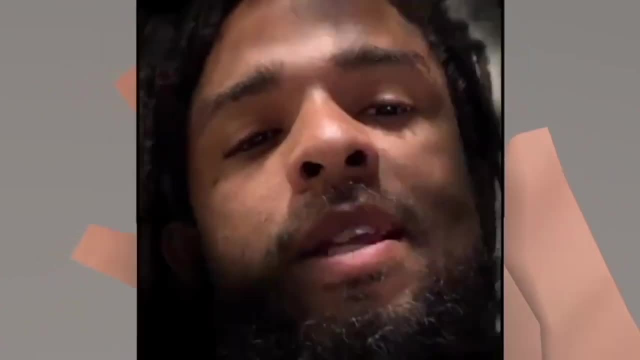 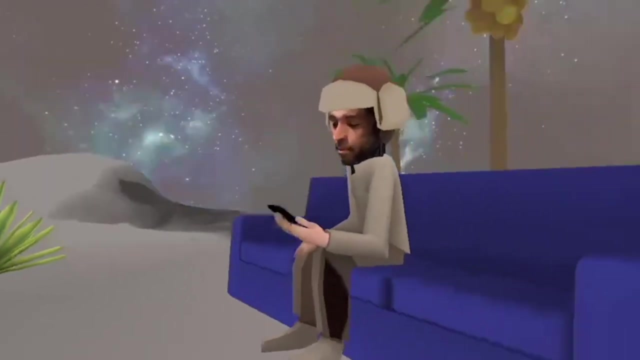 dimensions, like you know, seventh, eighth, ninth, tenth, i think the eighth is locked. i think the eighth dimension is locked. like i was saying before, uh, every, you know every dimension is not the same, but uh, yeah, as far as uh, you know the famine diagrams, you can see that the photon keeps. 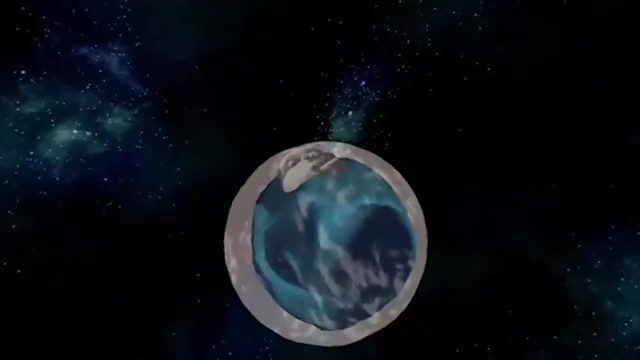 traveling. and then it and it splits into, uh, two q symbols- i'm assuming these are quarks right- and then it splits into two q symbols- i'm assuming these are quarks right- and then it splits into two q symbols- i'm assuming these are quarks right- and then it splits into two quarks right, and then a little glue on a little g. 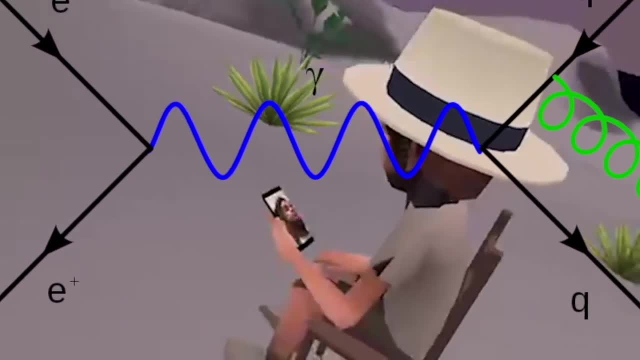 a little glue on a little g. a little glue on a little g, uh bounces off and into a little circle, or uh bounces off and into a little circle, or uh bounces off and into a little circle or circular spiral. you know so, these diagrams, 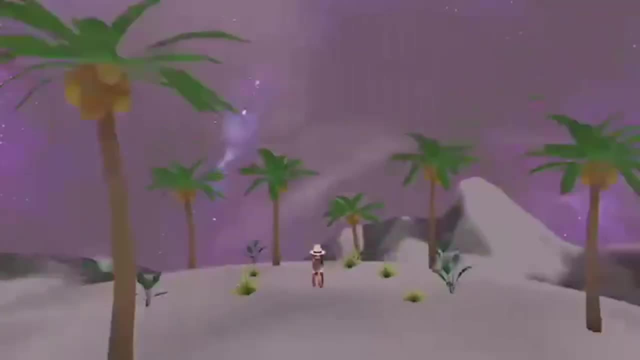 circular spiral. you know so these diagrams circular spiral. you know so these diagrams. you know they, uh are very, very similar ttm. you know they, uh are very, very similar ttm. you know they, uh are very, very similar ttm as well. i was influenced by these because 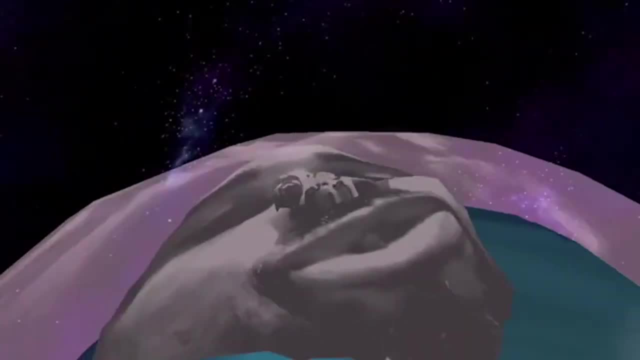 as well, i was influenced by these. because, as well, i was influenced by these. because, you know, ttm is uh essentially the fourth. you know, ttm is uh essentially the fourth. you know, ttm is uh essentially the fourth dimensional trail of the of the uh q. 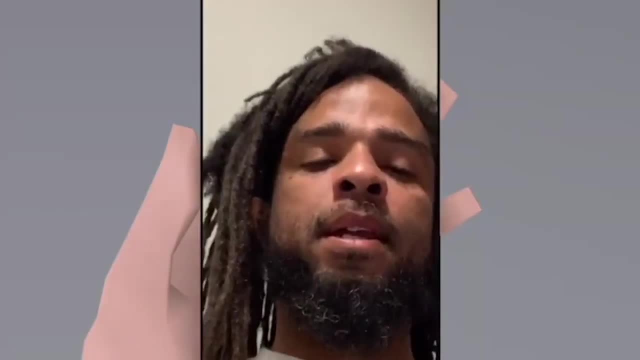 dimensional trail of the of the uh q. dimensional trail of the of the uh q point. you know so um ttm uh mechanics point. you know so um ttm uh mechanics point. you know so um ttm uh mechanics. and all you, all, everybody that has a 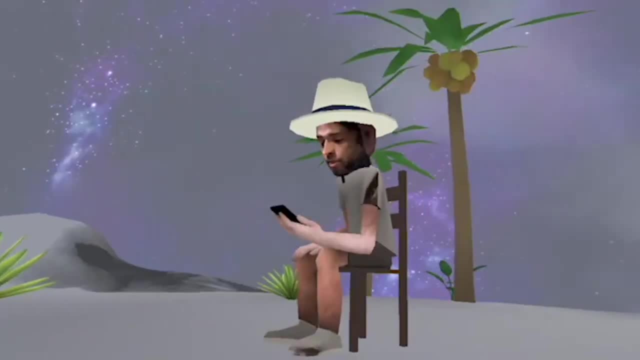 and all you all, everybody that has a, and all you all, everybody that has a matrix poster. you know these are all matrix poster. you know these are all matrix poster. you know these are all fourth dimensional movements of the fourth dimensional movements of the fourth dimensional movements of the crossfader over over time. i'm sorry, the. 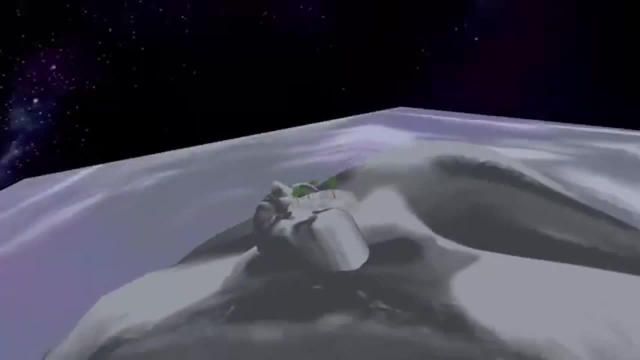 crossfader over over time. i'm sorry, the crossfader over over time, i'm sorry the. the q point, the q point, the q point over time and the clicks. you know the the over time and the clicks. you know the the over time and the clicks. you know the. the clicks represent the crossfader you. 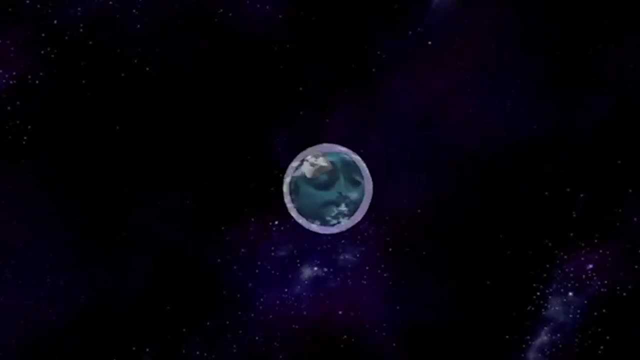 clicks represent the crossfader. you clicks represent the crossfader. you know because know, because know, because you know trigonometry is the movement of. you know trigonometry is the movement of. you know trigonometry is the movement of waves, but waves, but. 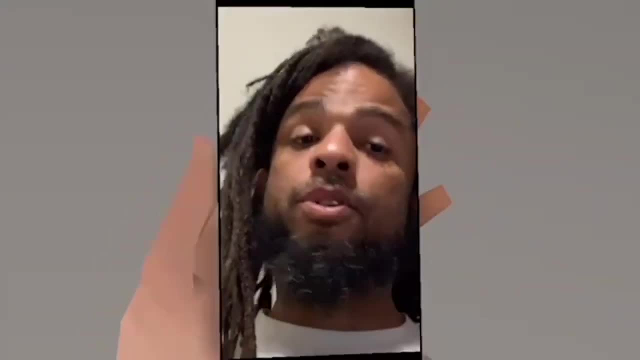 waves. but um calculus is when you start to cut. um calculus is when you start to cut. um calculus is when you start to cut those waves up, those waves up, those waves up. so what turntables are doing is calculus. so what turntables are doing is calculus. 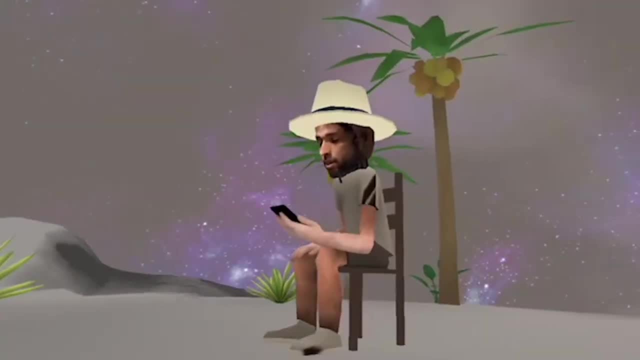 so what turntables are doing is calculus. you know what i'm saying. you know what i'm saying. you know what i'm saying. and that works with all reality, and, and that works with all reality, and, and that works with all reality, and existence, existence, existence in general. um, for those that don't know, 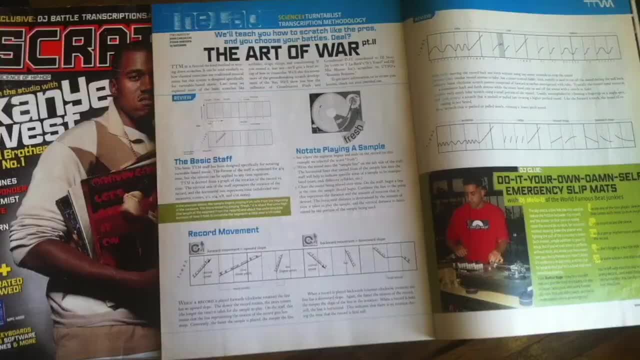 in general, um for those that don't know in general, um for those that don't know, um. about 21 years ago, um, about 21 years ago, um, i created something called the turntable um. i created something called the turntable um. i created something called the turntable transcription methodology, which is a. 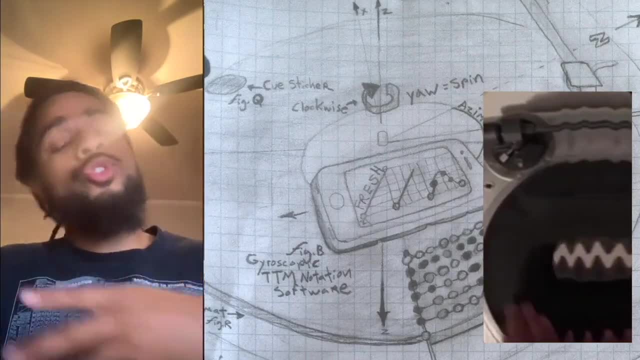 transcription methodology, which is a transcription methodology, which is a system of system of system of music notation for dj music that's used, music notation for dj music that's used, music notation for dj music that's used all around the world. all around the world, all around the world, they call it ttm turntable is. 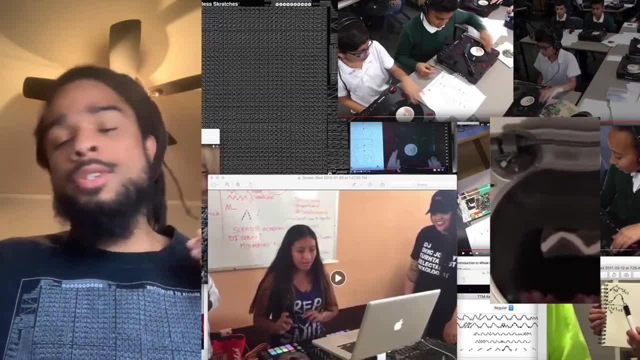 they call it ttm turntable. is they call it ttm turntable? is transcription methodology. the graph transcription methodology. the graph transcription methodology. the graph represents sounds right. represents sounds right. represents sounds right. it's used in elementary schools in the. it's used in elementary schools in the. 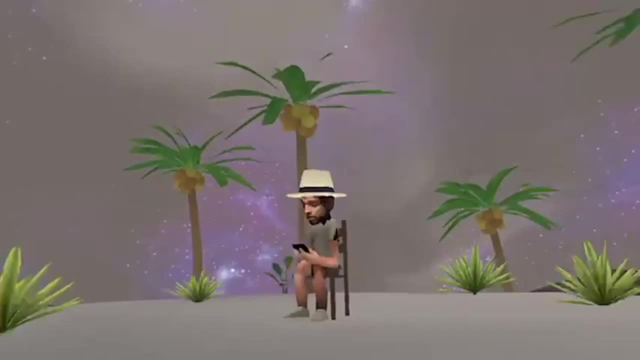 it's used in elementary schools in the uk. it's so i'm gonna uh just go over basically. so i'm gonna uh just go over, basically. so i'm gonna uh just go over basically. uh, uh on a deeper level. uh, what a photon. uh, uh, on a deeper level. uh, what a photon. 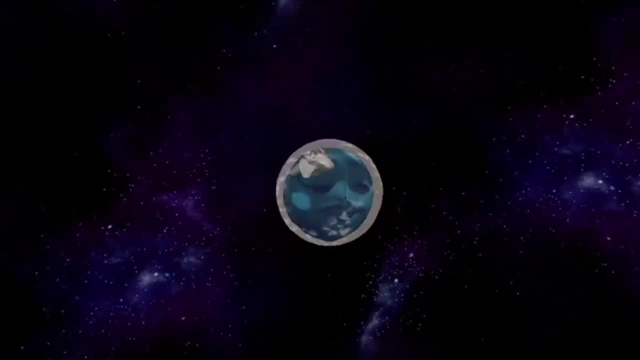 uh, uh, on a deeper level, uh, what a photon can do? can do, can do, um, um, even though you know photons are um, um, even though you know photons are um, um, even though you know photons are represented by gamma, you don't represented by gamma, you don't. 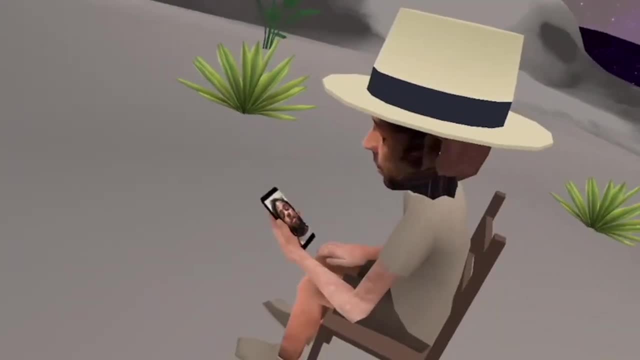 represented by gamma. you don't. it's important to note that they're not. it's important to note that they're not. it's important to note that they're not gamma rays. you know what i'm saying? the gamma rays. you know what i'm saying? the. 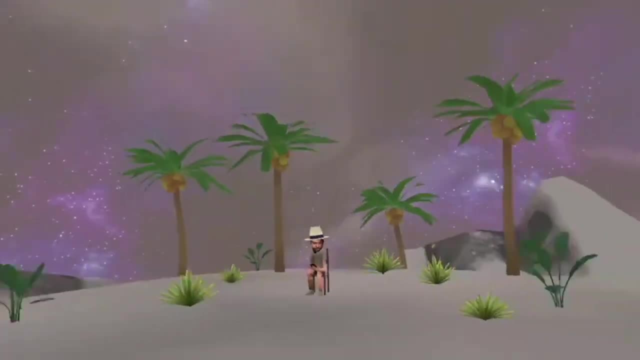 gamma rays. you know what i'm saying. the gamma ray is a type of gamma ray, is a type of gamma ray, is a type of of electro electromagnetic spectrum ray, of electro electromagnetic spectrum ray, of electro electromagnetic spectrum ray. but it's not all encompassing, it's just 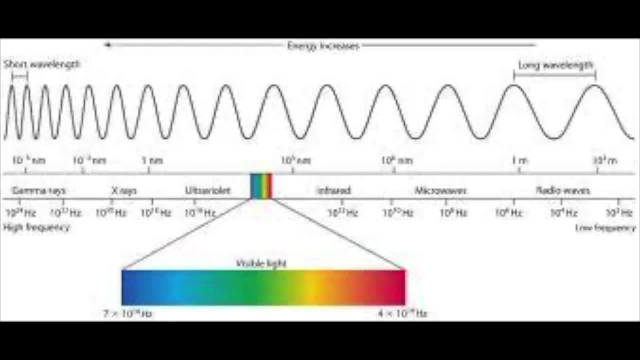 but it's not all encompassing. it's just, but it's not all encompassing. it's just one spectrum. gamma rays are just one, one spectrum. gamma rays are just one one spectrum. gamma rays are just one spectrum. you know the um our visual spectrum. you know the um our visual. 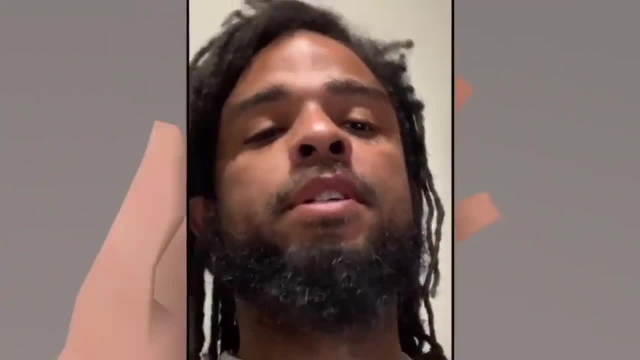 spectrum. you know the um our visual light spectrum is is just a limited light spectrum. is is just a limited light spectrum. is is just a limited spectrum, right, you know different insects spectrum, right, you know different insects spectrum, right, you know different insects. different animals can, different animals can. 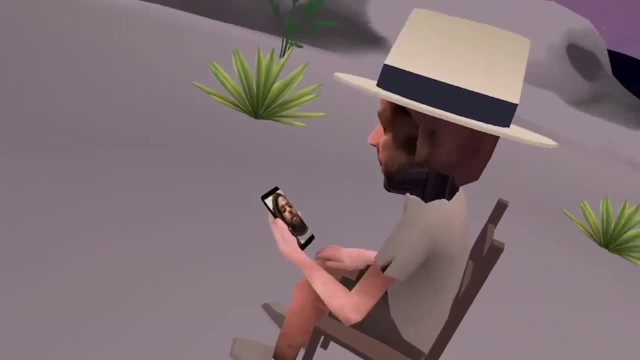 different animals can see much farther in different, see much farther in different, see much farther in different spectrums. but our spectrum is very much spectrums, but our spectrum is very much spectrums, but our spectrum is very much limited, limited, limited, um, you know, to the whole, uh, kind of. 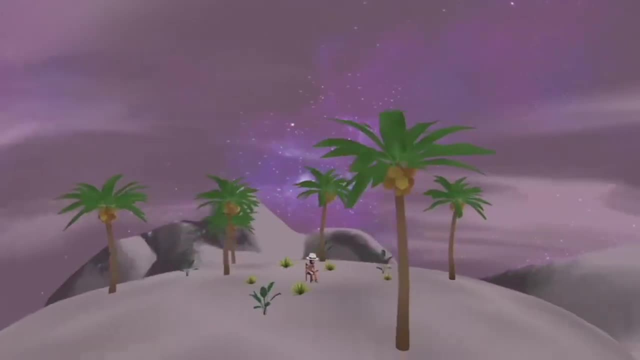 um, you know to the whole, uh kind of, um, you know to the whole, uh kind of rainbow spectrum, rainbow spectrum, rainbow spectrum, right, and then, uh, you know there's right, and then, uh, you know there's right, and then, uh, you know, there's infrared and ultraviolet below. 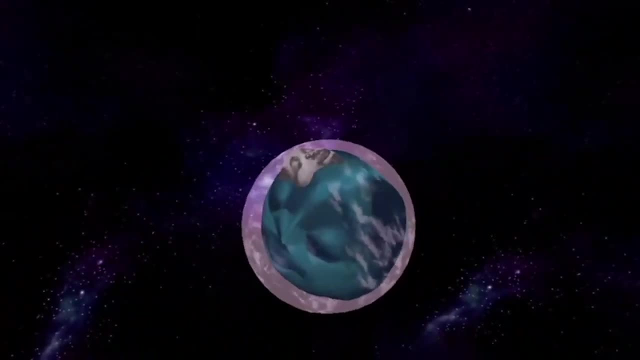 infrared and ultraviolet, below infrared and ultraviolet, below, below and above us, um you know. and then below and above us, um you know. and then below and above us, um you know. and then he gets all these, he gets all these, he gets all these other types of waves and things like. 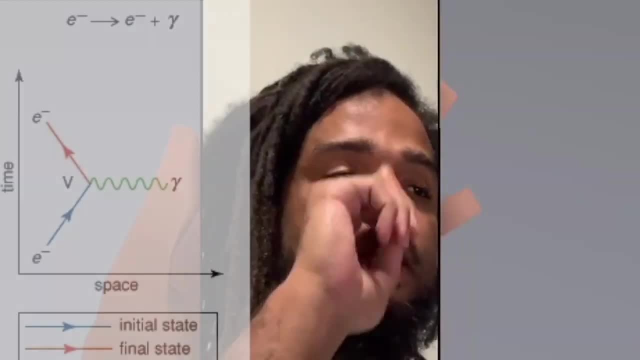 other types of waves and things like other types of waves and things like that. that that you know so the so, even though they use- you know so the so, even though they use- you know so the so- even though they use the greek gamma symbol, the greek gamma symbol. 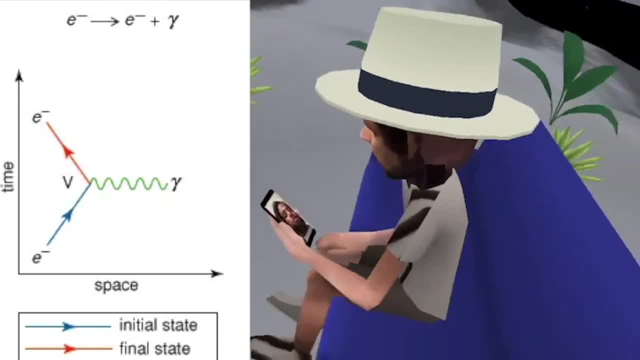 the greek gamma symbol for uh. the photon photons are not only for uh. the photon photons are not only for uh. the photon photons are not only gamma rays. that's what i just wanted to gamma rays. that's what i just wanted to gamma rays. that's what i just wanted to make clear. 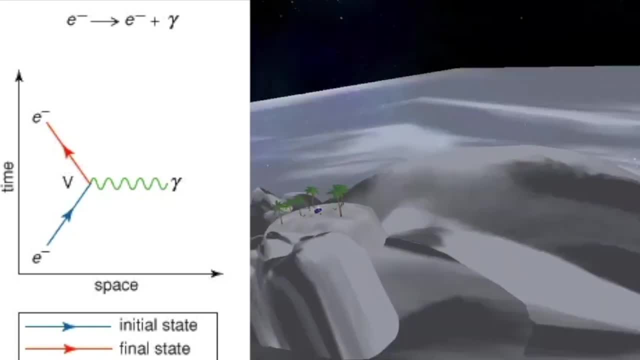 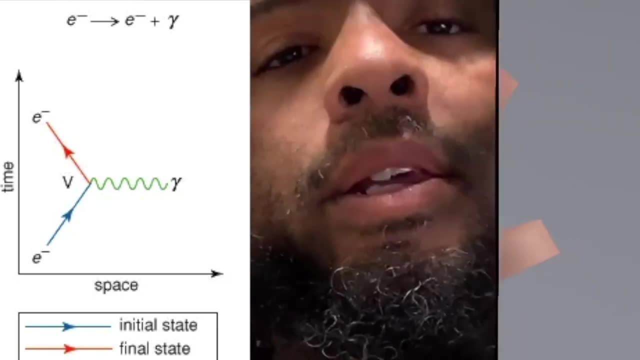 make clear, make clear. all right, so now, all right, so now, all right. so now, if you think about um uh, if you think about um uh, if you think about um uh particle wave duality, the fact that um particle wave duality, the fact that um particle wave duality, the fact that um, you know the copenhagen uh experiments. 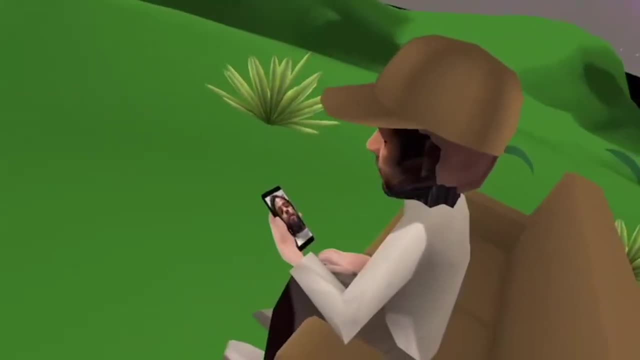 you know the copenhagen uh experiments. you know the copenhagen uh experiments showed us that. showed us that. showed us that you know when uh uh. you know when uh uh. you know when uh uh. when a particle, when a photon is shot. when a particle, when a photon is shot. 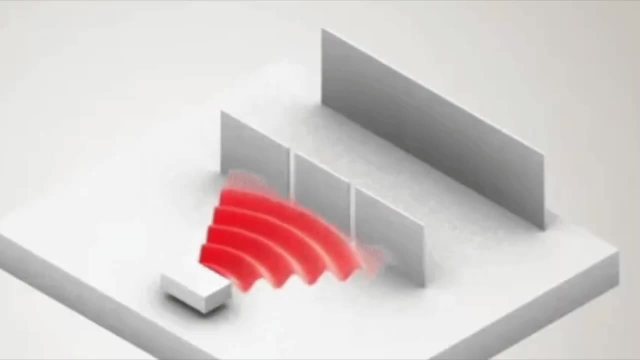 when a particle, when a photon is shot through through, through, um it can act like a wave, or it can act um, it can act like a wave, or it can act um, it can act like a wave, or it can act like like, like a particle, depending on. you know, if the a particle, depending on you know if the a particle, depending on you know if the person's looking at it or not, and that person's looking at it or not, and that person's looking at it or not, and that kind of goes to the you know tree falls. 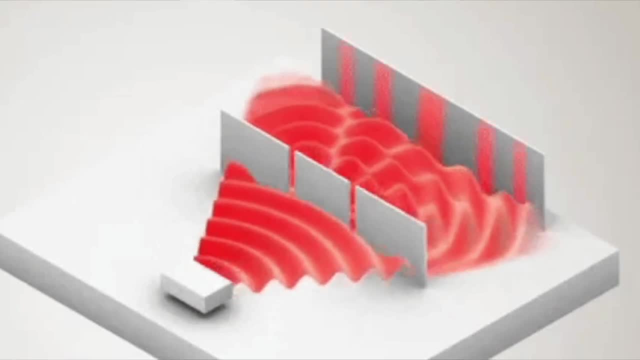 kind of goes to the you know tree falls kind of goes to the you know tree falls in the forest, in the forest, in the forest, kind of thing, um, and does it? does it kind of thing, um, and does it. does it kind of thing, um, and does it? does it make a sound? 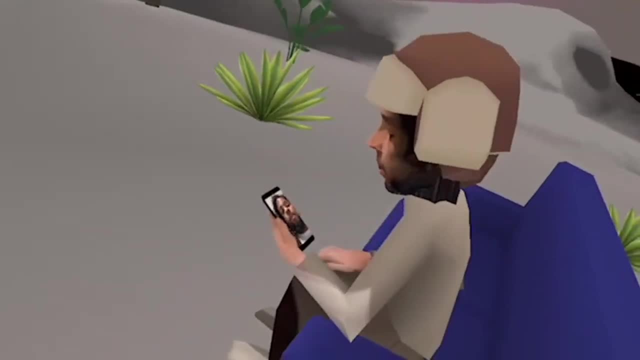 make a sound. make a sound. and you know the copenhagen experiment. and you know the copenhagen experiment and you know the copenhagen experiment shows us it's different, you know. shows us it's different, you know. shows us it's different, you know it. it doesn't necessarily make a sound. 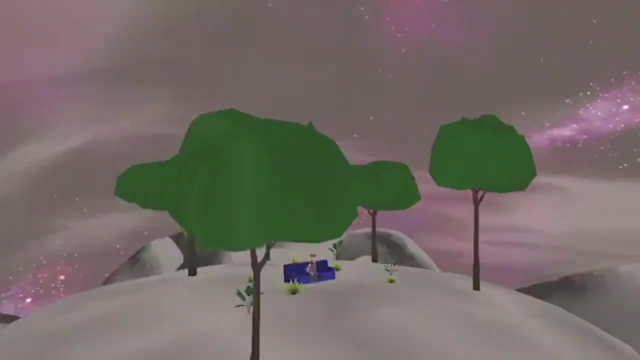 it it doesn't necessarily make a sound. it it doesn't necessarily make a sound if you're not there. if you're not there, if you're not there, experiencing it- and you know what i'm experiencing it and you know what i'm experiencing it and you know what i'm saying. like, obviously, things are. 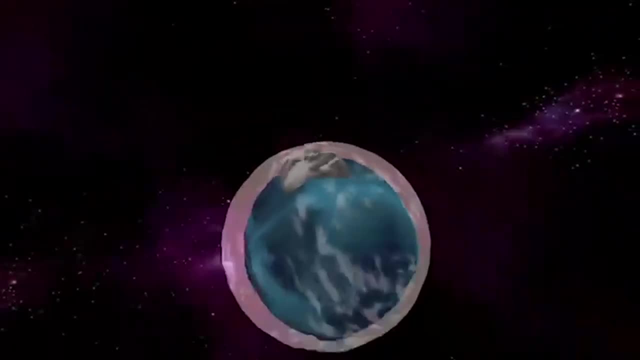 saying like obviously things are saying, like obviously things are happening, happening, happening. but uh, you know they call them quiff. but uh, you know they call them quiff. but uh, you know they call them quiff, pops and quiff. you know um pops and quiff, you know um. 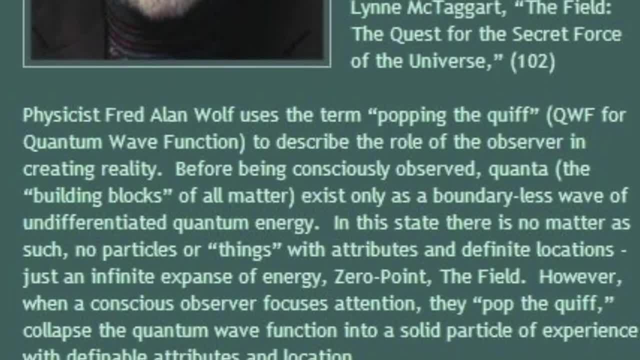 pops and quiff. you know, um the, the, the seeing the experience, um actually uh seeing the experience, um actually uh seeing the experience. um actually uh affects the experience. so there's no affects the experience. so there's no affects the experience. so there's no such thing as. 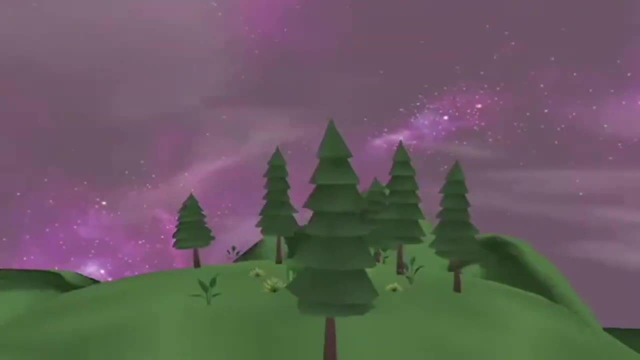 such thing as such thing as an objective experience, because when you an objective experience, because when you an objective experience, because when you, when you're actually viewing something, when you're actually viewing something, when you're actually viewing something, it's actually affecting that thing that it's actually affecting that thing that 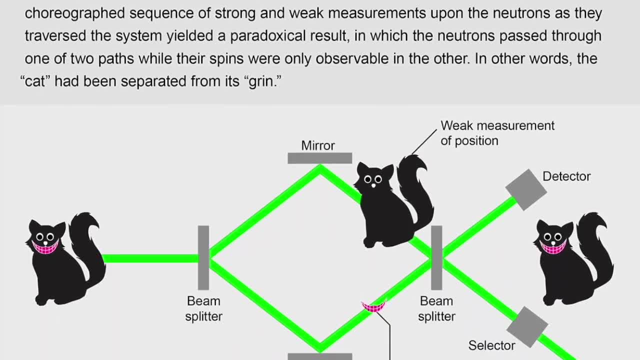 it's actually affecting that thing that you're viewing. you're viewing, you're viewing. you know what i'm saying and also look, you know what i'm saying and also look, you know what i'm saying and also look up the book of optics, up the book of optics. 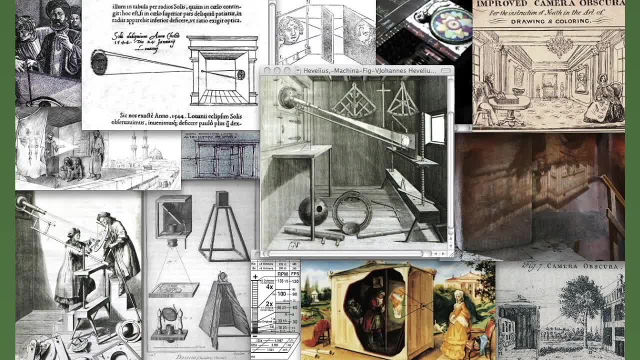 up the book of optics. you know what i'm saying by by uh. you know what i'm saying by by uh. you know what i'm saying by by uh. al-hazan, the book of optics. because the al-hazan, the book of optics, because the 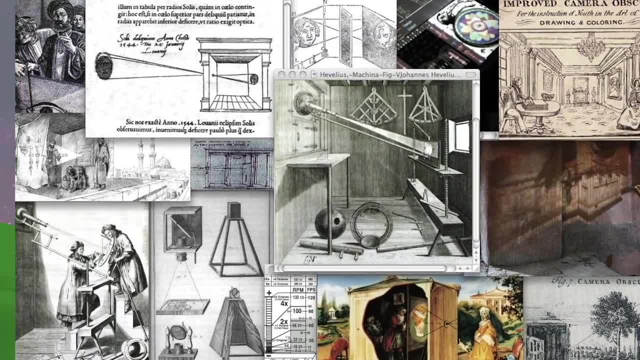 al-hazan, the book of optics. because the book of optics, you know that's the first book of optics. you know that's the first book of optics. you know that's the first book that we know about book, that we know about book, that we know about, about optics. you know what i'm saying? uh. 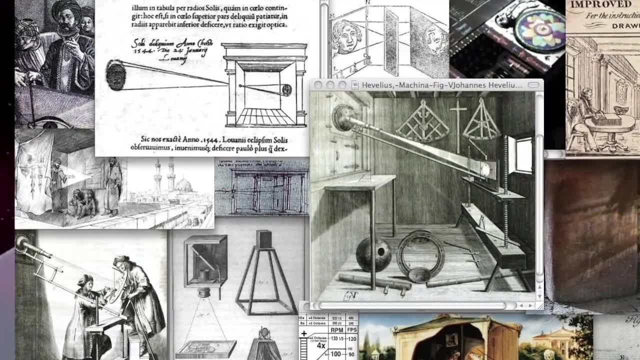 about optics. you know what i'm saying, uh, about optics. you know what i'm saying, uh, and this was written by a black man, and this was written by a black man, and this was written by a black man, you know, uh, over a thousand years ago. i. 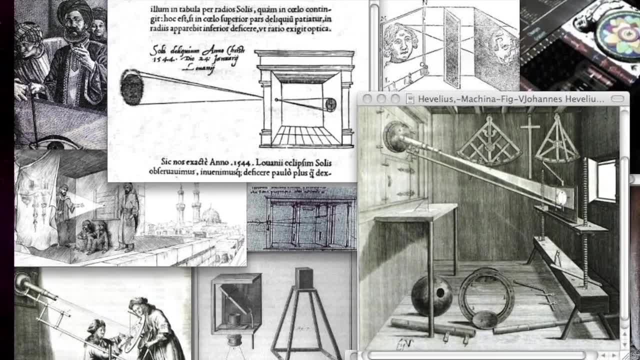 you know, uh, over a thousand years ago. i, you know, uh, over a thousand years ago. i, believe, believe, believe. and you know they've tried to whitewash and you know they've tried to whitewash and you know they've tried to whitewash him over the years. but look for the 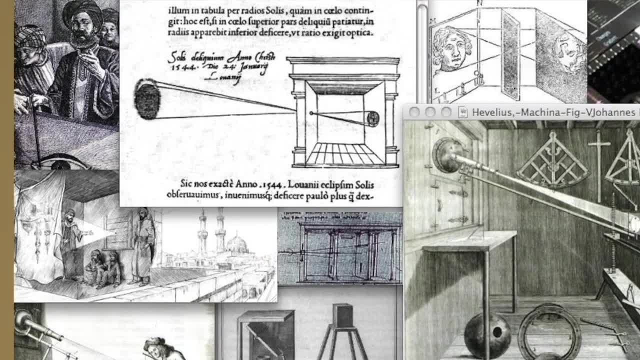 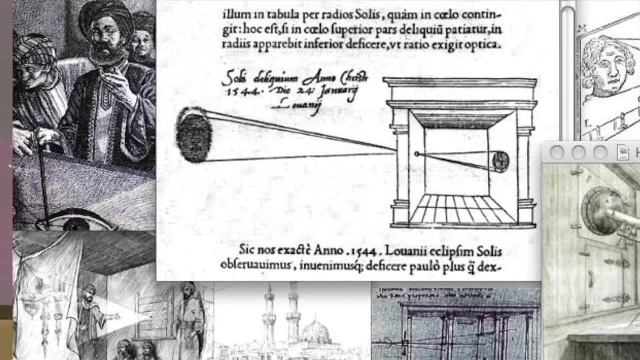 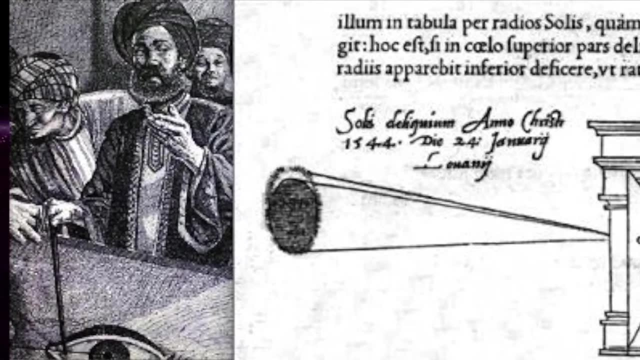 him over the years. but look for the him over the years. but look for the book showing just like a bunch of uh book showing just like a bunch of uh book showing just like a bunch of uh stuff drawn in the 1950s and 40s. you 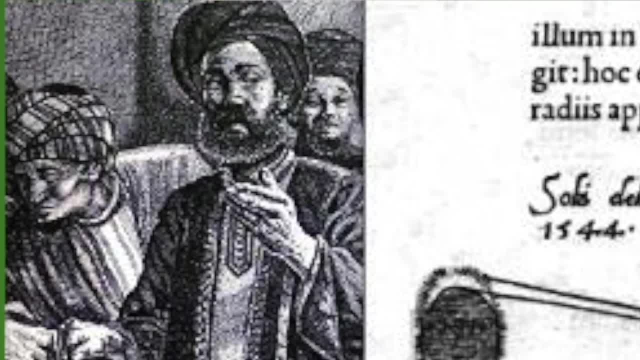 stuff drawn in the 1950s and 40s. you stuff drawn in the 1950s and 40s. you know, know, know 60s. you know different types of 60s. you know different types of 60s. you know different types of drawings. but you know you gotta go. 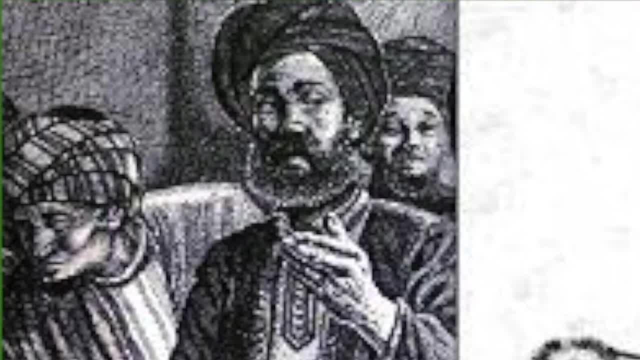 drawings. but you know you gotta go drawings, but you know you gotta go, gotta really research, because so um gotta really research, because so um gotta really research, because so, um, you know, look up for for al-hazan uh, you know, look up for for al-hazan uh. 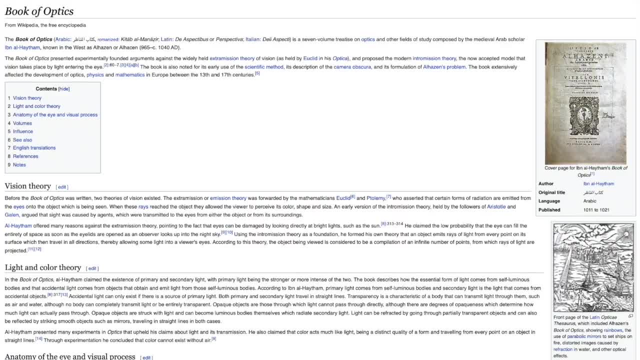 you know, look up for for al-hazan, uh, but uh, yeah, so the book of optics. but uh, yeah, so the book of optics, but uh, yeah, so the book of optics, book of optics and, and i feel like that book of optics and and i feel like that. 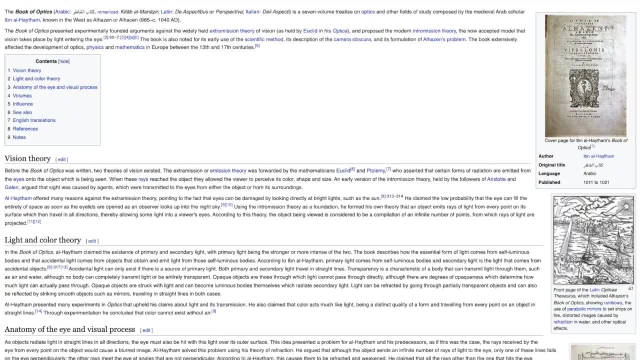 book of optics and, and i feel like that was his greek name. uh was his greek name. uh was his greek name. uh, you know um. i forget what his uh full. you know um. i forget what his uh full. you know um. i forget what his uh full muslim name was. but uh. 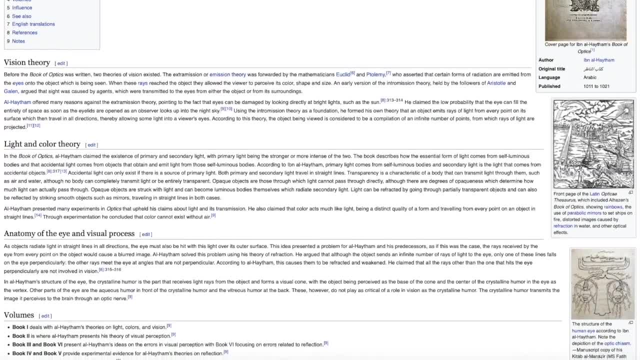 muslim name was, but uh, muslim name was, but uh. um, i'll show the screenshot of all these. um, i'll show the screenshot of all these, um, i'll show the screenshot of all these. you know things that i'm talking about. you know things that i'm talking about. 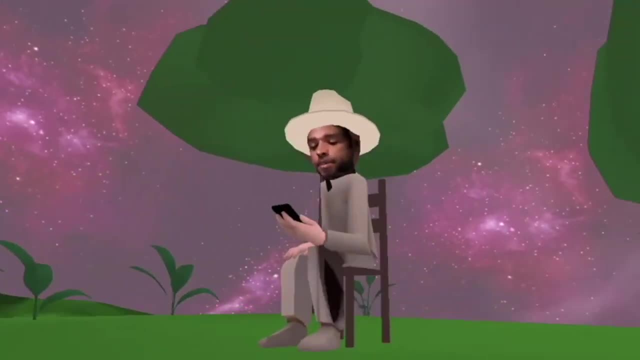 you know things that i'm talking about, um, but yeah, the book of optics. you know, um, but yeah, the book of optics. you know, um, but yeah, the book of optics. you know because before, because before, because before that you know a lot of the uh the that. you know a lot of the uh the. 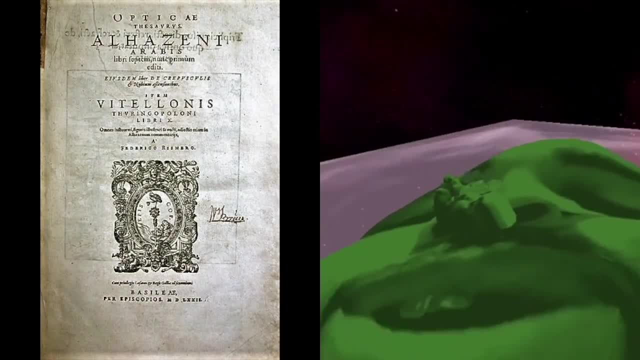 that you know a lot of the uh the people living, uh um people living, uh um people living, uh um. you know from coming from the dark ages. you know from coming from the dark ages. you know from coming from the dark ages. they thought that photons were shooting. 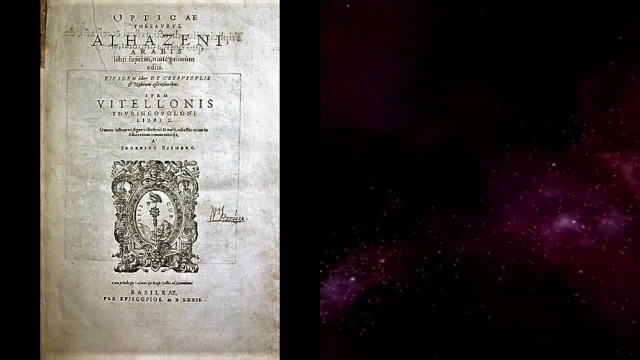 they thought that photons were shooting. they thought that photons were shooting out of our eyes, out of our eyes, out of our eyes. and scanning things, you know, and he was. and scanning things, you know, and he was. and scanning things, you know, and he was one of the first to. 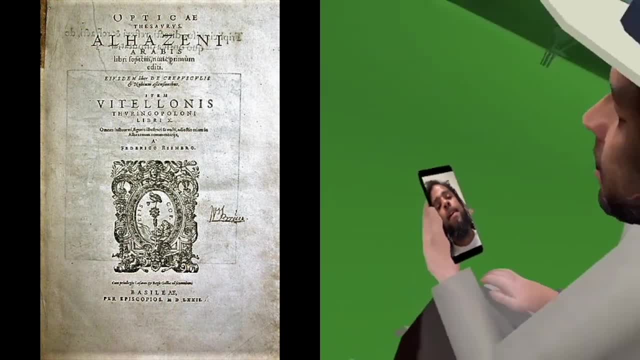 one of the first to one of the first to really put it down in a modern book, really put it down in a modern book, really put it down in a modern book. format, format, format. uh, you know in arabic, you know what i'm? uh, you know in arabic, you know what i'm. 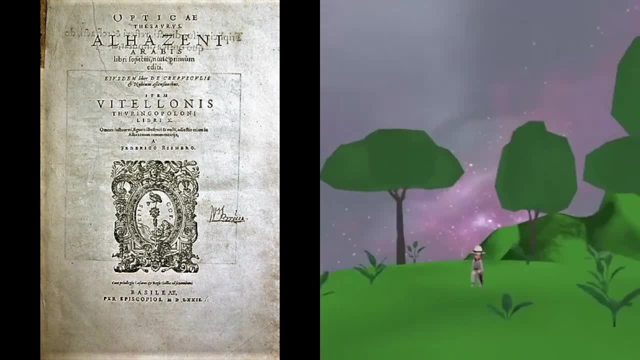 uh, you know in arabic, you know what i'm saying? that saying that, saying that, uh, the photons and the light and the, uh, the photons and the light and the, uh, the photons and the light, and the things are coming into our eye. things are coming into our eye. 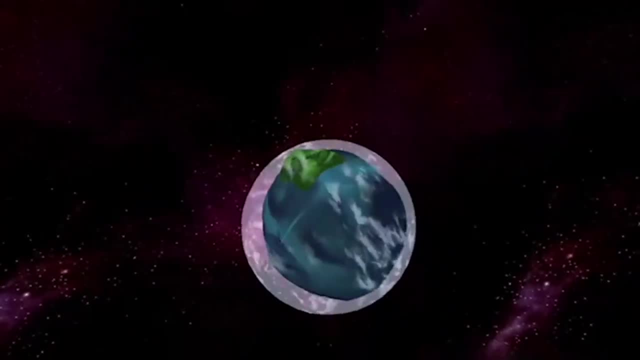 things are coming into our eye. you know what i'm saying so definitely. you know what i'm saying so definitely. you know what i'm saying so definitely. look up the book of optics. look up the book of optics. look up the book of optics. um, yeah, so with the famine, 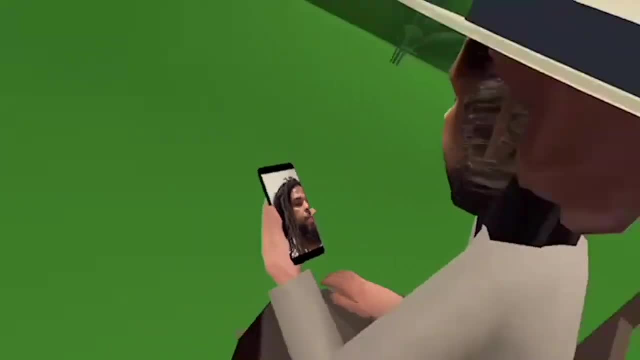 um, yeah, so with the famine. um, yeah, so with the famine diagrams. i'm just going to read a little diagrams. i'm just going to read a little diagrams. i'm just going to read a little bit from uh from wikipedia, bit from uh from wikipedia, bit from uh from wikipedia. so the photon is a type of elementary. 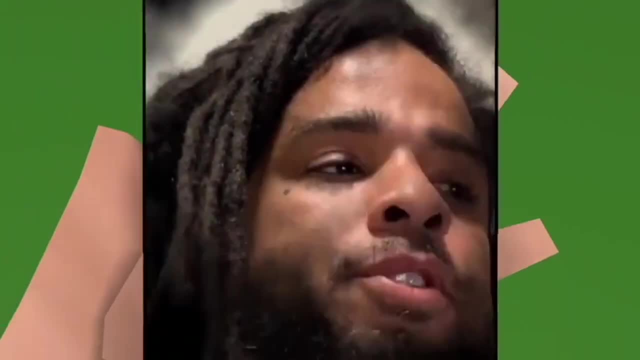 so the photon is a type of elementary. so the photon is a type of elementary carrier for the electromagnetic force. carrier for the electromagnetic force, carrier for the electromagnetic force. photons are massless, so they always move. photons are massless, so they always move. photons are massless, so they always move at the speed of light. 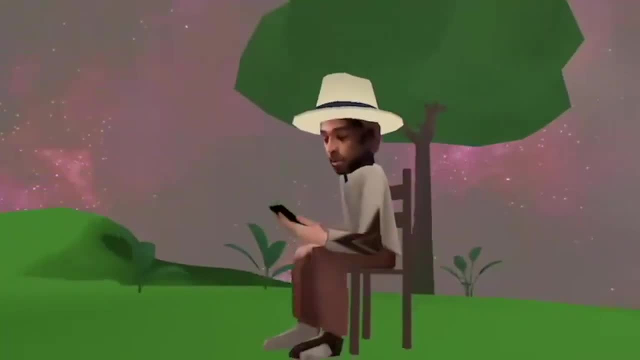 at the speed of light, at the speed of light in a vacuum right and in a vacuum right and in a vacuum right. and our bodies are made out of of light out. our bodies are made out of of light out. our bodies are made out of of light, out of photons, but they're wrapped in. 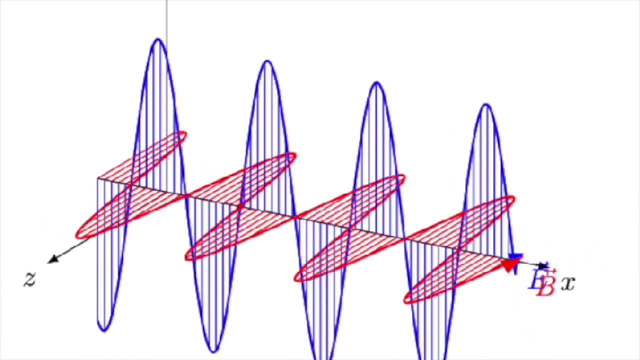 of photons, but they're wrapped in of photons, but they're wrapped in magnetism, so they're magnetism, so they're magnetism, so they're. you know, uh, they become other particles. you know, uh, they become other particles. you know, uh, they become other particles, and things like that. 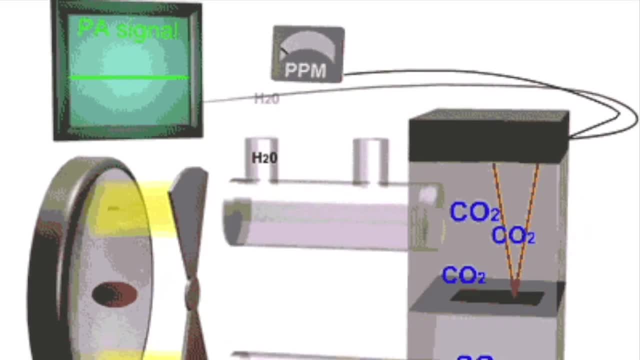 and things like that and things like that, like, and that's what the fame and like. and that's what the fame and like and that's what the fame and diagrams can show us like when you're diagrams can show us like when you're diagrams can show us like when you're mixing chemicals up. 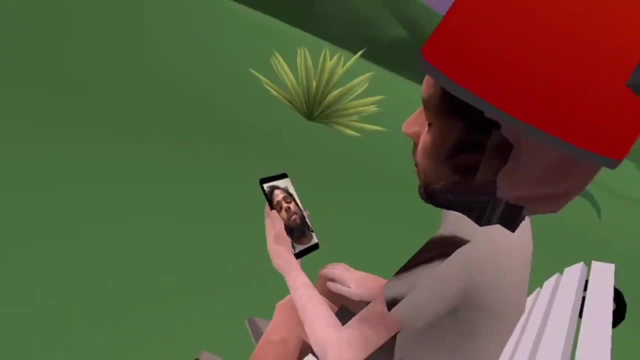 mixing chemicals up, mixing chemicals up. you know uh these different chemicals? you know uh these different chemicals. you know uh these different chemicals? are are being mixed up together, are are being mixed up together. are are being mixed up together and uh they're forming different uh and uh they're forming different uh. 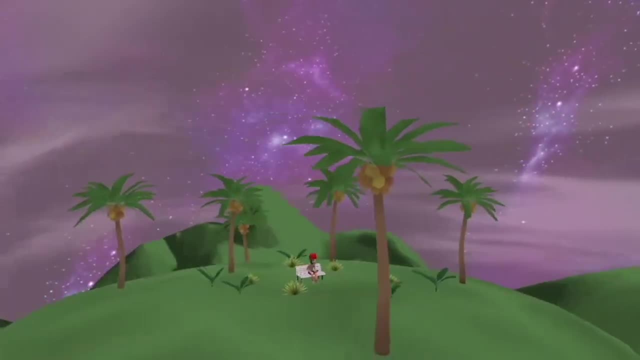 and, uh, they're forming different, uh, new strands of molecules. and you know new strands of molecules and you know new strands of molecules. and you know, certain things are bonding, certain certain things are bonding, certain certain things are bonding. certain things are knocking each other um. things are knocking each other um. 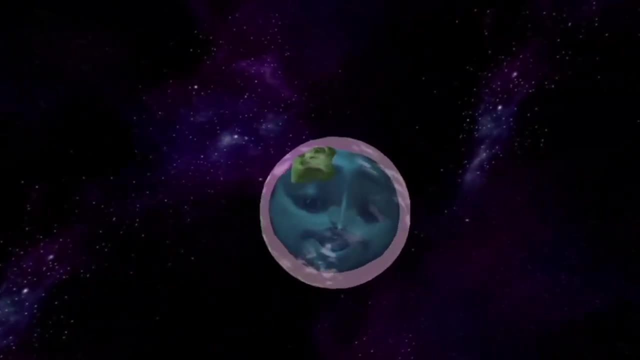 things are knocking each other um, out of a a certain bond, and you know, out of a, a certain bond, and you know, out of a a certain bond, and you know, things can alter and change, you know, and things can alter and change, you know, and things can alter and change, you know, and we call that that chemistry, right? 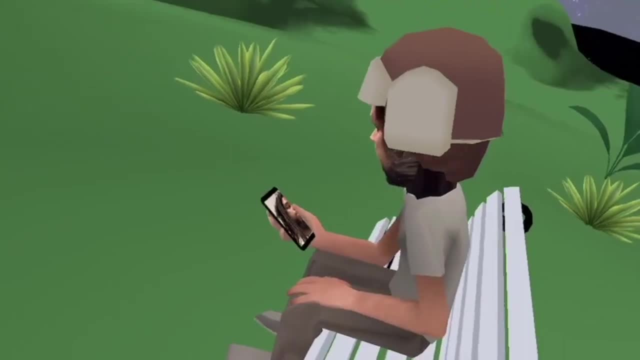 we call that that chemistry right. we call that that chemistry right. um so so, to continue that the photon, um so so, to continue that the photon. um so so to continue that the photon belongs to the class of bosons, belongs to the class of bosons, belongs to the class of bosons, like all elementary particles, photons. 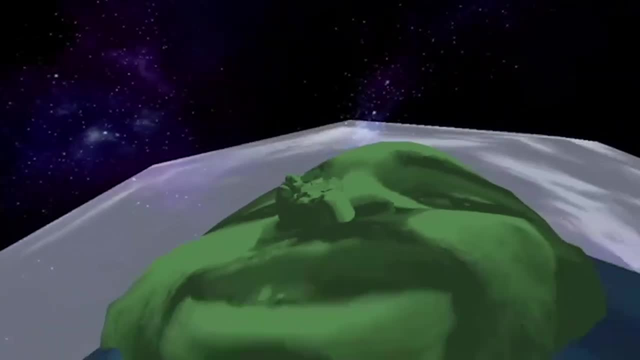 like all elementary particles, photons. like all elementary particles, photons are currently best explained by quantum, are currently best explained by quantum, are currently best explained by quantum mechanics: mechanics mechanics and exhibit wave particle duality and exhibit wave particle duality and exhibit wave particle duality, their behavior, and that's what i was. 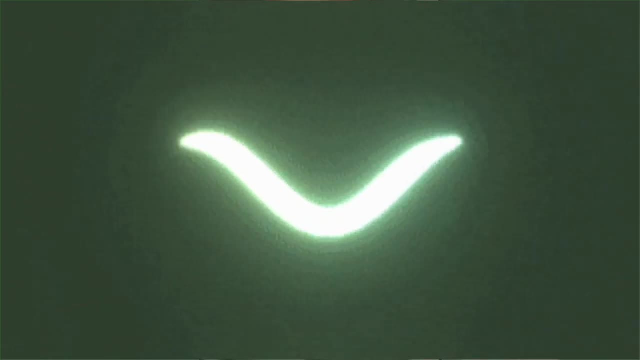 their behavior and that's what i was their behavior and that's what i was talking about: the? uh the copenhagen, talking about the uh the copenhagen, talking about the? uh the copenhagen experiment, because, as far as particle experiment, because, as far as particle experiment, because, as far as particle wave duality, 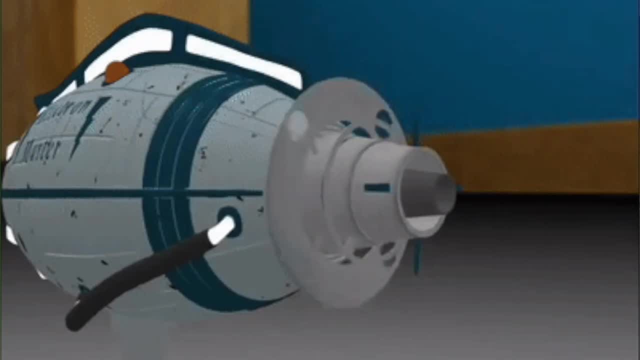 wave duality, wave duality. um, you know when they shot those. um, you know when they shot those. um, you know when they shot those photons through the double slit, photons through the double slit, photons through the double slit. um, you know, sometimes they were acting. um, you know, sometimes they were acting. 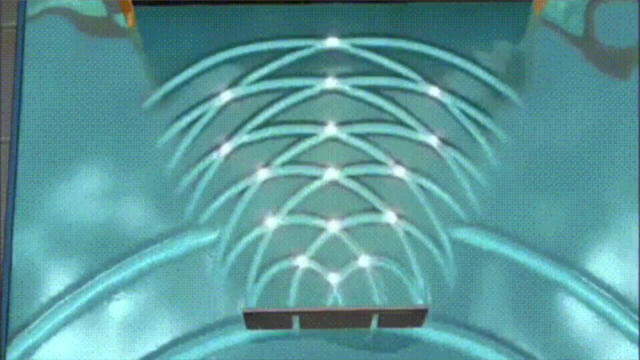 um, you know, sometimes they were acting like, like, like, uh, it was a wave going through the two. uh, it was a wave going through the two. uh, it was a wave going through the two double slits. and sometimes they act like double slits and sometimes they act like. 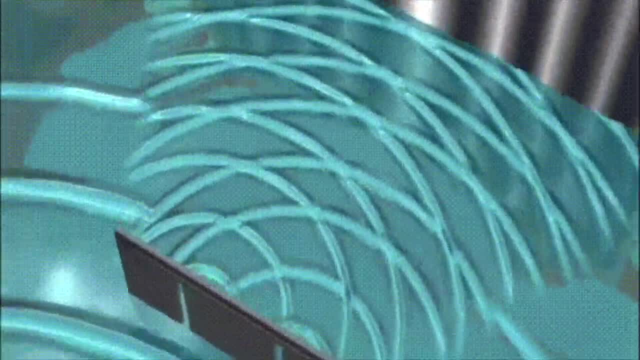 double slits and sometimes they act like there was like a shotgun blast. and there was like a shotgun blast and there was like a shotgun blast and there's a bunch of uh little particles. there's a bunch of uh little particles. there's a bunch of uh little particles going through the double, the double split. 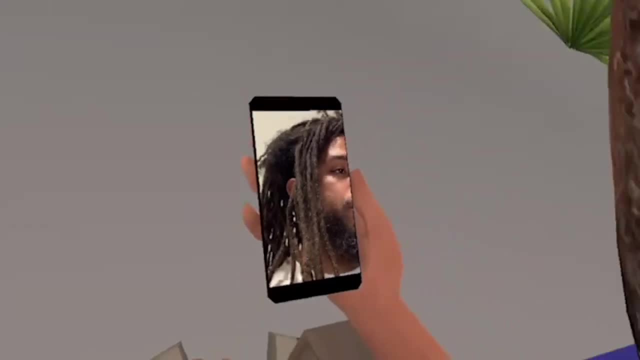 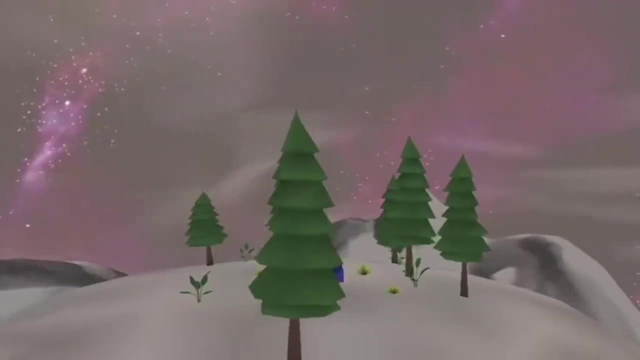 going through the double, the double split, going through the double, the double split, right, right, right, um, um, um, so, so, so, their behavior, featuring properties of their behavior, featuring properties of their behavior, featuring properties of both waves and particles, both waves and particles, both waves and particles. right, so that, so you know if we're made. right so that. so you know if we're made right so that. so you know if we're made out of that, if we're made out of photons out of that, if we're made out of photons out of that, if we're made out of photons encapsulated in. 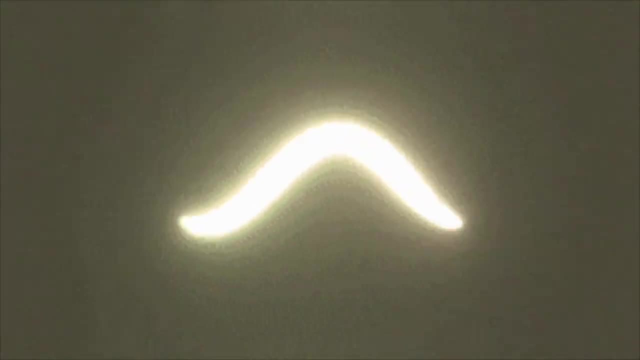 encapsulated in. encapsulated in and um and um and um. magnetism- different types of magnetism. magnetism: different types of magnetism. magnetism: different types of magnetism. then that you know that that goes with, then that you know that that goes with, then that you know that that goes with that. you know as well, you know what i'm. 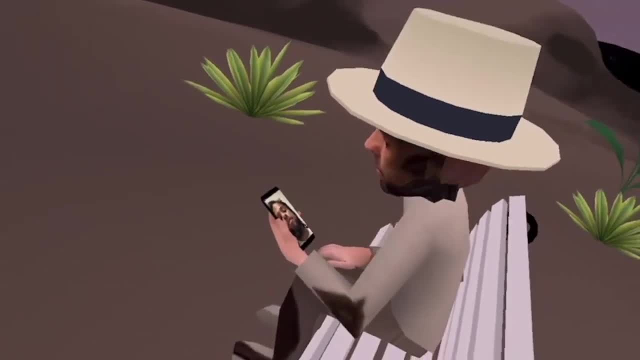 that you know as well, you know what i'm, that you know as well, you know what i'm saying. because we you can bump down saying, because we you can bump down saying, because we you can bump down using energy, you can bump down, uh, using energy, you can bump down, uh. 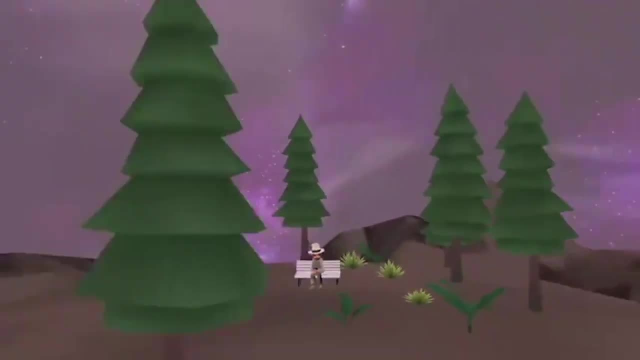 using energy, you can bump down uh different, different, different uh molecules or different particles to uh molecules, or different particles to uh molecules or different particles to different states, different states, different states, and you know uh people that do know, and you know uh people that do know, and you know uh people that do know about what's happening in europe. 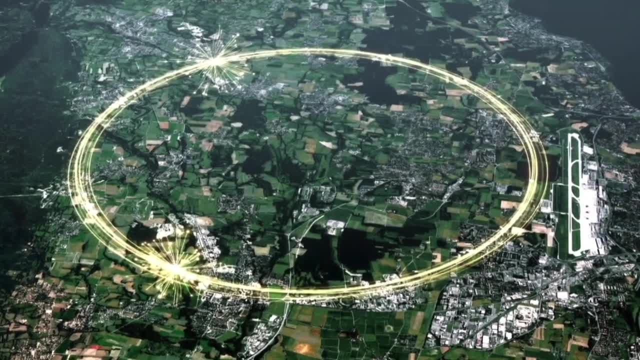 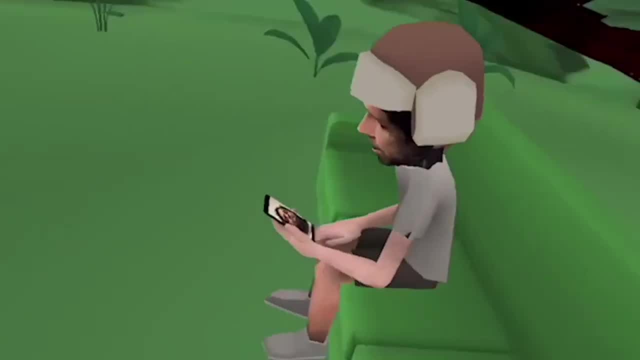 about what's happening in europe. about what's happening in europe. you know and shout out to uh more mother. you know and shout out to uh more mother. you know and shout out to uh more mother. shout out to more mother. she just won uh. shout out to more mother, she just won uh. 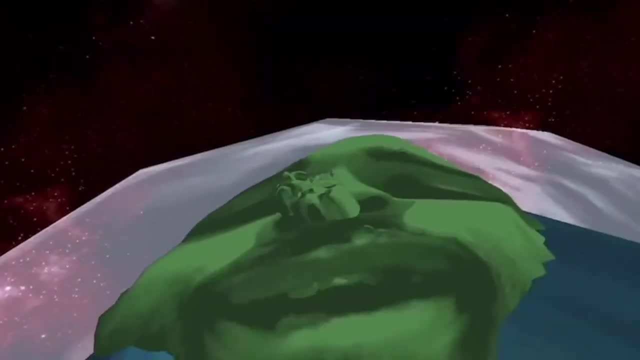 shout out to more mother. she just won, uh, the award to be able to uh do her music. the award to be able to uh do her music. the award to be able to uh do her music and do her practice at the super. and do her practice at the super. 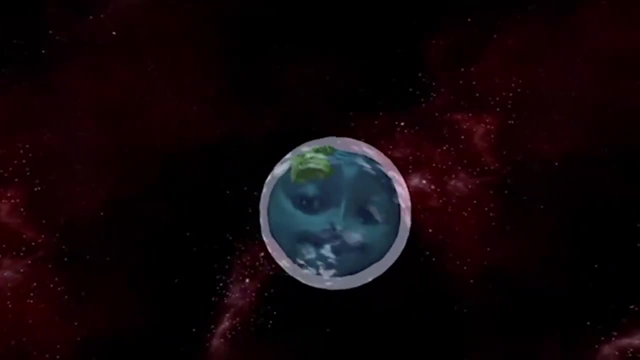 and do her practice at the super collider. but i do agree with collider. but i do agree with collider. but i do agree with brett carr that more mother needs to be brett carr, that more mother needs to be brett carr, that more mother needs to be careful. 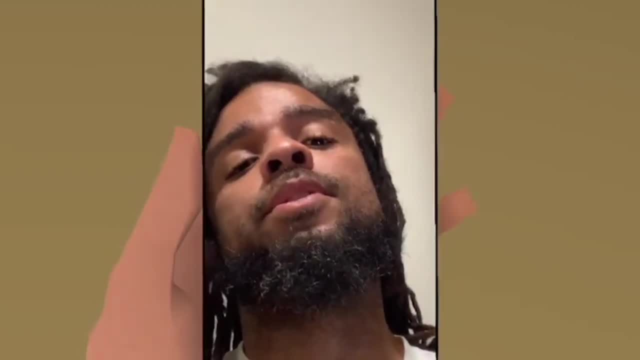 careful, careful, because they've done a bunch of rituals. because they've done a bunch of rituals, because they've done a bunch of rituals down there at the super collider stuff down there at the super collider stuff, down there at the super collider stuff- um, you can look at some of brett carr you. um, you can look at some of brett carr. you, um, you can look at some of brett carr. you know a kyle ross some of his videos and know a kyle ross some of his videos and know a kyle ross some of his videos and he's got the. 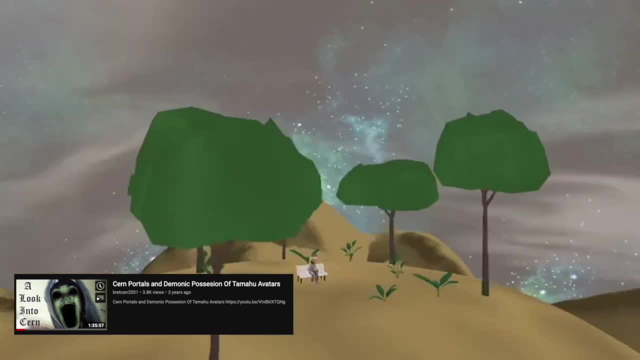 he's got the. he's got the actual ceremonies that they were actually actual ceremonies, that they were actually actual ceremonies, that they were actually doing at the uh super collider thing, but doing at the uh super collider thing, but doing at the uh super collider thing, but you, uh, you can actually look that up and 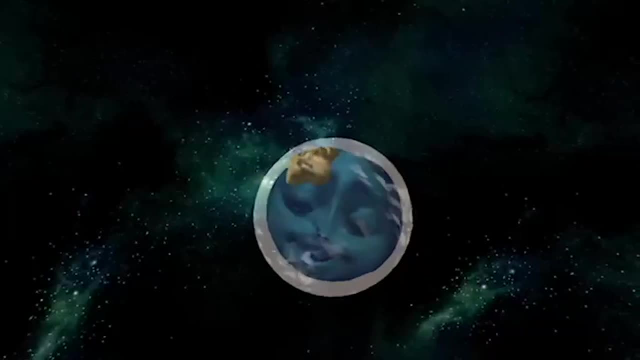 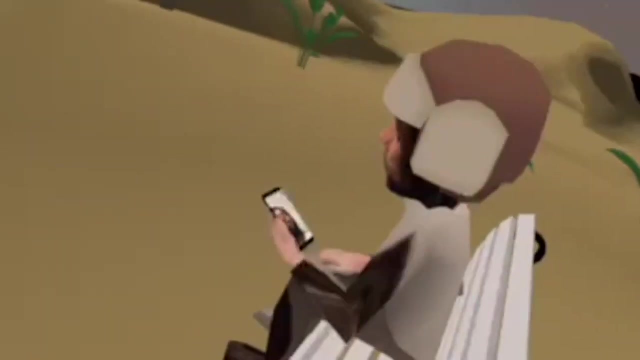 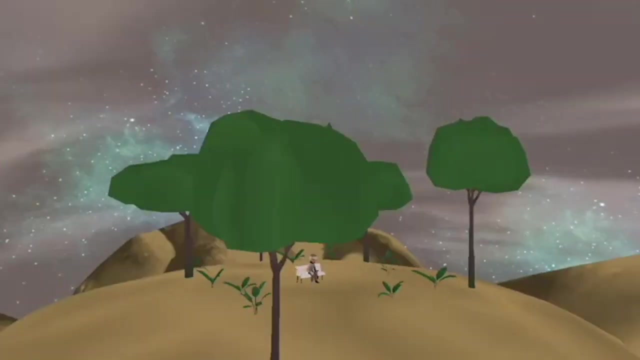 you, uh, you can actually look that up and you, uh, you can actually look that up and actually shout out, to actually shout out, to actually shout out to. you know from like a singer, because i you know from like a singer, because i you know from like a singer because i don't listen to r b, but when it's all. 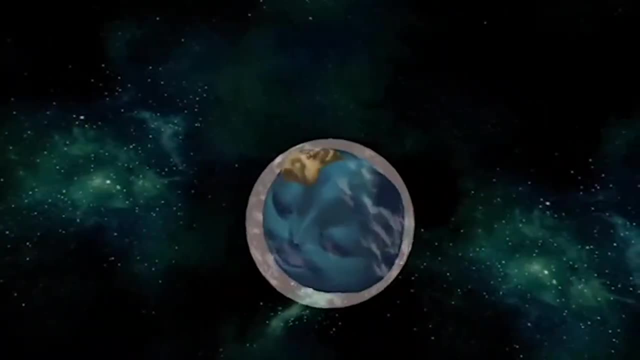 don't listen to r b, but when it's all. don't listen to r b, but when it's all, when it's glitchy beats, when it's glitchy beats, when it's glitchy beats, i like it. uh, you know. leah too, you know. 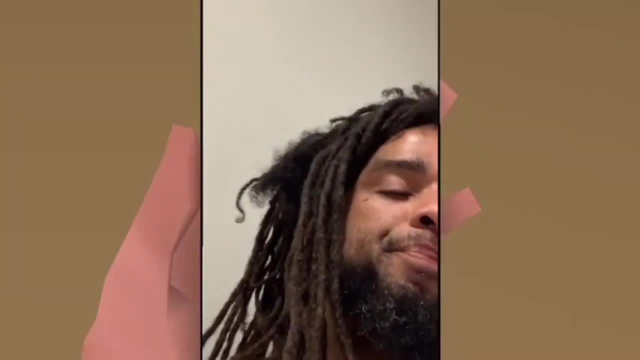 i like it. uh, you know leah too, you know i like it. uh, you know leah too. you know, like, like, like timberland beats, but uh, yeah, so timberland beats, but uh, yeah, so timberland beats, but uh, yeah, so, um, you know. so we're going to read to: um, you know, so we're going to read to. um, you know, so we're going to read to: the rest of this, the modern photon, the rest of this, the modern photon, the rest of this, the modern photon. concept originated during the first two. concept originated during the first two. 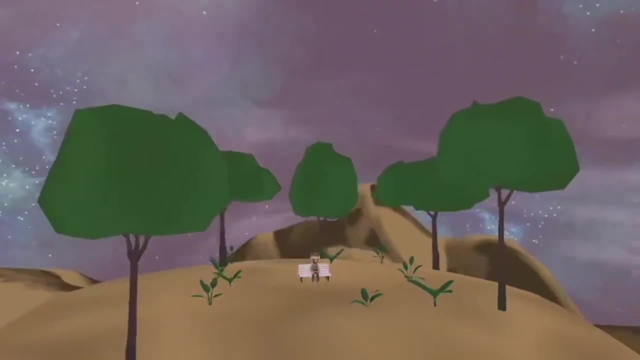 concept originated during the first two decades of the 20th century, with the decades of the 20th century, with the decades of the 20th century, with the work of albert einstein, who built work of albert einstein, who built work of albert einstein, who built upon the research of max planck. now, 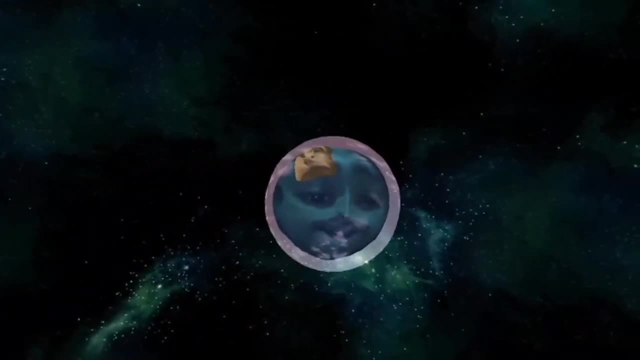 upon the research of max planck. now, upon the research of max planck. now, actually, obviously, we know, you know, actually, obviously, we know, you know, actually, obviously we know, you know we're talking about, we're talking about, we're talking about, you know, rays and and, uh, you know. 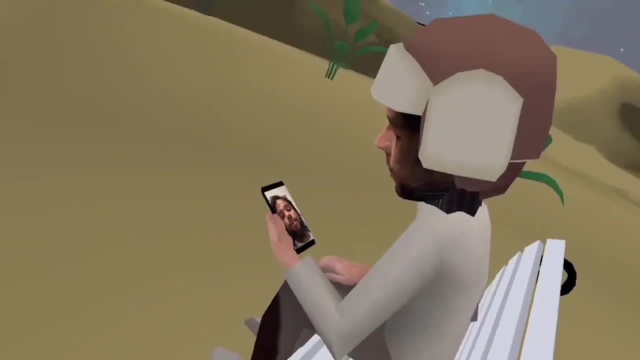 you know rays and and? uh, you know you know rays and and? uh, you know snake waves and stuff like that. these snake waves and stuff like that, these snake waves and stuff like that. these diagrams- uh, you know diagrams. uh, you know diagrams. uh, you know. all relate to or higher uh technology. 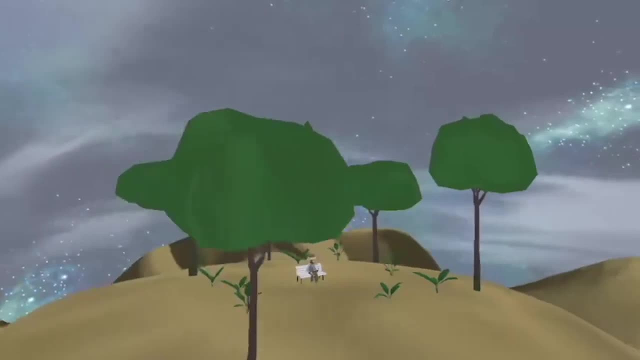 all relate to, or higher uh technology. all relate to, or higher uh technology. that was, that was, that was. you know we still can't replicate. you know we still can't replicate. you know we still can't replicate pyramids and things like that. so, pyramids and things like that, so 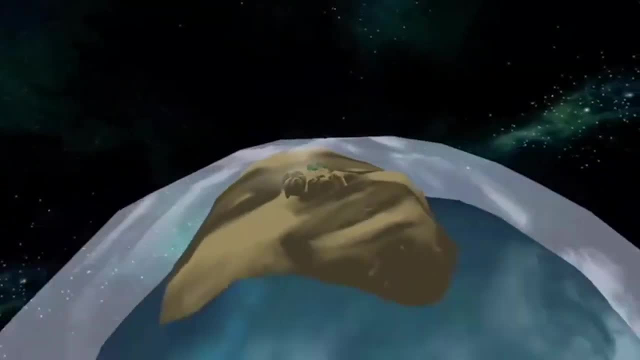 pyramids and things like that. so, uh, i'm not keeping reading to to all of uh, i'm not keeping reading to to all of uh, i'm not keeping reading to to all of those, as far as the people that those, as far as the people that 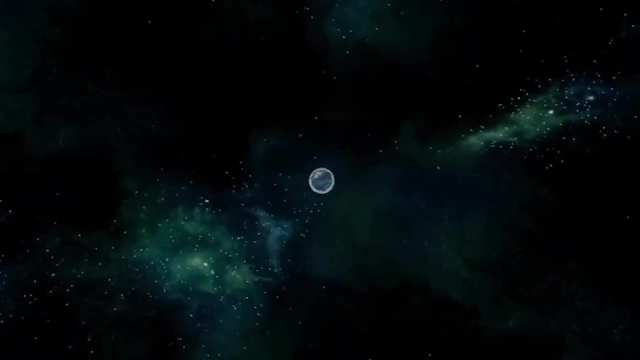 those, as far as the people that discover all these principles, because discover all these principles, because discover all these principles, because you know a lot of these things were, you know a lot of these things were, you know a lot of these things were unlocked when they raided, uh, egypt in. 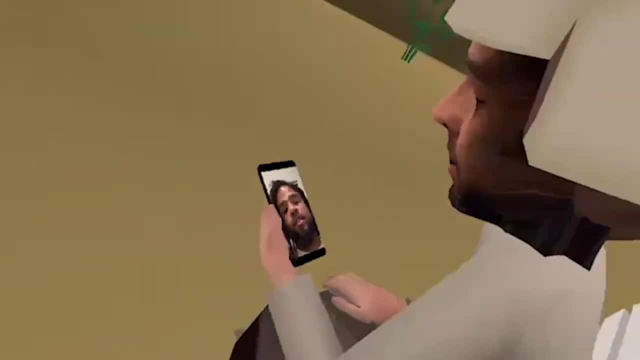 unlocked when they raided uh egypt in. unlocked when they raided uh egypt in the 1800s and stuff like that. you know the 1800s and stuff like that. you know the 1800s and stuff like that. you know they unlocked a lot of different secrets. they unlocked a lot of different secrets. they unlocked a lot of different secrets and we don't know which ones are locked and we don't know which ones are locked, and we don't know which ones are locked and which ones were invented and which ones were invented. 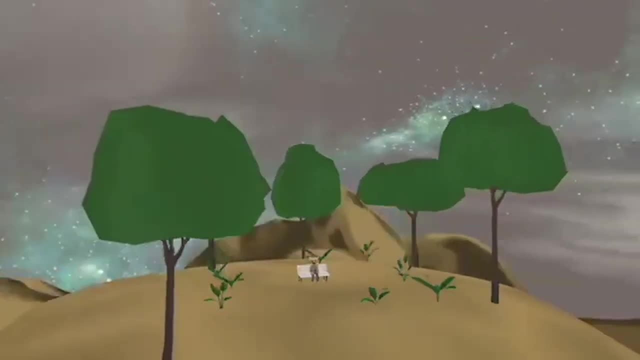 and which ones were invented. but uh, but i'll give credit where. but uh, but i'll give credit where. but uh, but i'll give credit where credit's due so far, credit's due so far. credit's due so far you know. so uh, einstein introduced the 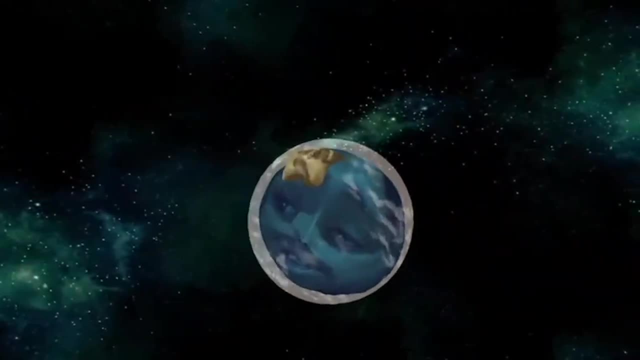 you know so, uh, einstein introduced the. you know so, uh, einstein introduced the idea that light itself is made of idea, that light itself is made of idea, that light itself is made of. discrete units of energy in 1926. discrete units of energy in 1926. 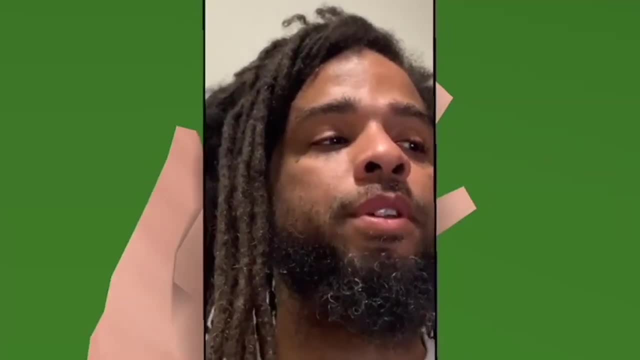 discrete units of energy. in 1926, gilbert and lewis popularized the term. gilbert and lewis popularized the term. gilbert and lewis popularized the term photon for these energy units. photon for these energy units. photon for these energy units. subsequently, many of the experiments subsequently, many of the experiments. subsequently, many of the experiments validated einstein's approach. validated einstein's approach. validated einstein's approach in the standard model particle physics. in the standard model particle physics. in the standard model particle physics. photons and other elementary particles. photons and other elementary particles. 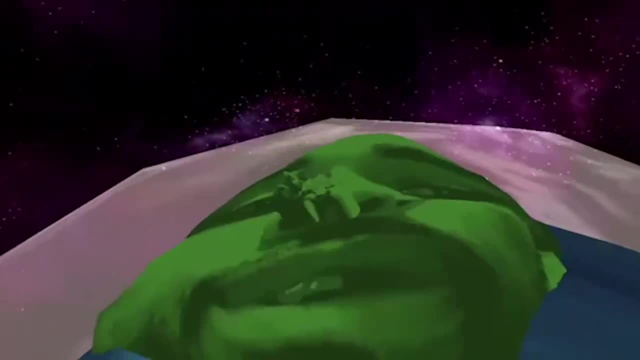 photons and other elementary particles are described as necessary consequences. are described as necessary consequences. are described as necessary consequences of physical laws having a certain of physical laws. having a certain of physical laws having a certain symmetry at every point in space time. of physical laws having a certain symmetry at every point in space time. 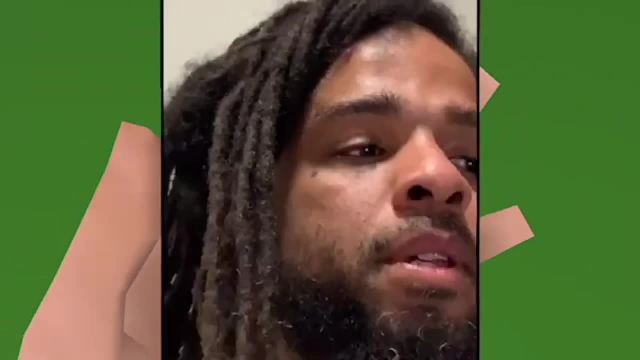 of physical laws having a certain symmetry at every point in space time. the intrinsic properties of symmetry at every point in space time. the intrinsic properties of symmetry at every point in space time. the intrinsic properties of particles such as charge mass spin. particles such as charge mass spin. 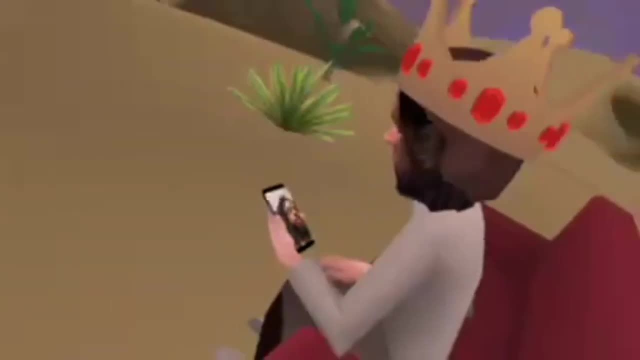 particles such as charge, mass, spin, are determined by this gauge symmetry, are determined by this gauge symmetry, are determined by this gauge symmetry. the photon concept has led to. the photon concept has led to. the photon concept has led to momentous advances in experimental, momentous advances in experimental. 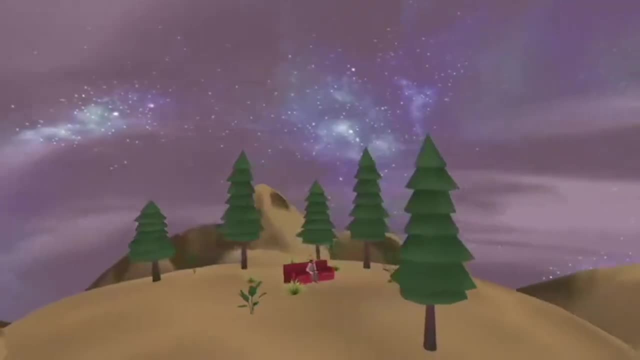 momentous advances in experimental theoretical physics, including theoretical physics, including theoretical physics, including lasers Bose-Einstein condensation. lasers Bose-Einstein condensation. lasers Bose-Einstein condensation. quantum field theory and the quantum field theory and the quantum field theory and the probabilistic interpretation of quantum. 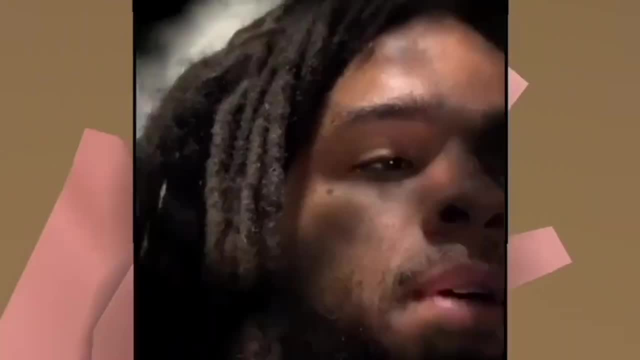 probabilistic interpretation of quantum. probabilistic interpretation of quantum mechanics. it has been applied to mechanics. it has been applied to mechanics. it has been applied to photochemistry: high resolution photochemistry, high resolution photochemistry. high resolution microscopy. see with photochemistry, microscopy, see with photochemistry, microscopy. see with photochemistry. um, you know the colors that are emanating? 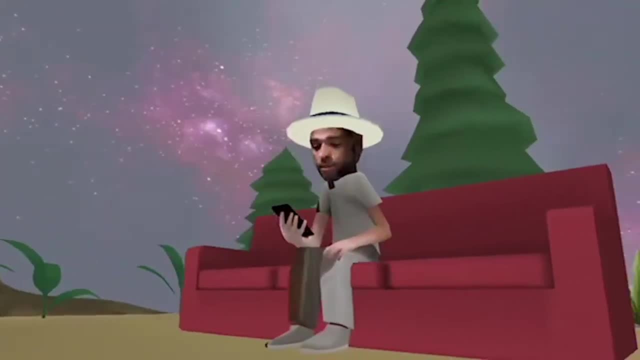 um, you know the colors that are emanating, um, you know the colors that are emanating from our body, from our body, from our body. you can see the elements. you know the. you can see the elements. you know the. you can see the elements. you know the, every element, you know every flame. if, 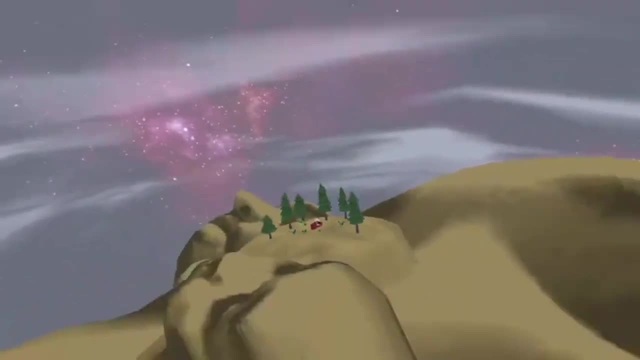 every element, you know every flame. if every element, you know every flame. if you burn um, you burn um. you burn um. you know in the periodic table of. you know in the periodic table of, you know in the periodic table of elements, if you burn each different elements, if you burn each different. 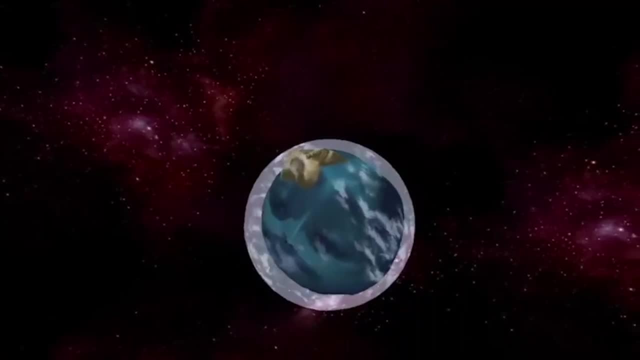 elements. if you burn each different element, every flame, every element is element, every flame, every element is element, every flame, every element is going to create a different color flame, going to create a different color flame. going to create a different color flame, like we know, if you burn copper, uh, like, 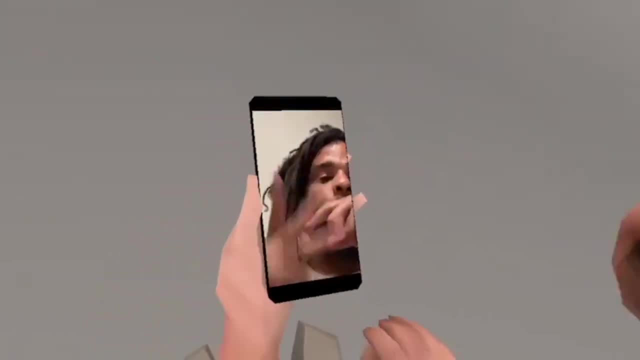 like we know if you burn copper. uh like like we know if you burn copper, uh like my wedding ring right here. this is my my wedding ring right here. this is my my wedding ring right here. this is my wedding ring. it's got copper in the wedding ring. it's got copper in the 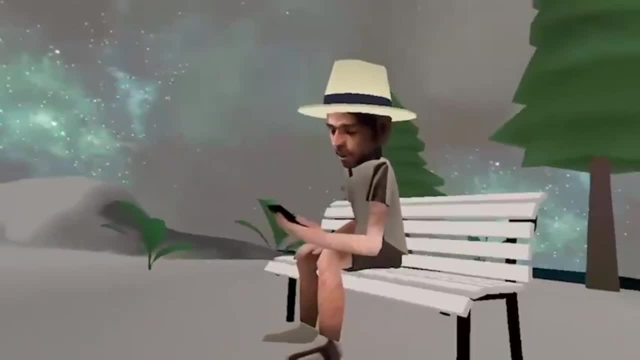 wedding ring. it's got copper in the lining. you know what i'm saying? and uh, lining, you know what i'm saying. and uh lining, you know what i'm saying. and uh, if you burn copper, it's going to create. if you burn copper, it's going to create. 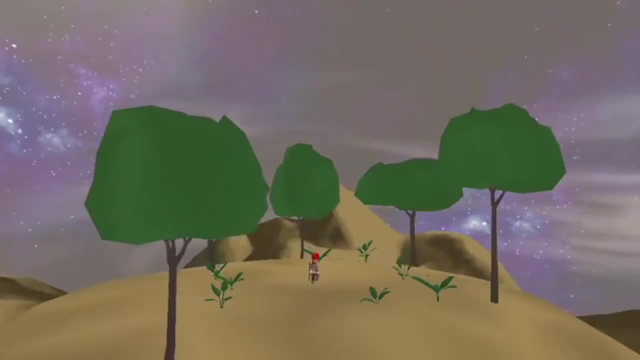 if you burn copper, it's going to create a green flame. a green flame, a green flame. let's see if i can change the hat. oh, let's see if i can change the hat. oh, let's see if i can change the hat. oh, there we go. 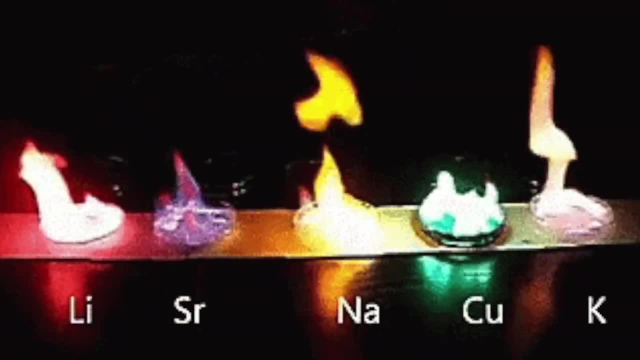 there we go, there we go: um, it's going to create a green flame, um, it's going to create a green flame, um, it's going to create a green flame. and uh, you know every other element, so, and uh, you know every other element, so, and uh, you know every other element, so i'll show the flames too. that of the i'll show the flames, too, that of the. i'll show the flames, too, that of the elements. you know what i'm saying? look elements. you know what i'm saying? look elements. you know what i'm saying. look all that stuff up. that's, that's real. 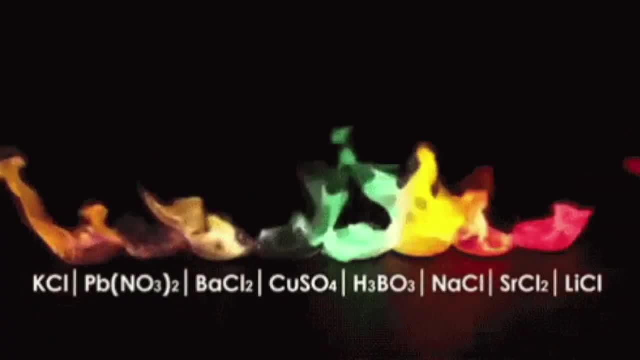 all that stuff up? that's that's real. all that stuff up? that's that's real. they never taught me that in school. they they never taught me that in school. they they never taught me that in school. they never taught me that in school. they never taught me that every single element has. 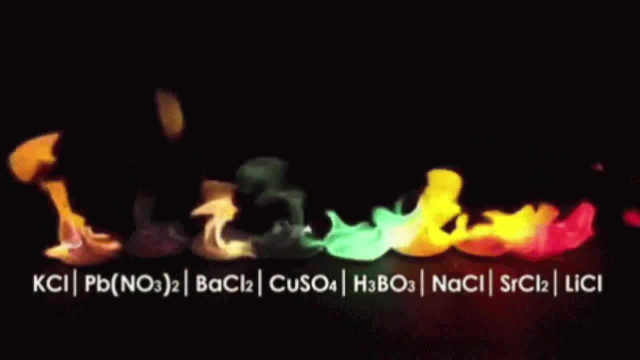 never taught me that every single element, has never taught me that every single element has a different color like: why don't they a different color like why don't they a different color like: why don't they have that chart in school? have that chart in school, have that chart in school, you know. so i'm going to be compiling a 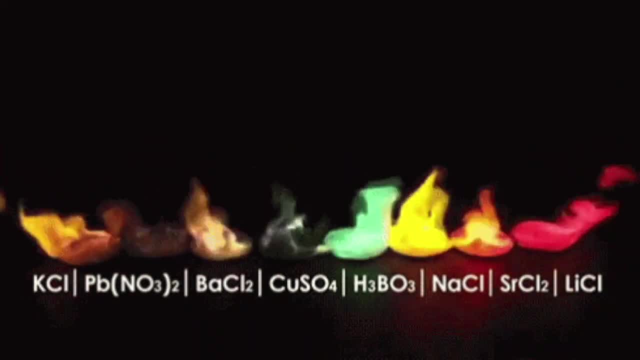 you know, so i'm going to be compiling a. you know, so i'm going to be compiling a bunch of things for uh. bunch of things for uh. bunch of things for uh. my own pedagogies for, for uh um. my own pedagogies for for uh um. 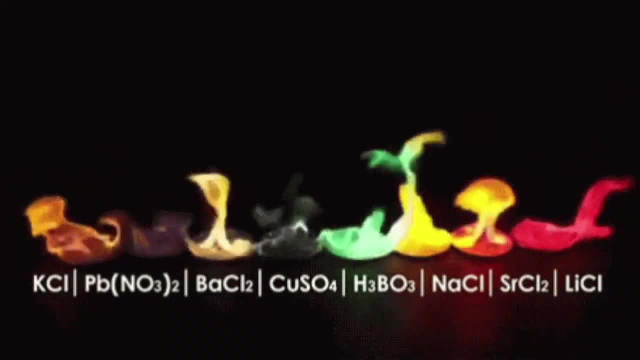 my own pedagogies for for uh, um, you know teaching. uh, you know teaching. uh, you know teaching. uh, all ages and all levels of students. you all ages and all levels of students. you all ages and all levels of students. you know, because we've come out of the dark. 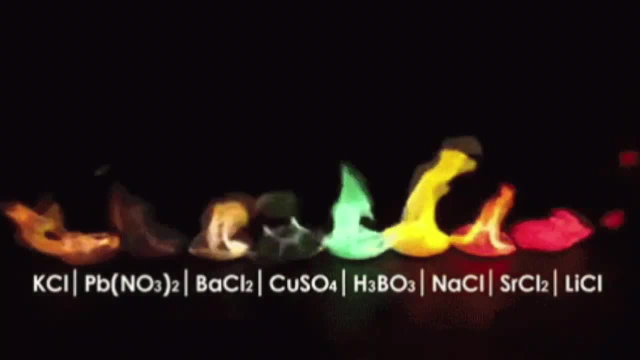 know, because we've come out of the dark. know, because we've come out of the dark ages, we're still coming out of dark ages, ages we're still coming out of dark ages, ages we're still coming out of dark ages and, i think, a lot of the things that um 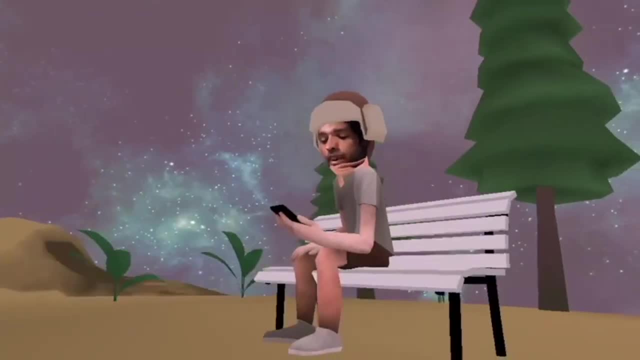 and i think a lot of the things that, um, and i think a lot of the things that um, that the dark ages are a part of. is is that the dark ages are a part of. is is that the dark ages are a part of. is is fracturing information and scattering it. 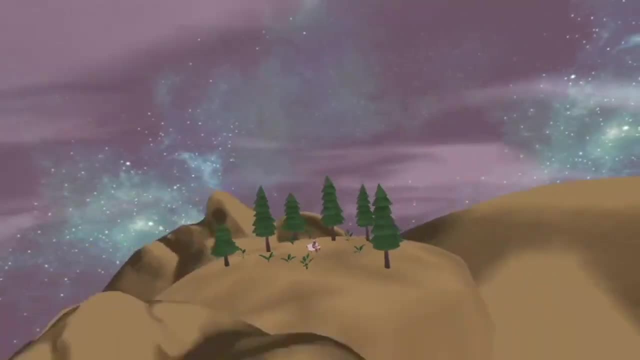 fracturing information and scattering it. fracturing information and scattering it around. not putting it in one place around. not putting it in one place around. not putting it in one place so that people can capitalize off of it, so that people can capitalize off of it, so that people can capitalize off of it and get you a bunch of student loan. 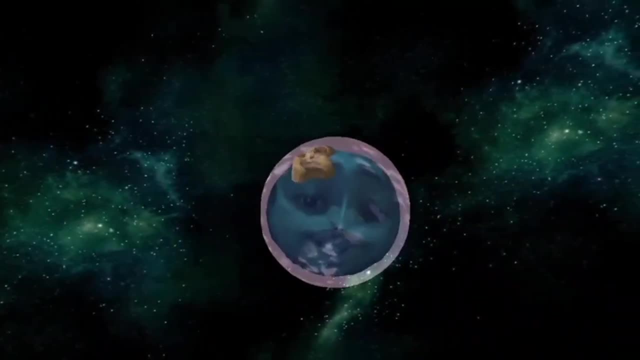 and get you a bunch of student loan and get you a bunch of student loan debt. you know what i'm saying? debt? you know what i'm saying debt? you know what i'm saying? student loan debt to me is like slavery. student loan debt to me is like slavery. 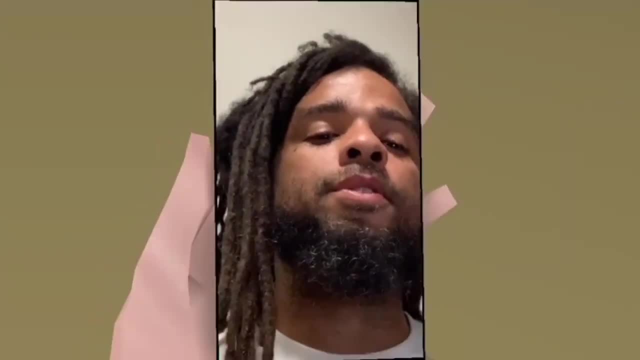 student loan debt to me is like slavery in the feet in the future, in the feet in the future, in the feet in the future. there's not going to be student loan, there's not going to be student loan, there's not going to be student loan debt. you know it's like. why are you? 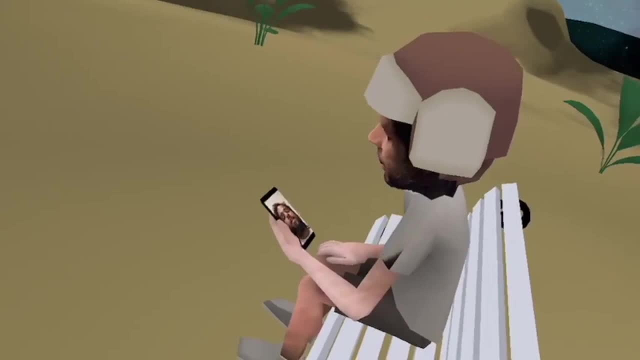 debt. you know it's like: why are you debt? you know it's like: why are you charging people for education? hoarding charging people for education? hoarding charging people for education, hoarding information, information, information. you know what i'm saying, you know. you know what i'm saying, you know. 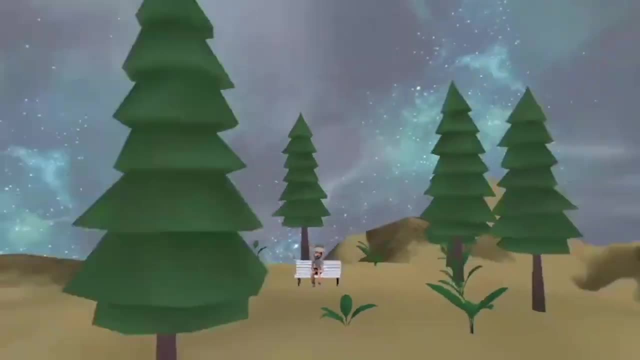 you know what i'm saying, you know obviously you know that people should. obviously you know that people should. obviously you know that people should have private information, have private information, have private information private. but uh, you know um like what private. but uh, you know um like what. 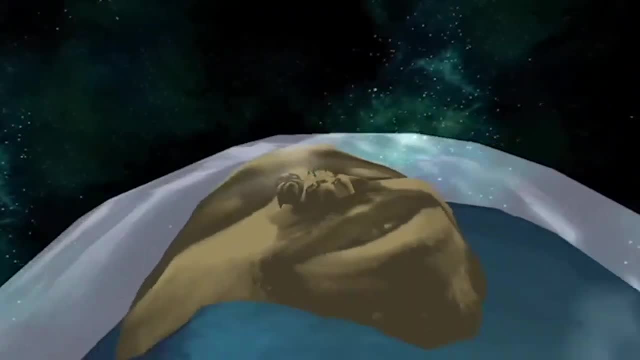 private. but uh, you know, um, like what they did at the beach that summer. they did at the beach that summer. they did at the beach that summer. you know that could be private information. you know that could be private information. you know that could be private information- their pictures. 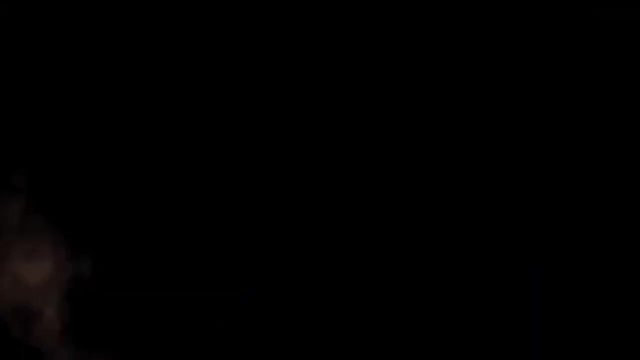 their pictures, their pictures. but if it's like you know calculus, and. but if it's like you know calculus and. but if it's like you know calculus and physics, you know physics, you know physics, you know. why is it costing money from all you? why is it costing money from all you? 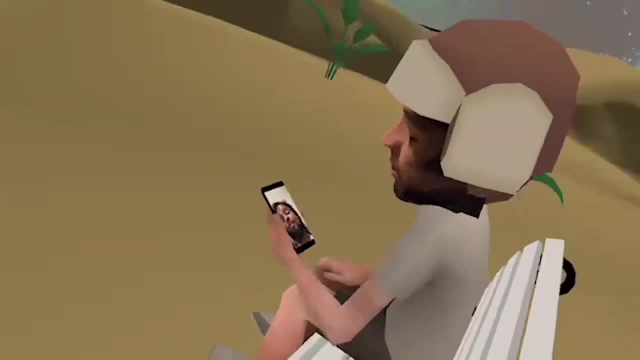 why is it costing money from all you know. why is it only making? know, why is it only making? know, why is it costing money from all you know. why is it only making? uh, you know the top cast, you know. uh, you know the top cast, you know. 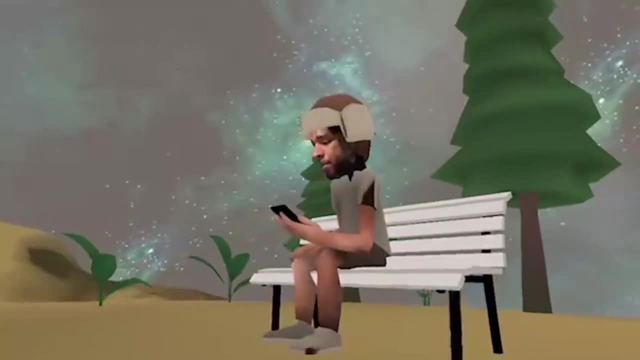 uh, you know the top cast, you know all the money, you know all the money, you know all the money, you know so, um, you know, back to uh. so, um, you know back to uh. so, um, you know, back to uh, feynman, you know the way this relates to. 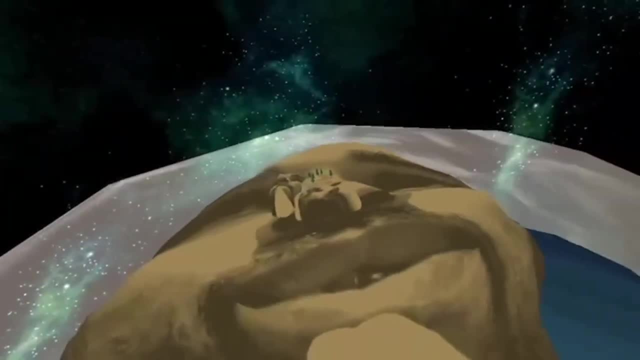 feynman. you know the way this relates to feynman. you know the way this relates to the new life, um the new life, um the new life, um stuff. is that you know new life was stuff? is that you know new life was stuff? is that you know new life was talking about? um the fifth dimension, but 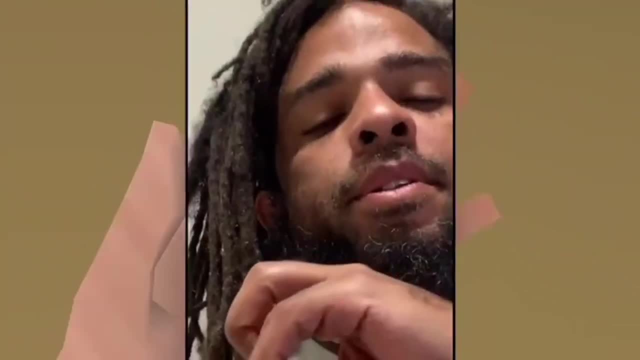 talking about um the fifth dimension, but talking about um the fifth dimension, but he wasn't giving. he wasn't giving, he wasn't giving any idea about what the fifth dimension, any idea about what the fifth dimension is. we cannot perceive dimensions. is we cannot perceive dimensions? is we cannot perceive dimensions that are higher than the fourth dimension? 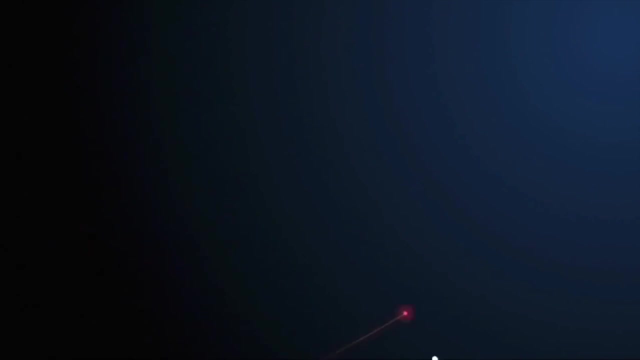 that are higher than the fourth dimension, that are higher than the fourth dimension because they exist on a subatomic level, because they exist on a subatomic level, because they exist on a subatomic level, these higher dimensions actually deal. these higher dimensions actually deal. these higher dimensions actually deal with the possibilities if a person were 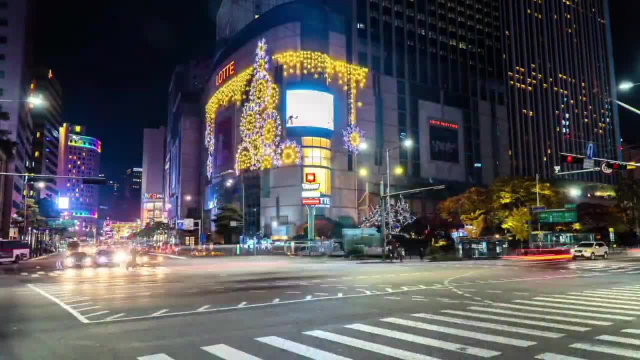 with the possibilities. if a person were with the possibilities, if a person were living in a world of five dimensions, living in a world of five dimensions, living in a world of five dimensions, then he would be able to play with time. then he would be able to play with time. 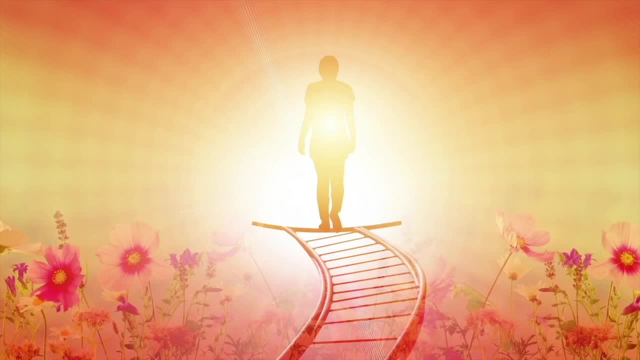 then he would be able to play with time in different ways, in different ways. in different ways. he could move either in past or in. he could move either in past or in. he could move either in past or in future. it would also be possible for him. future: it would also be possible for him. 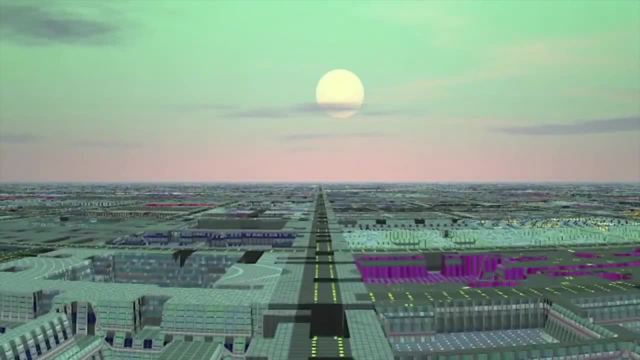 future, it would also be possible for him to be present at different locations, at to be present at different locations, at to be present at different locations at the same time. when we see a rope from the same time when we see a rope from the same time. when we see a rope from large distance, we only observe its one. 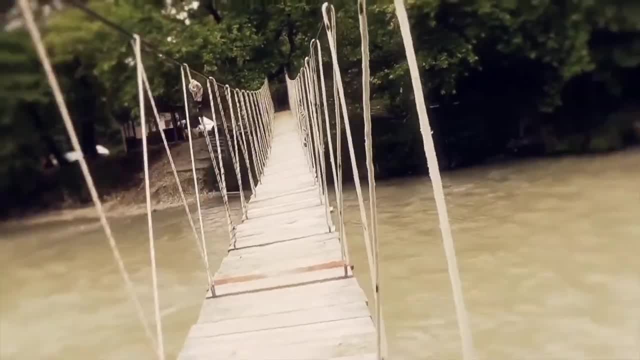 large distance. we only observe its one large distance. we only observe its one dimension, that is the length. but any dimension, that is the length, but any dimension, that is the length. but any insect moving on that rope will also see. insect moving on that rope will also see. 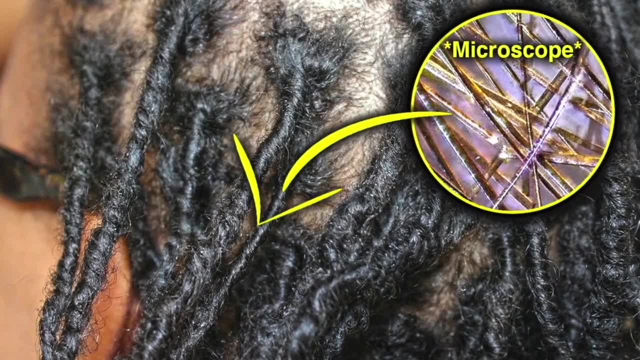 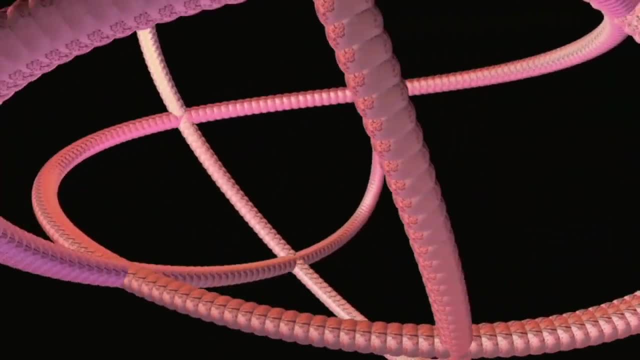 insect moving on that rope will also see other dimensions of the rope, other dimensions of the rope, other dimensions of the rope, like its thickness. it will also observe. like its thickness. it will also observe like its thickness. it will also observe the fine grooves and roughness. and 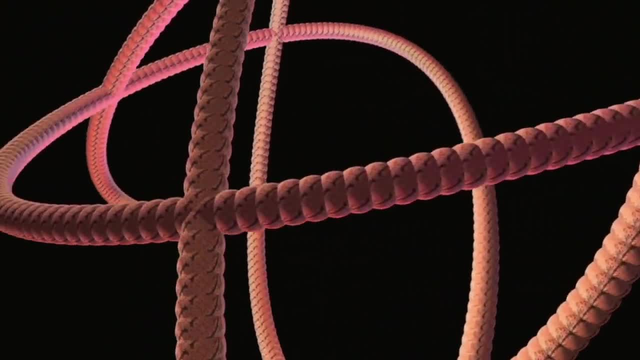 the fine grooves and roughness and the fine grooves and roughness and circumference of the rope, that could not circumference of the rope, that could not circumference of the rope, that could not be seen by a distant observer, you know, be seen by a distant observer, you know. 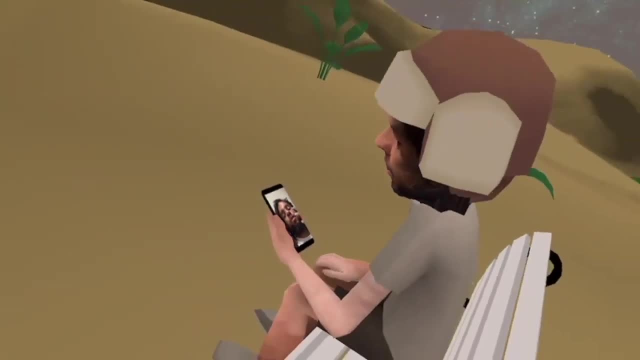 be seen by a distant observer. you know what i'm saying, what i'm saying, what i'm saying, and that's why i'm bringing up these, and that's why i'm bringing up these, and that's why i'm bringing up these fame and charts. and you know, because of fame and charts, and you know because of fame and charts, and you know because of. you know, as, as we've said before you, you know, as as we've said before you, you know, as, as we've said before, you could look at the, could look at the. 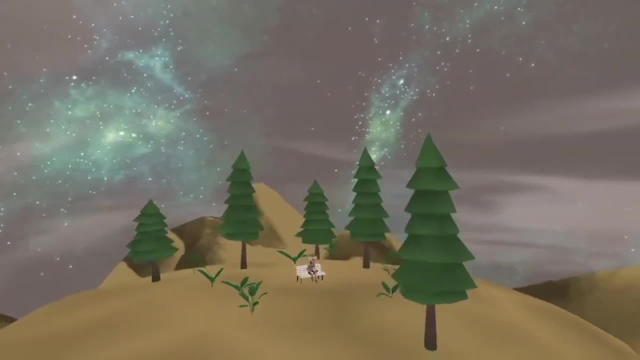 could look at the lecture with uh assir. we spoke about uh lecture with uh assir. we spoke about uh lecture with uh assir. we spoke about uh assir, the duke of tears. we were speaking assir the duke of tears. we were speaking. assir the duke of tears. we were speaking about um. 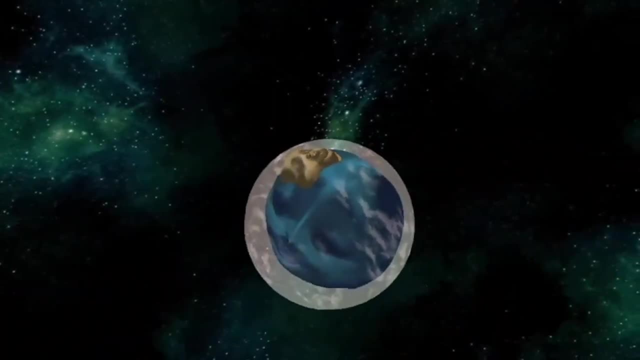 about um, about um. uh, you know dimensionality as well. uh, you know dimensionality as well. uh, you know dimensionality as well. towards the end of the lecture and you towards the end of the lecture, and you towards the end of the lecture. and you know, you can look at it as a box within. 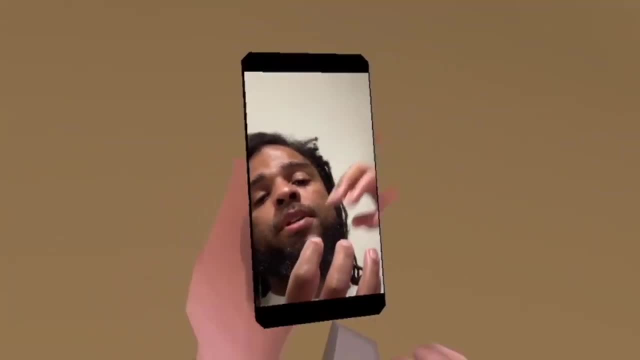 know you can look at it as a box within. know you can look at it as a box within a box within a box within a box, a box within a box within a box, a box within a box within a box, kind of like the russian uh those. kind of like the russian, uh, those kind of like the russian, uh, those russian toys. you know what i'm saying, russian toys. you know what i'm saying, russian toys, you know what i'm saying? where it's a little person inside of a. where it's a little person inside of a. 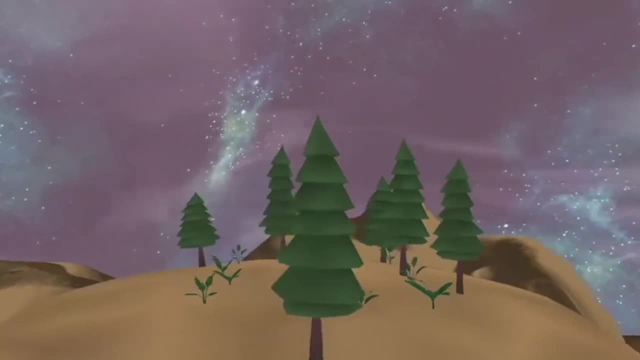 where it's a little person inside of a little person inside of a little person, little person inside of a little person, little person inside of a little person, and so you can think of multiverses in, and so you can think of multiverses in, and so you can think of multiverses in that way. you know, people have depicted. 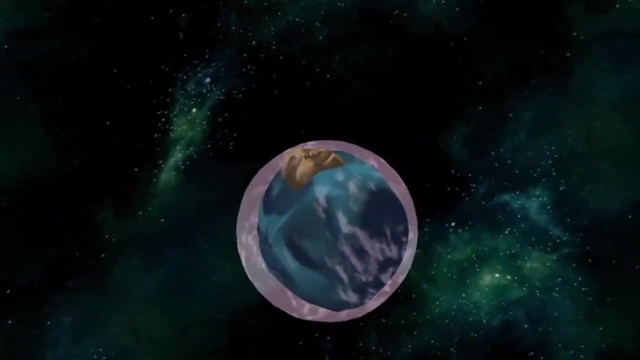 that way, you know, people have depicted, that way, you know, people have depicted multiverses, multiverses, multiverses. in a lot of different ways, um, and you in a lot of different ways, um, and you in a lot of different ways, um, and you know. so multiverses can be. 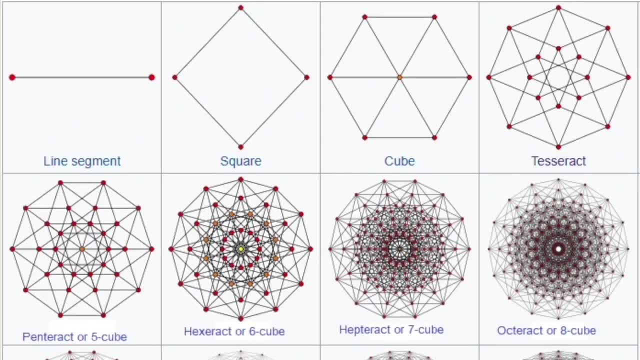 know so multiverses can be. know so multiverses can be a box within a box, right, because some of a box within a box. right, because some of the higher dimensions are actually the higher dimensions are actually the higher dimensions, are actually smaller dimensions, smaller dimensions. 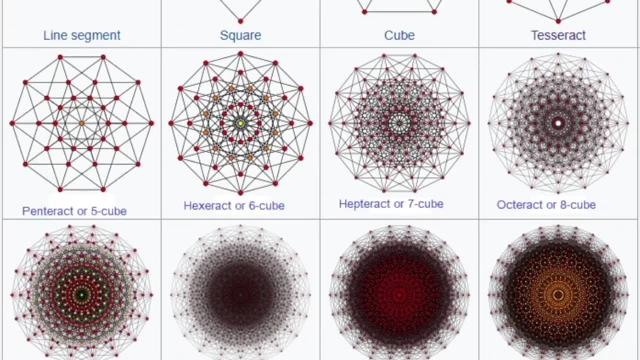 smaller dimensions. you know um, even though it's outside of you know um, even though it's outside of you know um, even though it's outside of our dimension. you know you can look at our dimension. you know you can look at our dimension. you know you can look at there's smaller dimensions and there's 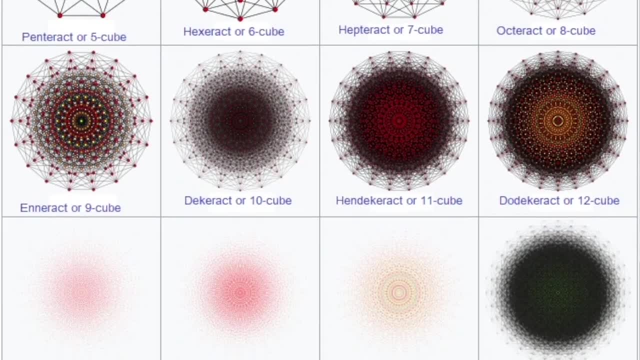 there's smaller dimensions and there's there's smaller dimensions and there's bigger dimensions, like what's happening, bigger dimensions like what's happening, bigger dimensions like what's happening in this animation where you're zooming, in this animation where you're zooming, in this animation where you're zooming out and somebody's able to look at. 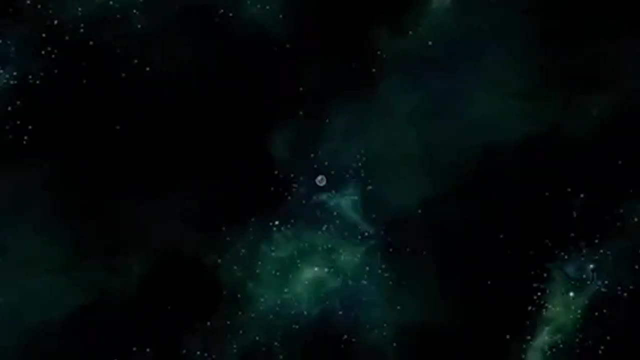 out and somebody's able to look at out, and somebody's able to look at something as like an object. you know what? something as like an object. you know what? something as like an object. you know what i'm saying and and that's what goes. i'm saying and, and that's what goes. 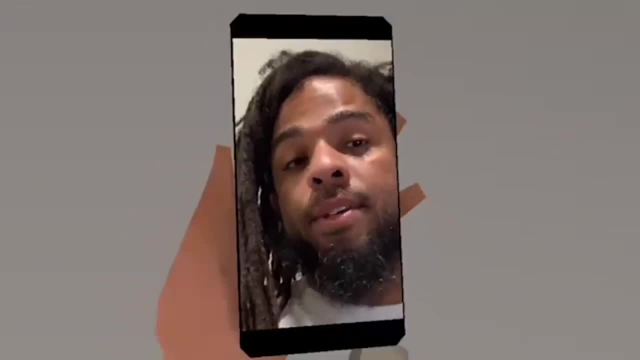 i'm saying and- and that's what goes back to uh, back to uh, back to uh- you know being on the event horizon, you, you know being on the event horizon, you, you know being on the event horizon. you know because, uh know, because uh know, because uh definitely check out the movie event. 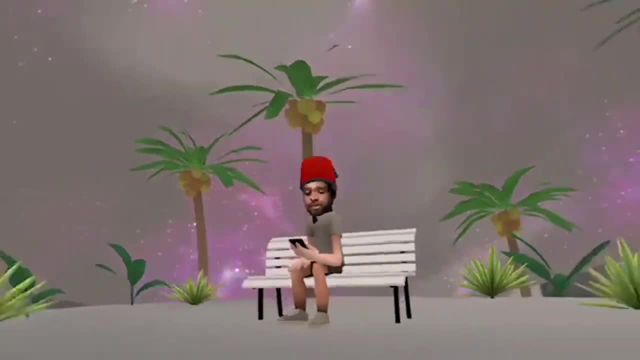 definitely check out the movie event. definitely check out the movie event. horizon, horizon, horizon, uh, because you know event in an event. uh, because you know event in an event. uh, because you know event in an event. horizon, they get near it and horizon, they get near it. and. 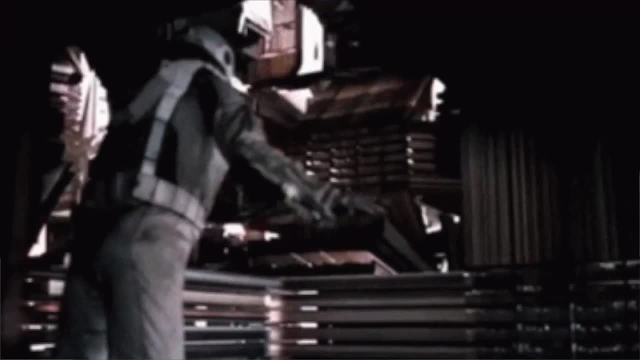 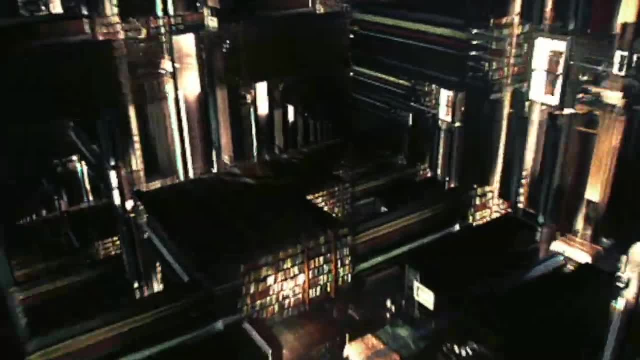 interstellar uh. definitely check out interstellar uh. they deal with kind of interstellar uh. they deal with kind of interstellar uh. they deal with kind of like: what a fifth dimensional uh like, what a fifth dimensional uh like what a fifth dimensional uh, civilization is. you know. 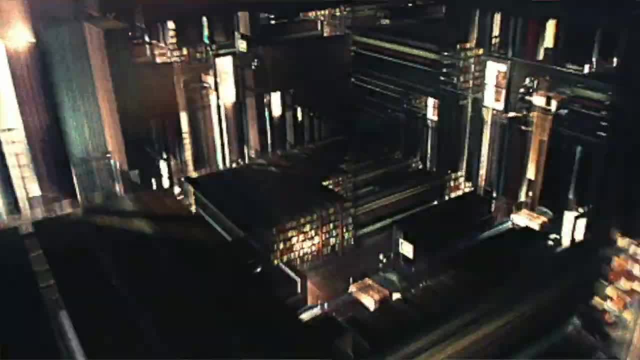 civilization is, you know civilization is, you know, a fifth dimensional civilization being a fifth dimensional civilization being a fifth dimensional civilization being one that can, uh, you know. uh looks at one that can, uh, you know. uh looks at one that can, uh, you know. uh looks at the the uh history as a. 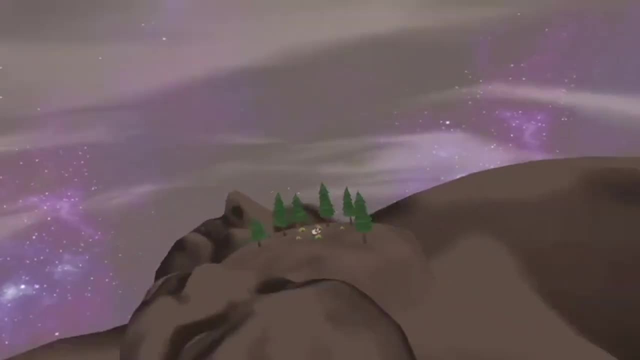 the, the uh history as a, the, the uh history as a, as an object, and they can change history as an object and they can change history as an object and they can change history, but they have their own history because, but they have their own history because, but they have their own history because their history is in their own. fifth, 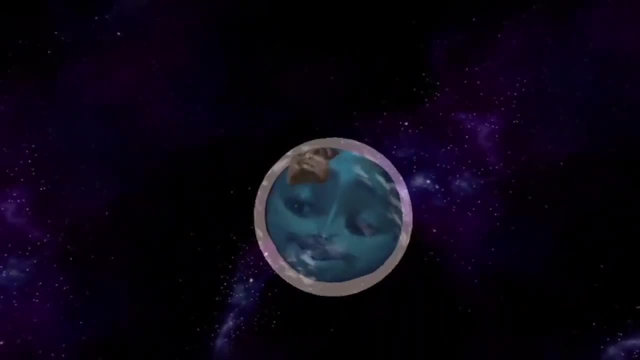 their history is in their own fifth, their history is in their own fifth dimension, and it's just relative, you dimension, and it's just relative, you dimension, and it's just relative. you know because, know, because know, because the people that are higher up in the, the people that are higher up in the, 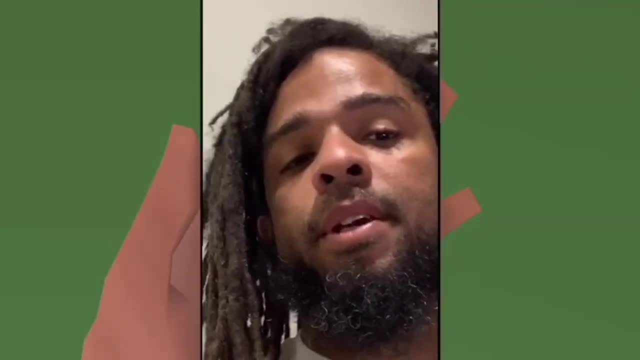 the people that are higher up in the sixth dimension above them, sixth dimension above them, sixth dimension above them. look at their dimension as an object. you look at their dimension as an object. you look at their dimension as an object. you know what i'm saying, so know what i'm saying so. 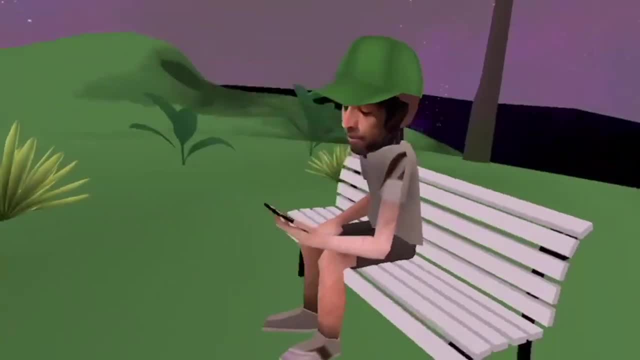 know what i'm saying, so you know a lot of people say uh. when you know a lot of people say uh. when you know a lot of people say uh when people pass away. they see their whole people pass away. they see their whole people pass away. they see their whole life flash before them. but who? life flash before them. but who? life flash before them, but who? who's to say that they're not just going? who's to say that they're not just going? who's to say that they're not just going to the fifth dimension and seeing the? to the fifth dimension and seeing the? 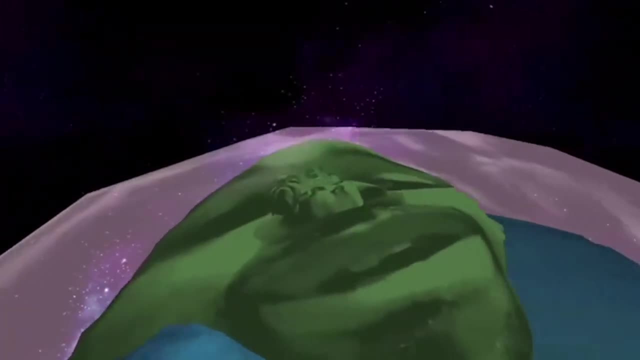 to the fifth dimension and seeing the fourth dimension as an object. so fourth dimension as an object, so fourth dimension as an object. so they're just looking at their whole life. they're just looking at their whole life. they're just looking at their whole life as like we look at an apple or an orange. as like we look at an apple or an orange, as like we look at an apple or an orange and you're moving it around, looking at and you're moving it around looking at and you're moving it around looking at the different ridges, the different ridges. 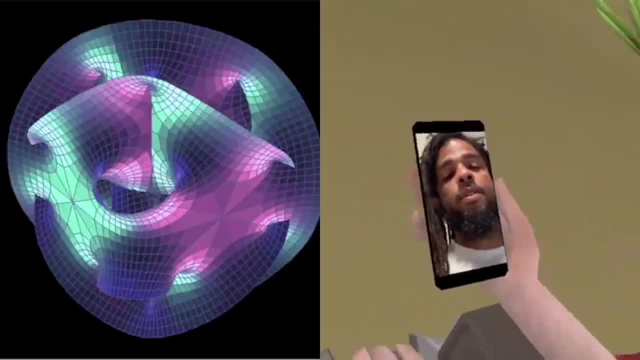 the different ridges or the different parts of it. it's just, or the different parts of it. it's just, or the different parts of it. it's just. like you know. moving your life around like you know. moving your life around like you know. moving your life around and seeing you know the diff. 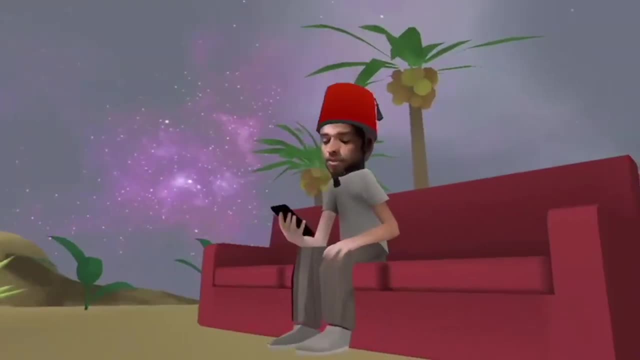 and seeing you know the diff and seeing you know the diff, all the different uh things that happen, all the different uh things that happen, all the different uh things that happen. right, because if you look back on a right, because if you look back on a right, because if you look back on a fourth dimensional trail, everything 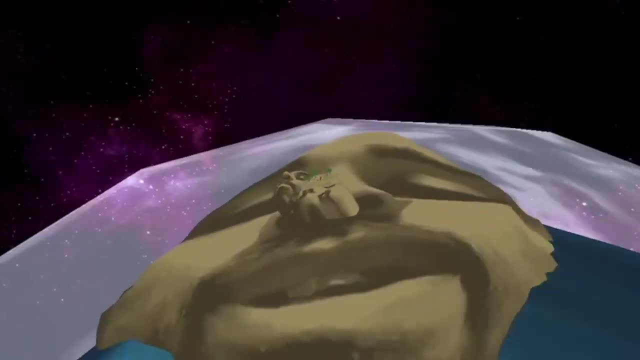 fourth dimensional trail, everything. fourth dimensional trail, everything you're gonna see, uh, you're gonna see, uh, you're gonna see, uh, you know all the trails like you move. you know all the trails like you move. you know all the trails like you move from one city to another city. you know. 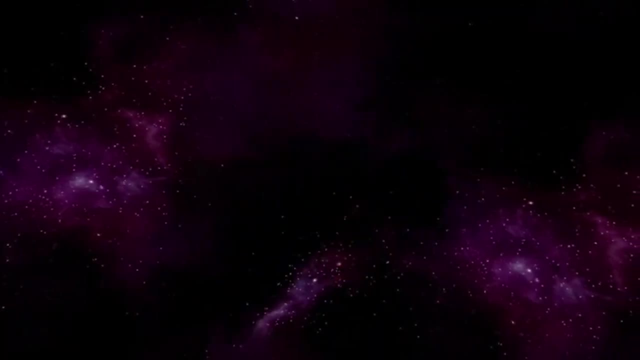 from one city to another city. you know, from one city to another city. you know um uh. shout out to tahir hempful. um uh. shout out to tahir hempful. um uh, shout out to tahir hempful, like i've seen before in his uh uh. 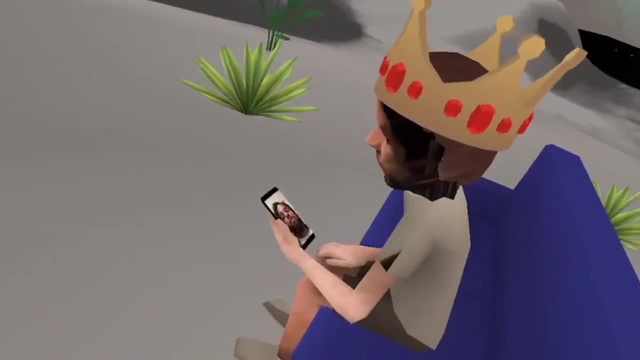 like i've seen before in his uh uh, like i've seen before in his uh uh. hip-hop uh database. uh project. hip-hop uh database, uh project. hip-hop uh database, uh project. um where uh he's you know breaking down, um where uh he's you know breaking down. 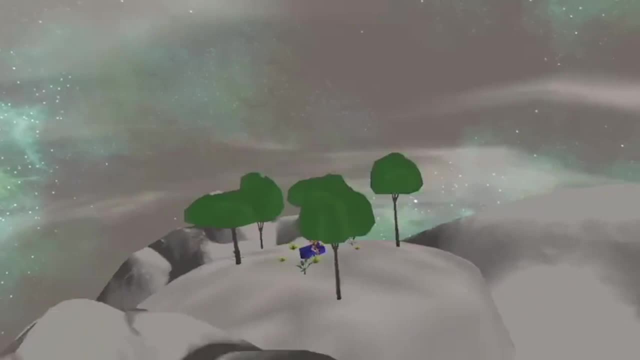 um, where uh he's, you know breaking down uh the, uh the, uh the the rap lyric databases and uh actually the rap lyric databases and uh actually the rap lyric databases and uh actually he was tracking uh kanye's movements. he was tracking uh kanye's movements. 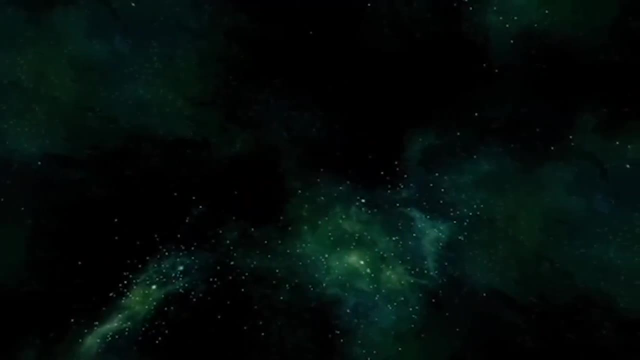 he was tracking uh kanye's movements through his fourth dimensional trail, through his fourth dimensional trail, through his fourth dimensional trail. he was actually uh, you know, because he was actually uh, you know, because he was actually uh, you know, because google trails, that's basically like your. 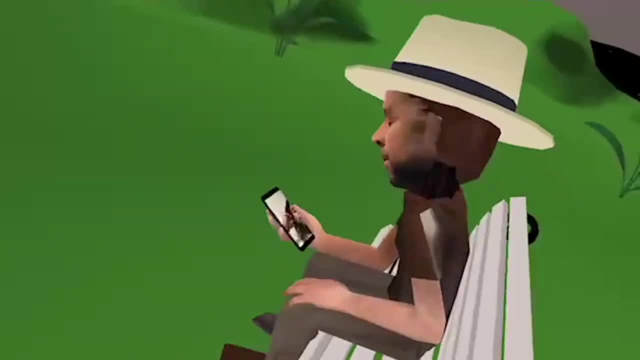 google trails. that's basically like your google trails, that's basically like your fourth dimensional movement, fourth dimensional movement, fourth dimensional movement. so, if you, you know, think about that like so. if you, you know, think about that like so. if you, you know, think about that like you're moving over time. your ancestors. 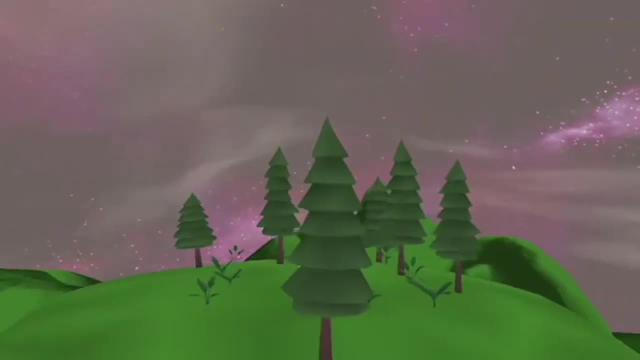 you're moving over time, your ancestors, you're moving over time, your ancestors moving over time, moving over time, moving over time, that's a trail. so a fifth dimensional that's a trail. so a fifth dimensional that's a trail. so a fifth dimensional view is going to be more of a view. 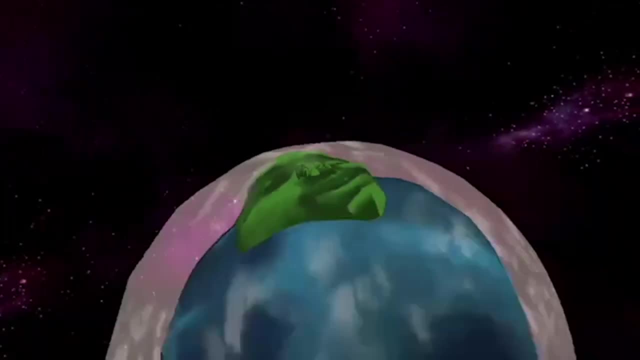 view is going to be more of a view. view is going to be more of a view. that's looking at that? um, all those that's looking at that? um, all those that's looking at that, um, all those trails, trails, trails, like a map, and that's what the famine 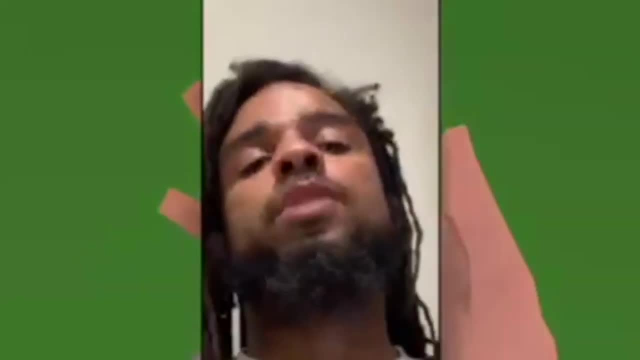 like a map and that's what the famine like a map and that's what the famine diagrams are. the famine diagrams are diagrams. are the famine diagrams are diagrams? are the famine diagrams are looking at all these particle? looking at all these particle? looking at all these particle interactions as a map?